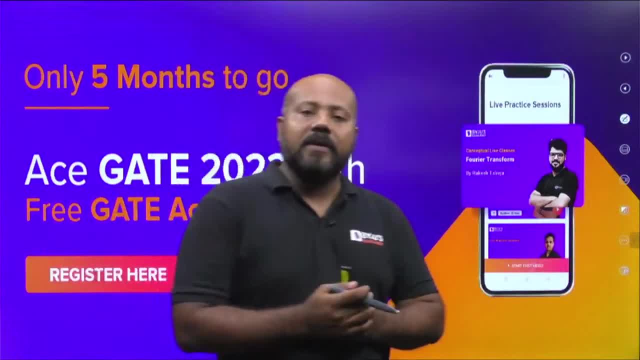 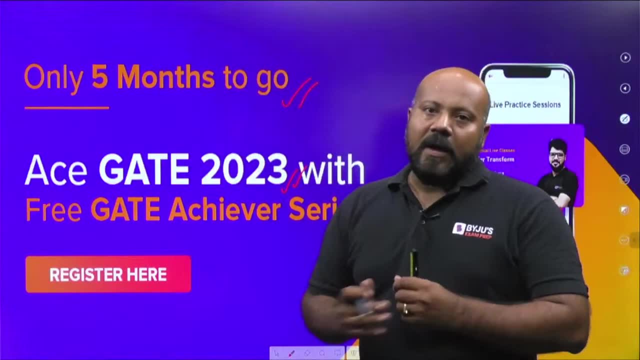 expertise. Before we start the session, a very important notification for all of you, All the candidates who are seriously preparing for GATE 2023, only five months are left In this time. if you want to accelerate your preparation, you need to prepare for GATE 2023. So, if you are, 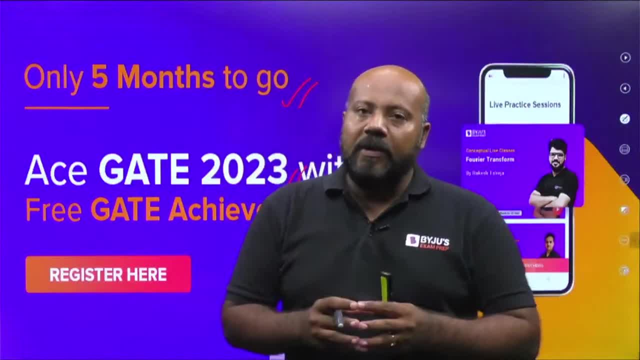 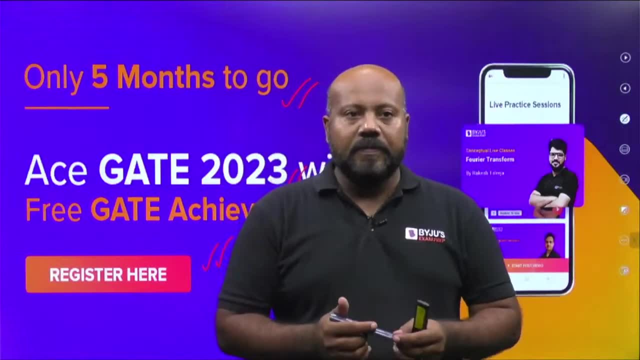 interested in preparing for GATE 2023, then you can join GATE Achiever Series, which is available on Byju's Exam Prep app. But to attend those sessions you have to get yourself registered. Good evening, Morley. How are you? 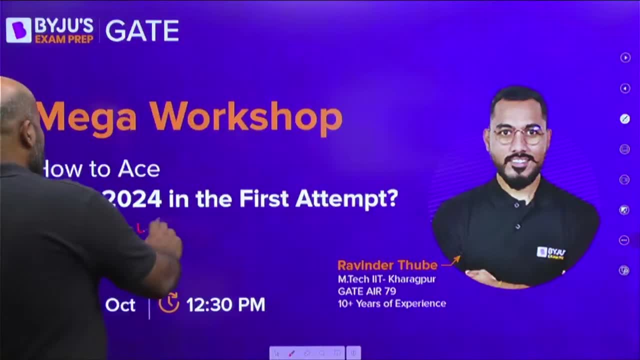 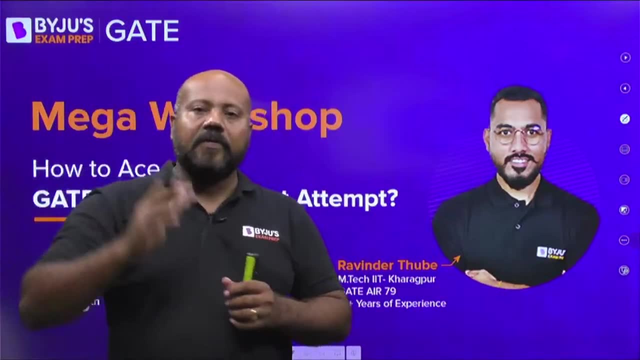 Now we have another important workshop: how to ace GATE 2024 in the first attempt. So all the candidates who are aiming GATE 2024, this workshop is going to be very important And one of your favorites is GATE 2024.. So if you are interested in GATE 2024, you can join GATE Achiever Series. which is available on Byju's Exam Prep app, And then, if you want to start preparing for GATE 2024,, you can join GATE 2022,, which is available on Byju's Exam Prep app, And then, if you want to start, preparing for GATE 2023, you can join GATE 2022.. So if you are interested in GATE 2025, you can join GATE 2023, you can join GATE 2025.. So if you are interested in GATE 2023, you can join GATE 2022. 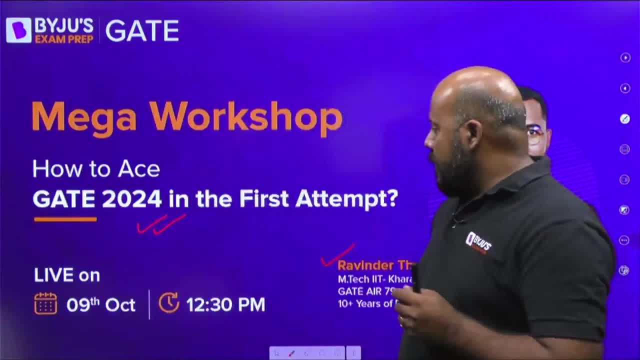 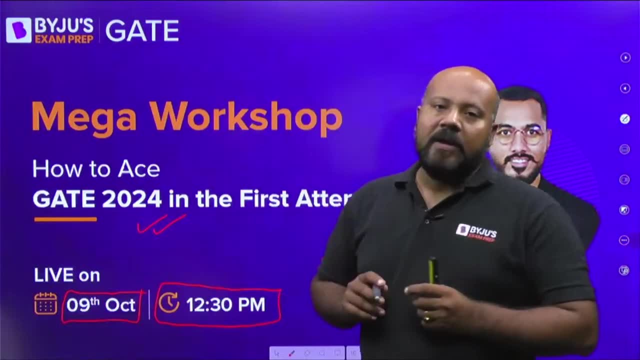 My favorite, Ravindra Sir, is going to conduct this workshop. Please note down the timings: It is going to be conducted on the ninth of October and the timing is going to be 1230pm. So do not forget to get yourself registered for this workshop, because all those candidates who are serious 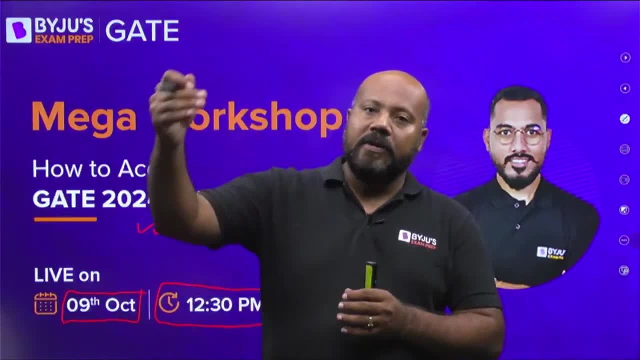 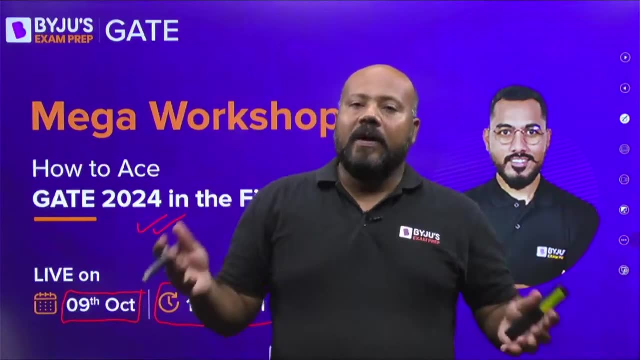 about GATE 2024,. GATE 2024 means 2023 is next year and next to next year. So, if you are in second year, if you are in third year and even if you are in final year and if you are aiming, 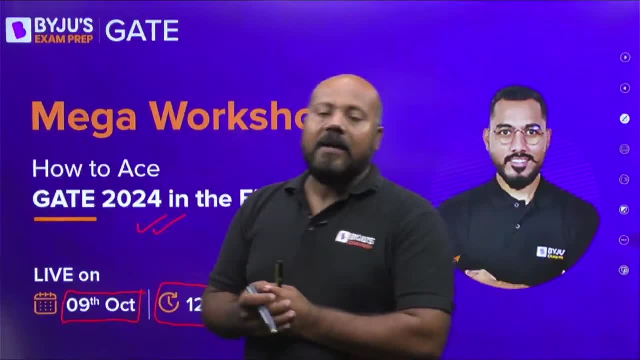 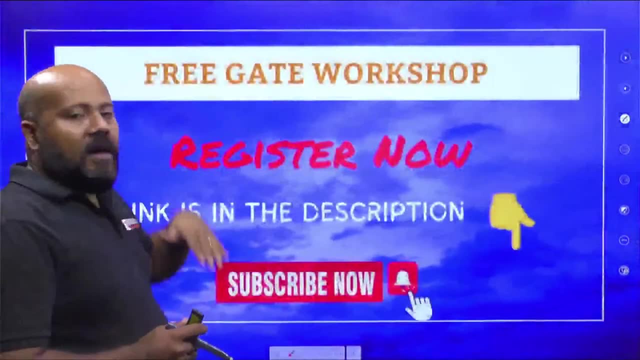 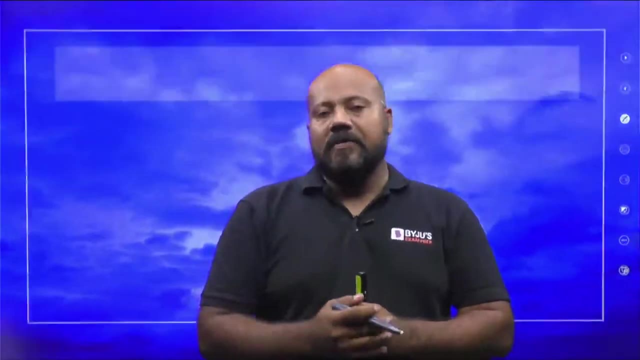 gate 2024, then this is the workshop highly, highly recommended for you now. for this workshop, you have to get yourself registered and the link for the registration is given in the description of this video. after the watching the session, you can follow the description, you will get the link. you can simply fill your details and you can get yourself. 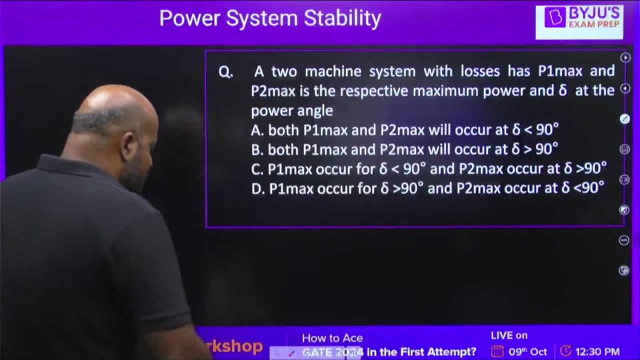 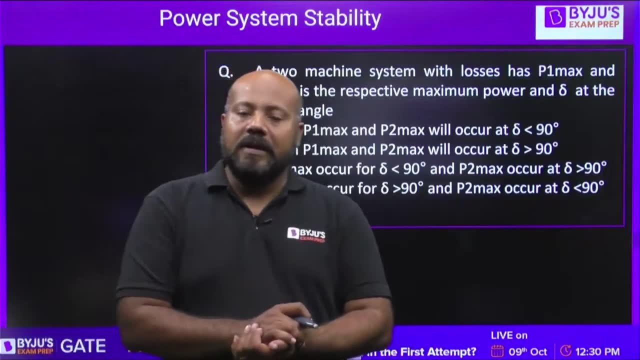 registered. so let me start with the first question. the first question, and before we start the session, let me tell you that today we will be focusing only on the steady state- stability, because of the limitation of the time. some other session i will be discussing upon the transient. 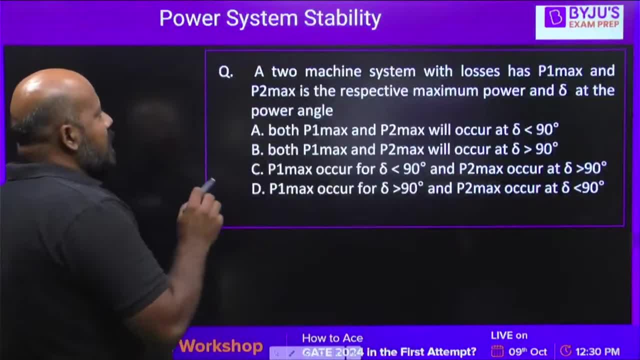 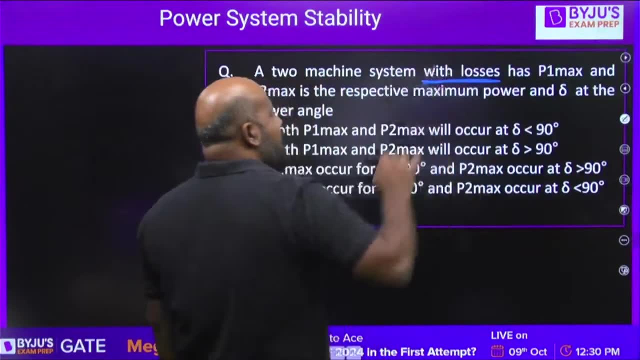 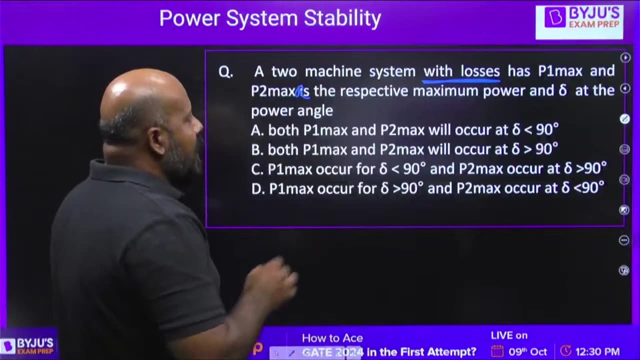 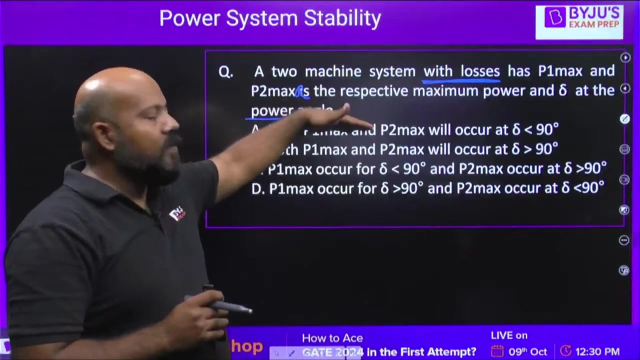 stability also. so he is saying there is a two machine system, is there with losses? two machine system with losses? it has p1 max and p2 max is the respective maximum power and del is the power angle. so he is trying to make some conclusions about the p1 max and p2 max and when they are going to occur. so please try to understand. 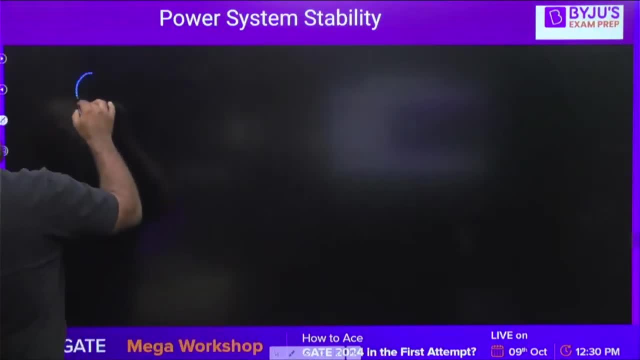 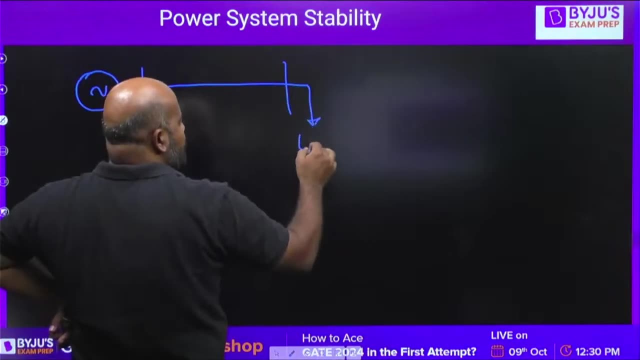 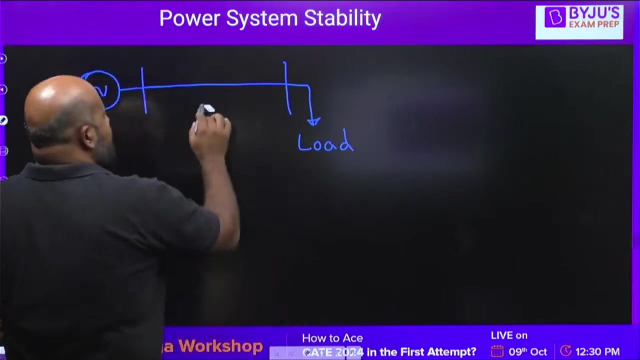 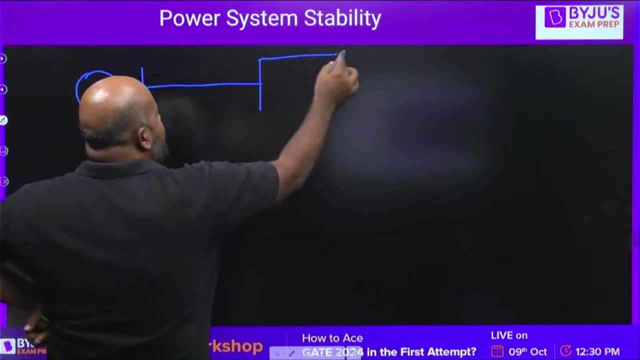 basically, if you talk about a system like this, suppose this is a generator. i am taking a two bus system and suppose this is a load. suppose this is a load, suppose this is a transmission line. or let me take, let me take a more general case. suppose this is any transmission line, because if 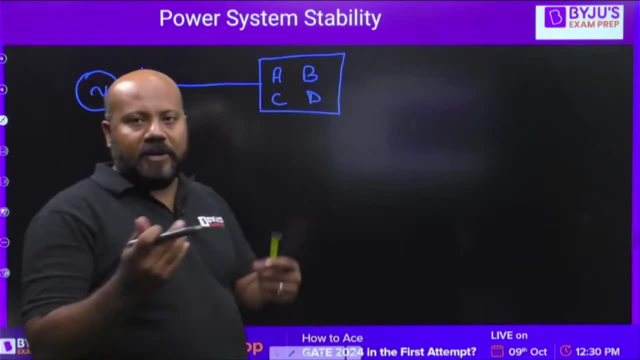 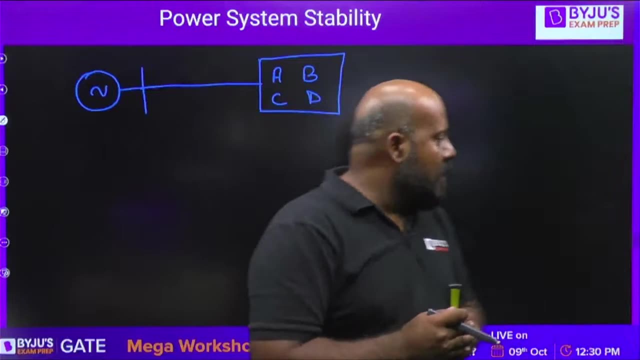 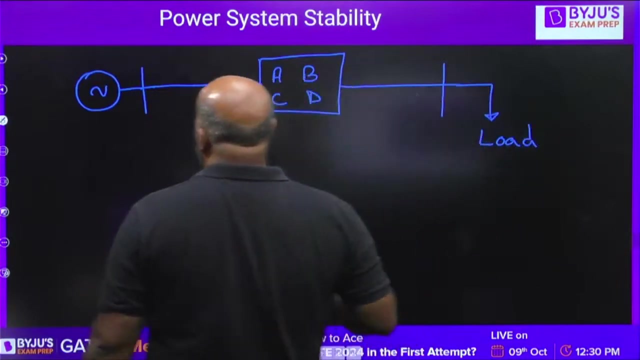 you represent your transmission line with abcd parameters. it is going to be the most general case. depending upon the values you are going to put for abcd parameters, you can do the analysis and suppose this is the load side. some load is connected here. okay, so it becomes the basic model and it is simply meaningless. if you look at the future state doubt set and you define hospital year down, we can currently grease vd pronounce去. 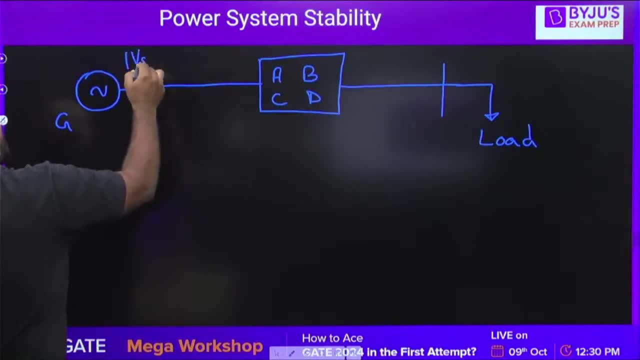 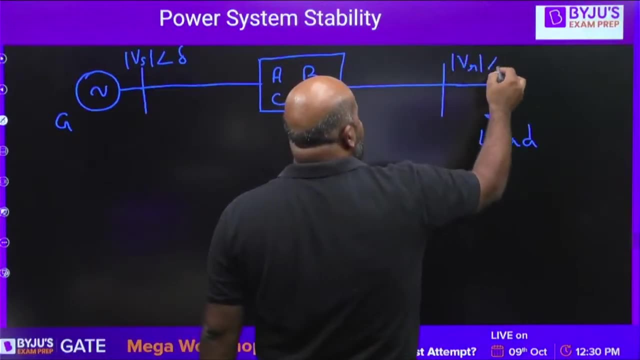 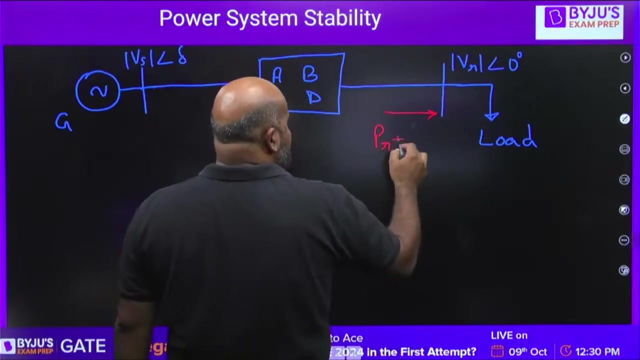 generator. suppose this is the sending end voltage, the angle is del and at the load side it is the receiving end voltage and phase angle is 0 degree. Now here we are talking about the real and reactive power reaching the receiving end, Yes or no? So how we define the stability? 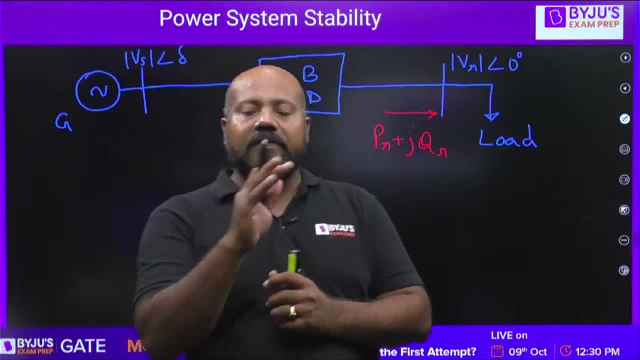 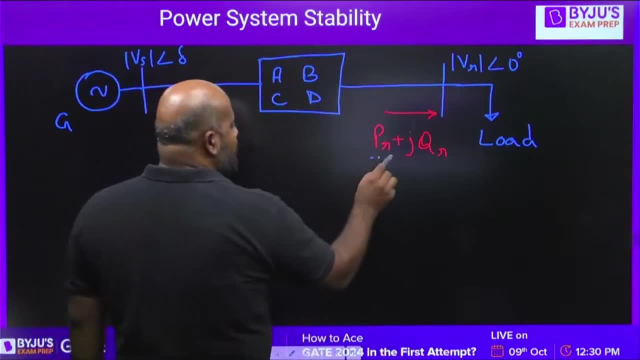 how we analyze the stability. you must be aware that for stability and efficiency, we deal with real power, not with the reactive power. So I am more and more interested to analyze the stability, So I will be focusing upon the real power received. What is going to? 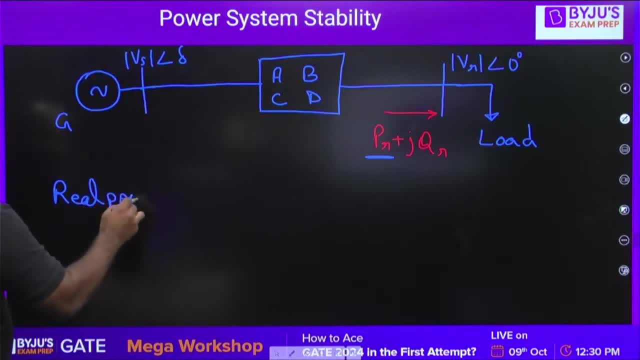 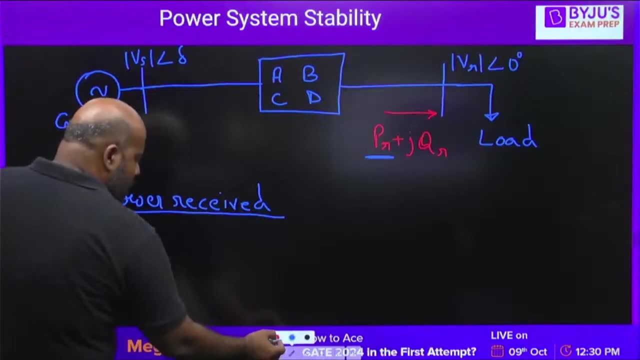 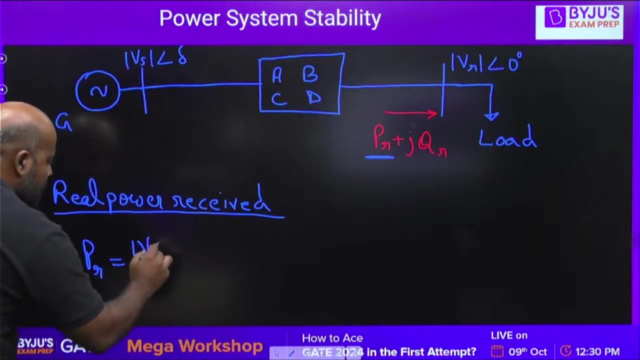 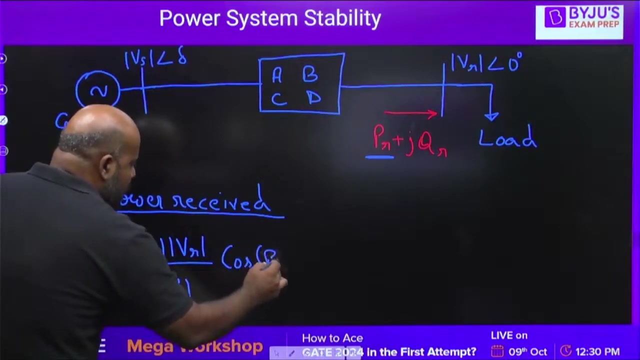 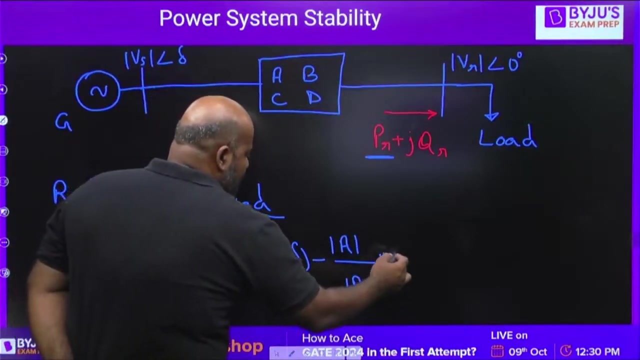 be real power received. Real power received. you must be aware What is the equation. The equation is: the real power received is mod Vs. mod Vr upon mod B, it is cos beta minus del. minus mod A upon mod B, it is mod Vr square cos. 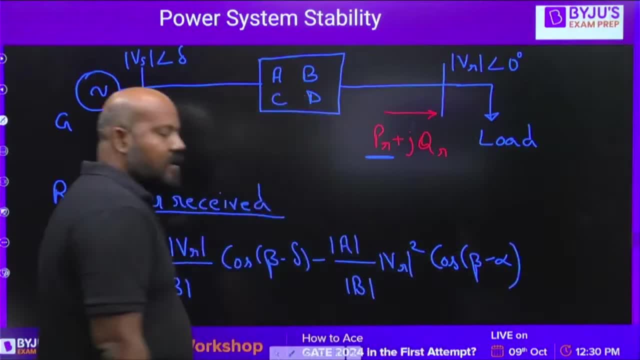 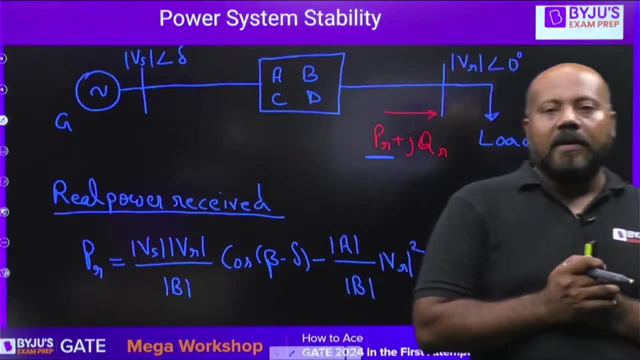 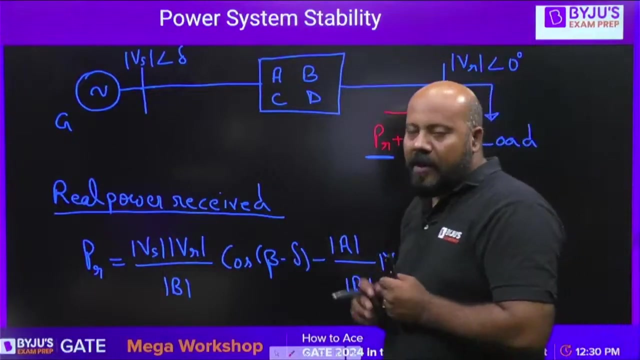 beta minus alpha. This is the general expression for real power received at the load side. Yes or no? Tell me yes or no in the comment section. Now let us understand some of the parameters. What is this beta and what is this alpha? 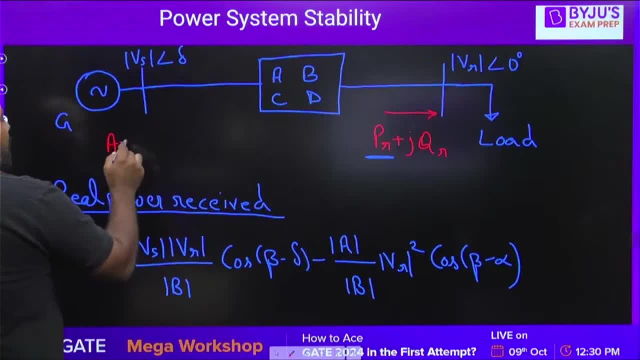 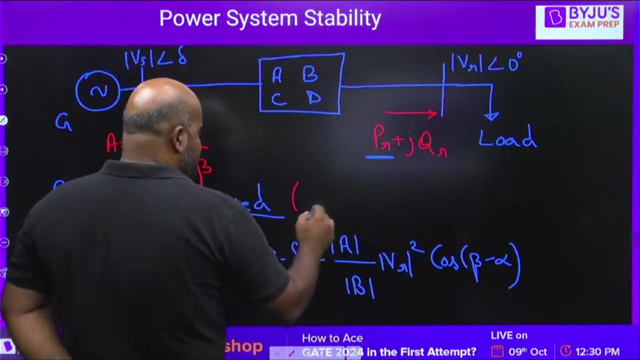 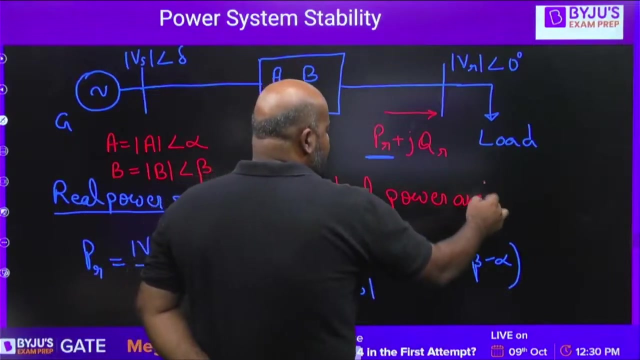 Basically, here in the ABCD parameters we are defining A parameter as magnitude A with angle alpha and B parameter as magnitude B and angle is beta. Now this equation we are calling as power angle relation, actual power angle relation. If you do some simplification, 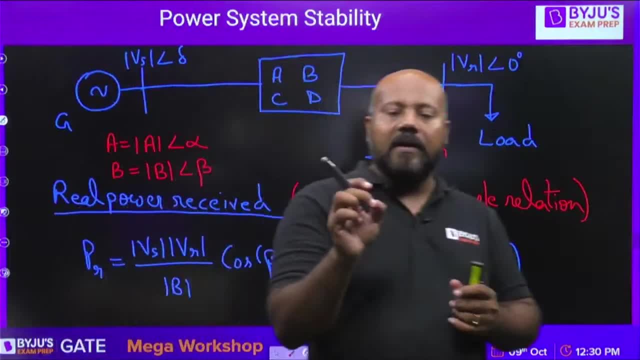 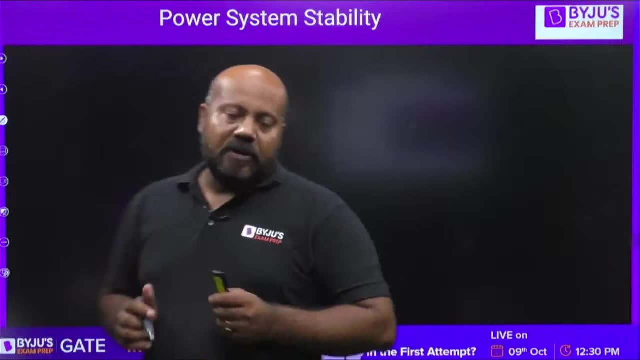 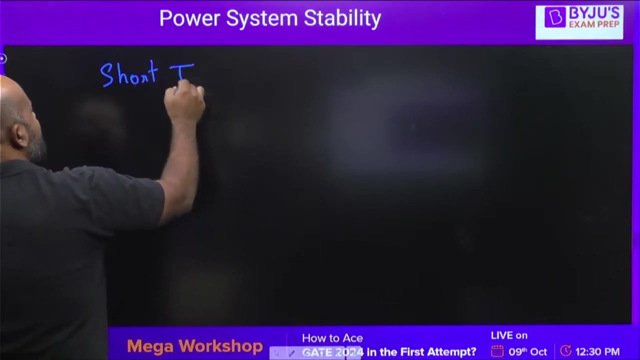 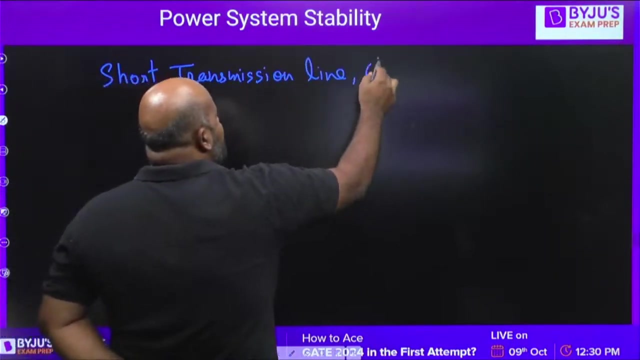 if you have some approximation, then you get the simplified formula that we are using most of the time. So let us understand what are the approximations. The approximations are for a short transmission line, If you consider that, suppose it is a lossless line. So when it is a lossless line, it means what? 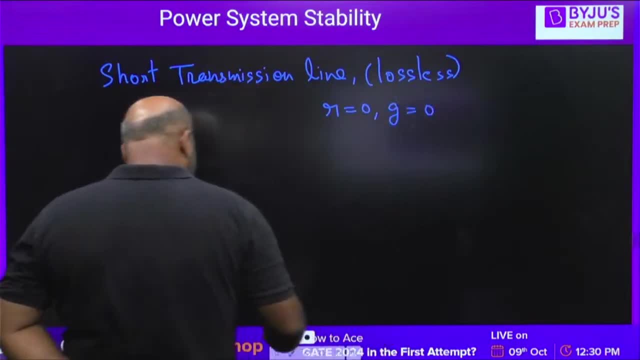 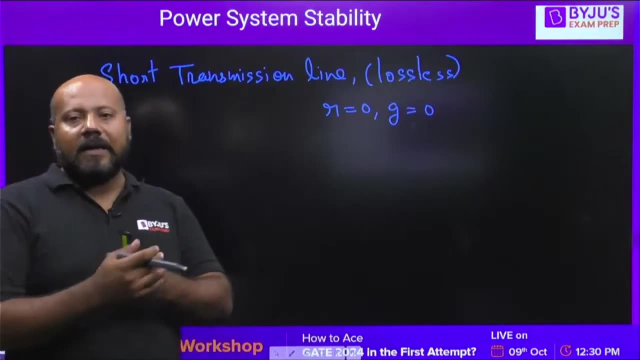 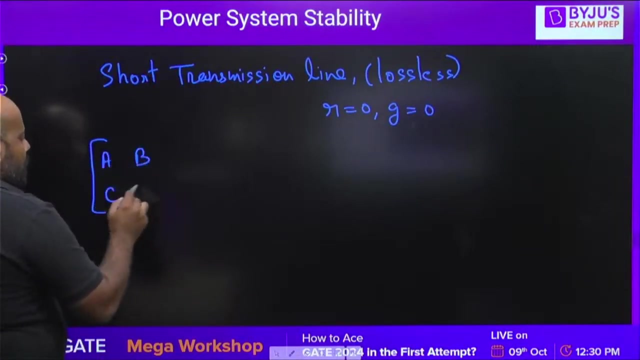 R0,, G0, yes or no. In case of a long transmission line, you can say like that, or simply you can say the resistive part of the line, impedance is going to be 0. So if you see the ABCD parameter for a, 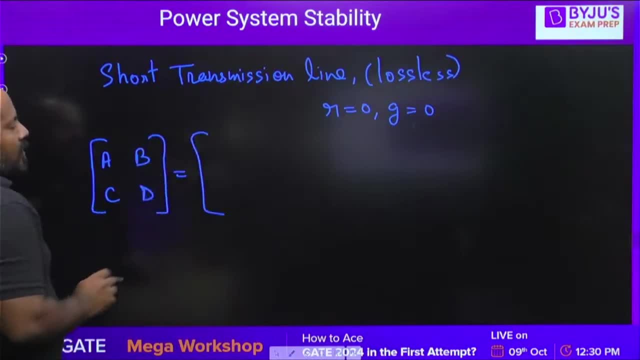 for a short transmission line. with the lossless condition it is going to be 1, jx 0, 1.. Yes or no? If you compare the A parameter and B parameter, you will get to know that A is going to be 1. 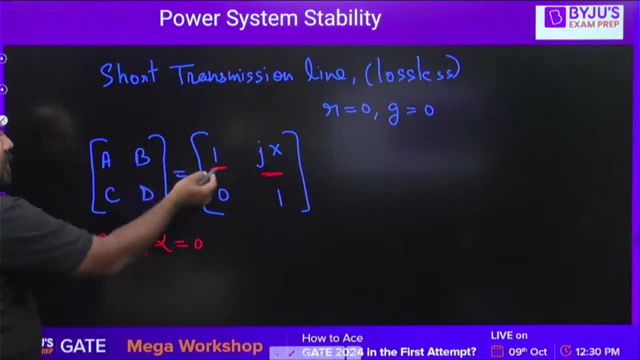 and alpha, that is, the phase angle of A, is going to be 0 because it is simply 1.. What is going to be B? The magnitude of B is simply going to be x and its phase angle is going to be 90 degree because it is jx. Let us put these values, these approximation. 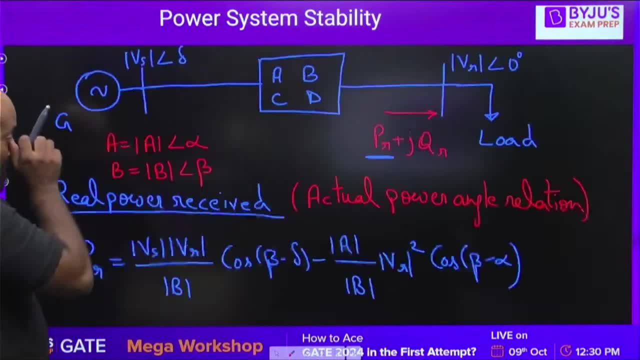 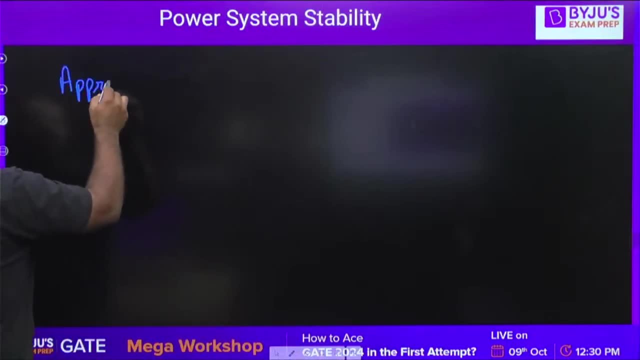 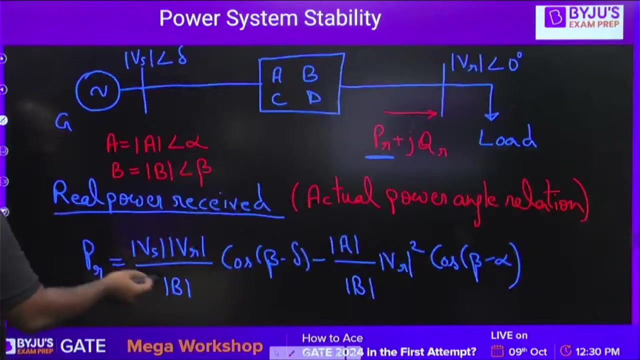 in this equation and see what is the equation you are getting. This is what we are calling as approximate power angle relation. Okay, approximate power angle. So if you put mod Vs, mod Vr, mod B is simply going to be x, Then it is cos. 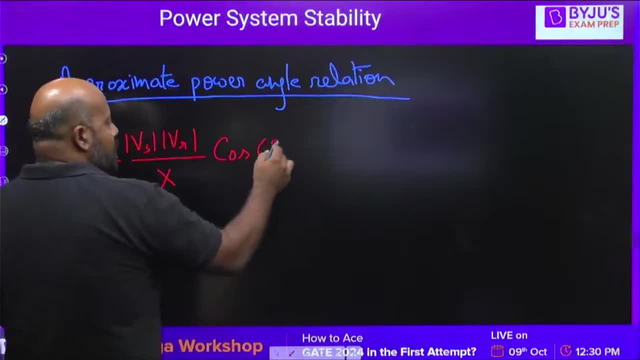 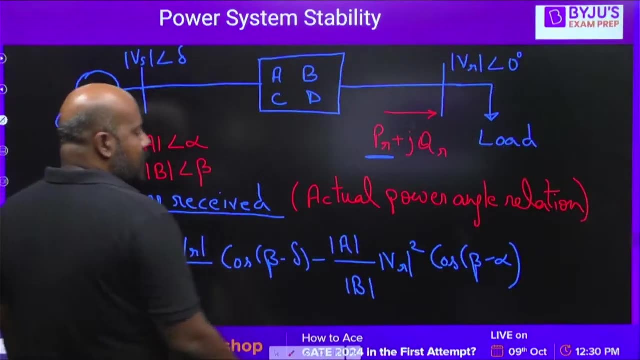 it is beta minus del What is beta. Beta is 90.. So it becomes 90 minus del minus mod A. What is mod A 1.. What is mod B x? It is Vr square upon x, mod Vr square upon x. 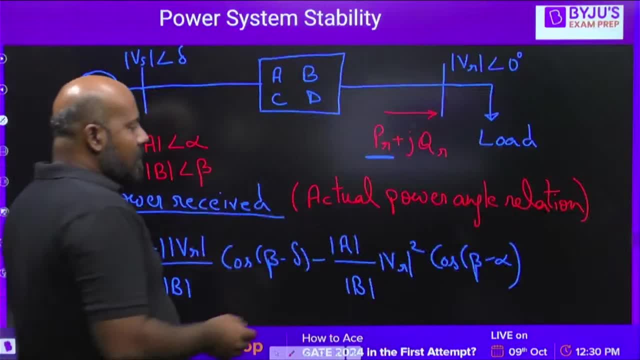 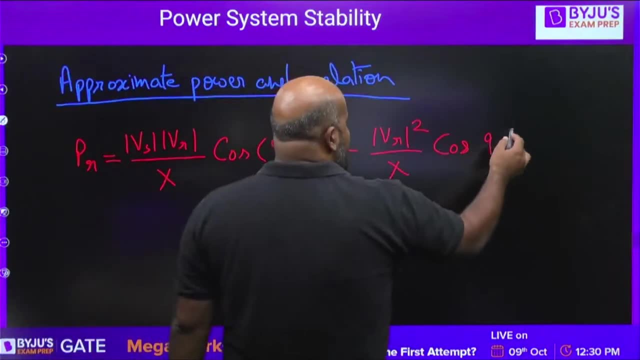 Then it is cos. And what is beta? Beta is 90.. Yes or no, Beta is 90.. What is alpha? Alpha is 0.. So it is cos 90 degree. Now you know that cos 90 is going to be 0. So it is simply 0.. 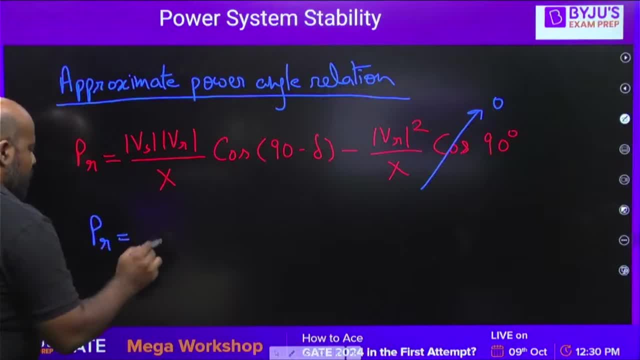 If you simplify this more, you can write: the real power received is mod Vs, mod Vr, mod, sorry, x or cos. 90 minus del is simply sin del. Everybody. just tell me in the comment section: are you able to follow this or not? 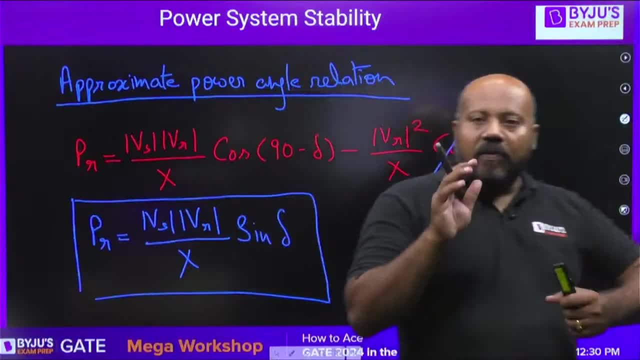 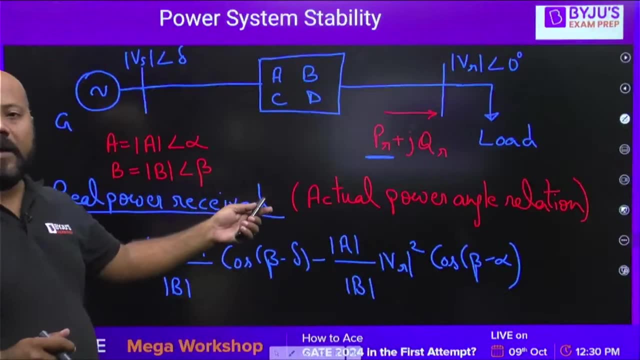 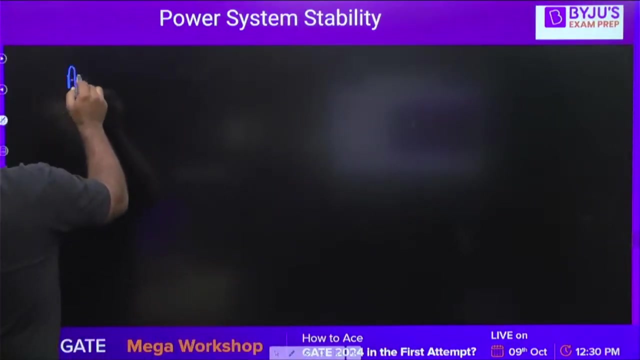 This is the approximate power angle relation. If you draw the power angle curve for both the cases- actual power angle relation and approximate power angle relation- If you see actual power angle curve, then you can write it. Sorry, you can draw it like this. 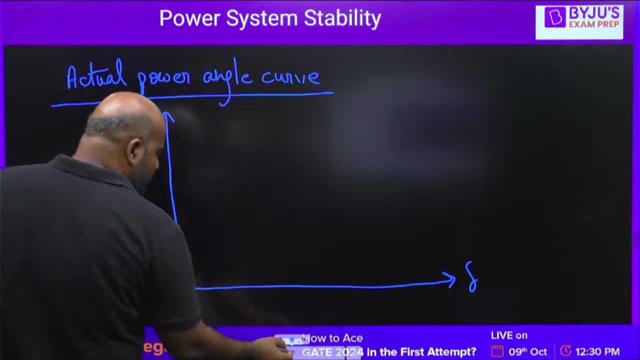 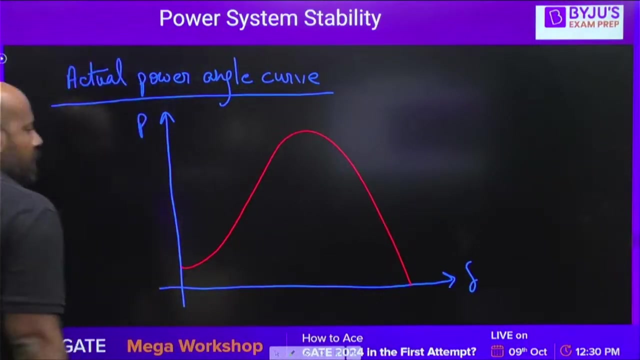 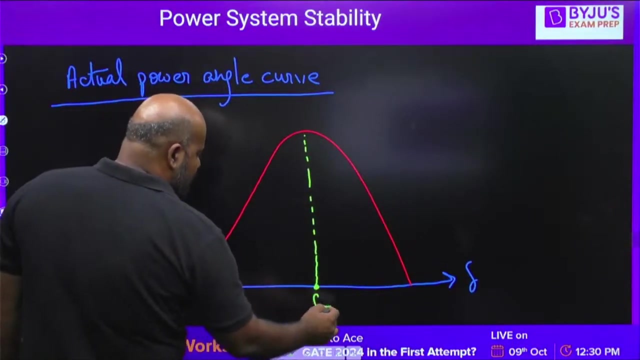 Del. this is going to be p value, Something like this, And let me use a different color. So the p max value you will be getting at del is equal to beta. Because if you see this relation, if you see this relation, can you tell me when this 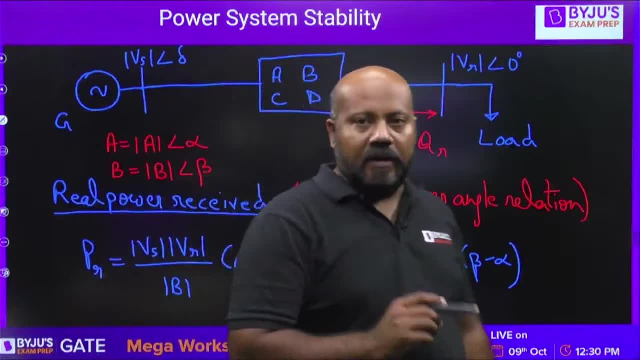 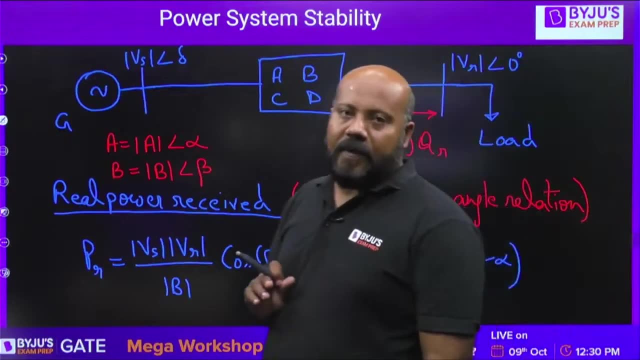 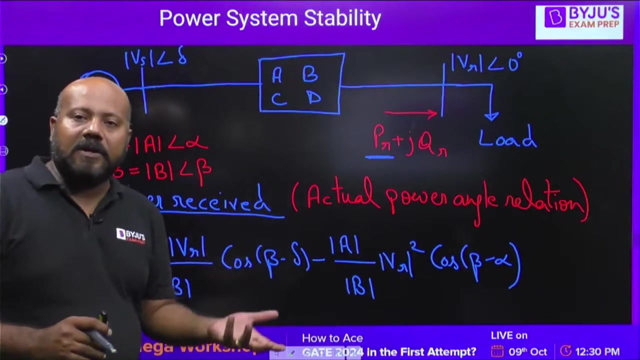 p? r value, the real power received is going to be maximum. Just check The first term: Vs Vr B. we are not changing Because voltage and line constant. we are not changing Cos, beta minus del Beta. we are not changing because line constants are constant. 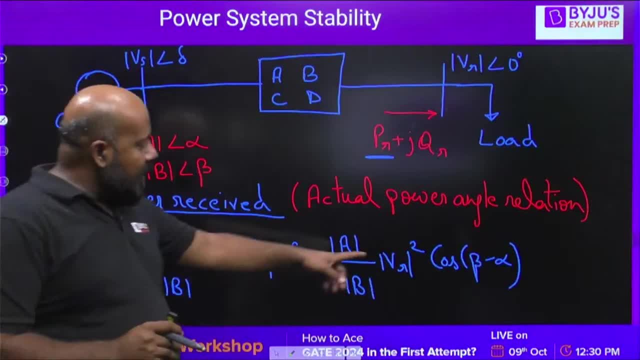 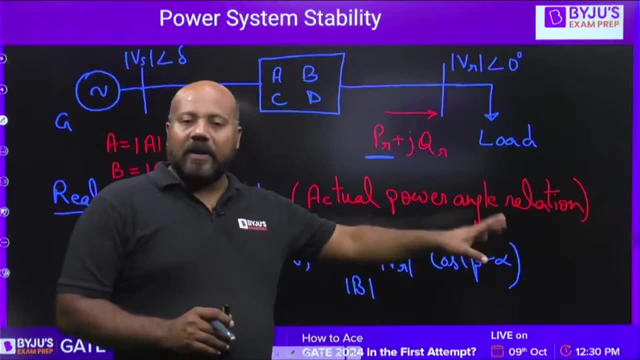 Only del is going to be the variable In the second term. a, b we are not changing Because line parameters Vr, voltage we are not changing. Beta and alpha we are not changing. It means the second term, we cannot change anything. 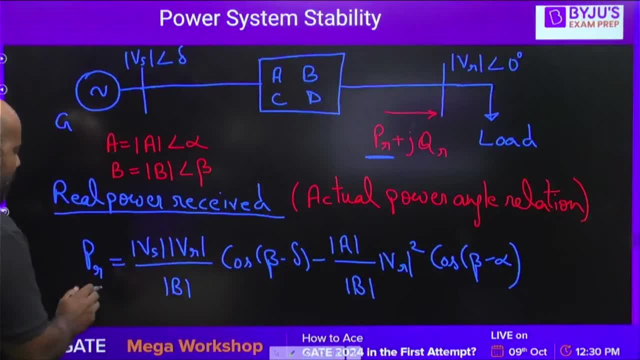 In the first term. only del we can change. So if I want a maximum value for this, then we have to maximize the first term. The first term can be maximum only and only when we make this value as 1.. Because 1 is the maximum value for any sinusoidal function. 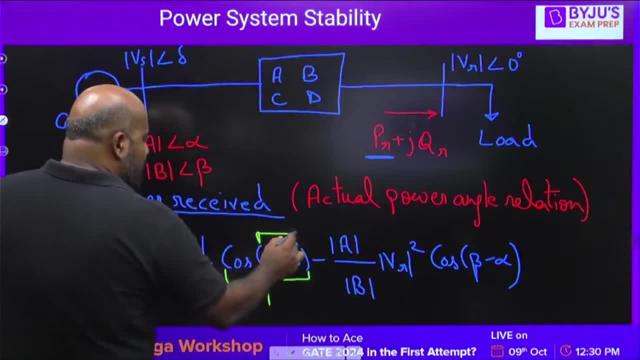 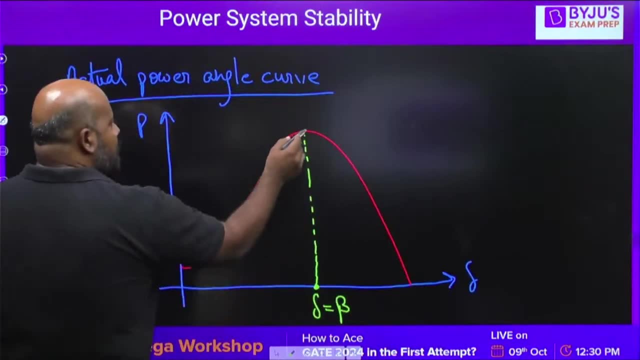 This cos angle is going to be 1.. When the cos angle becomes 1, it becomes 0.. It becomes 0 when del is equal to beta. So at del is equal to beta condition, you are getting the real power. 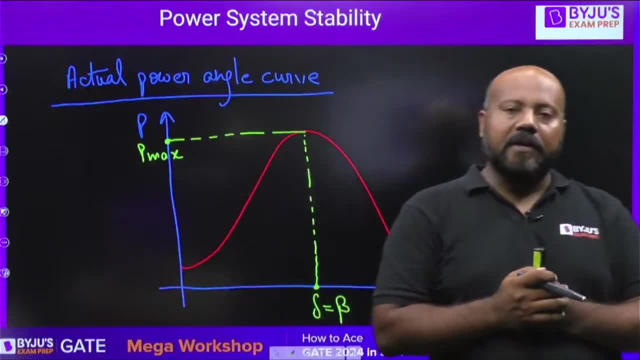 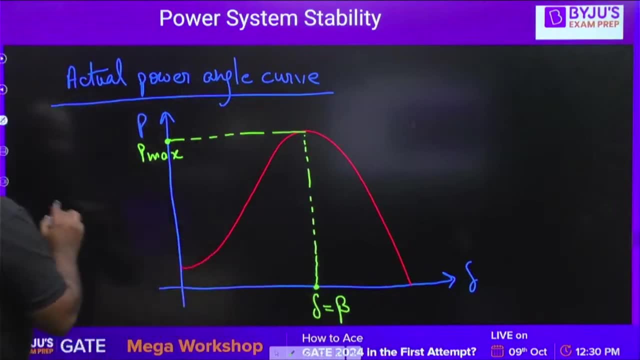 maximum real power received at the load side. Yes, Murli, you are right. Del is equal to beta. Is it clear? everybody Now see here: This beta angle is less than 90, but beta is very close, Close to 90.. 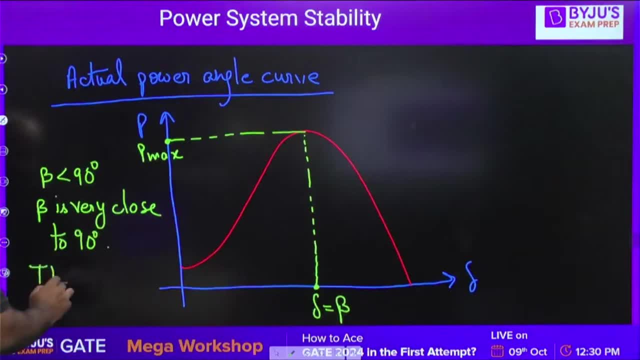 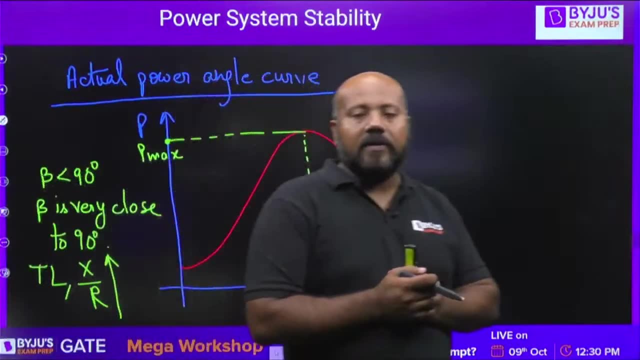 Can you tell me why? Because for your transmission line the x by r ratio is very high. It means the x value is going to be very dominant with respect to the r value. So definitely, beta value is going to be very close to 90 degree. 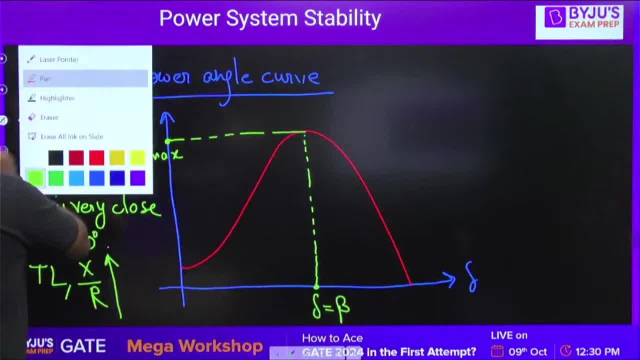 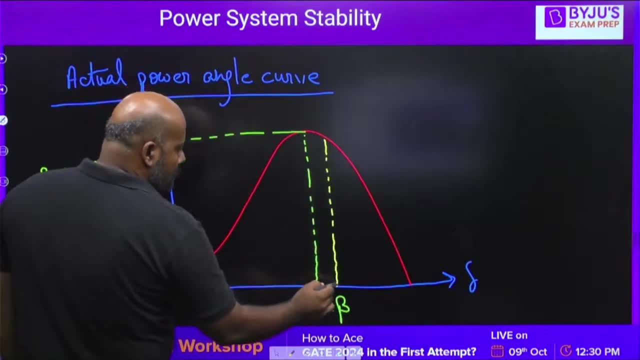 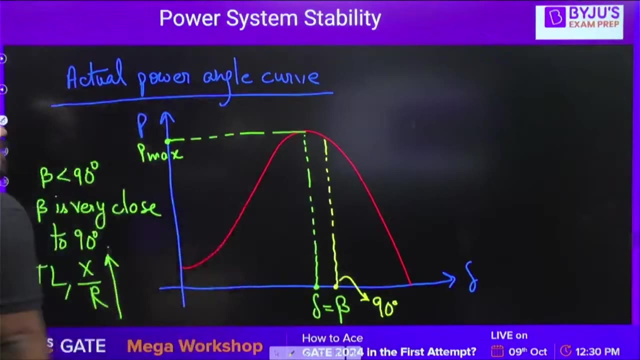 So if you want to draw it, you can draw it. for your understanding purpose, Let me use another color. This is going to be your 90 degree, because beta is just less than 90 degree. This is the case for actual power angle curve. 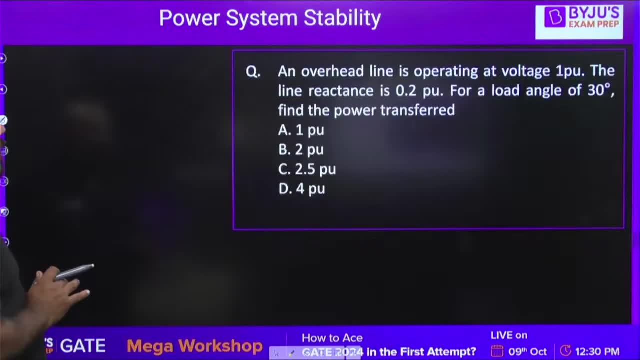 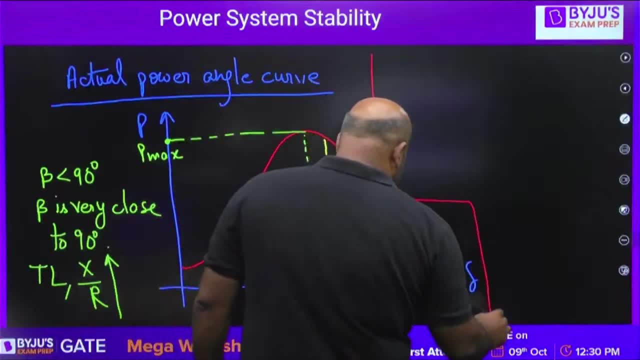 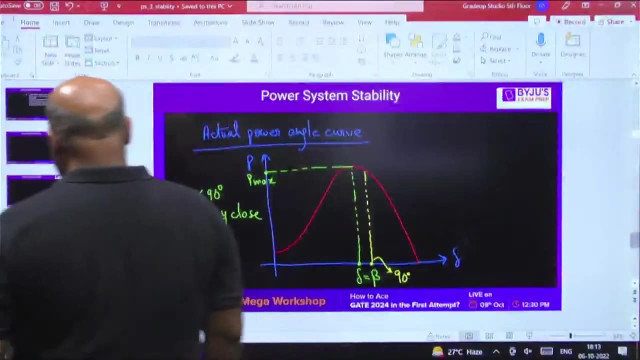 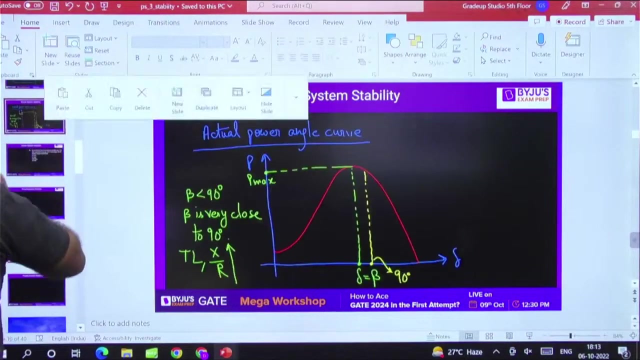 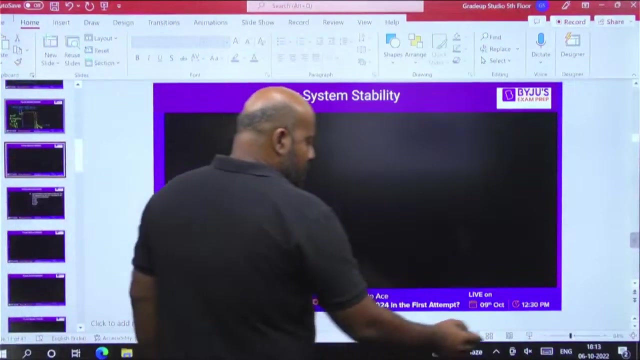 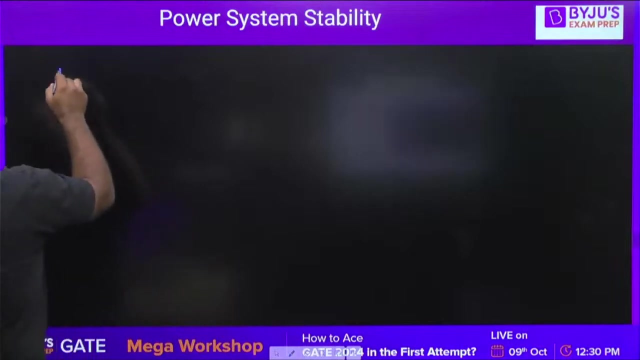 I hope everybody is okay to follow this. If you want, then you can draw the approximate power angle curve also. I am drawing here only. Otherwise let me use another page, Otherwise it becomes a little clumsy. So let me draw for actual power angle curve. 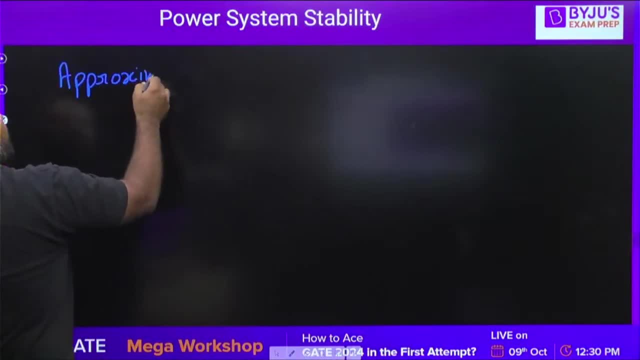 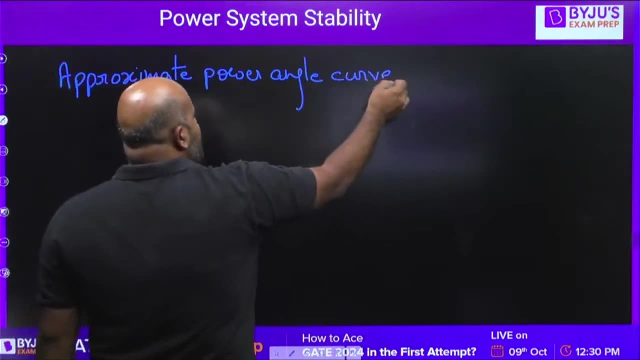 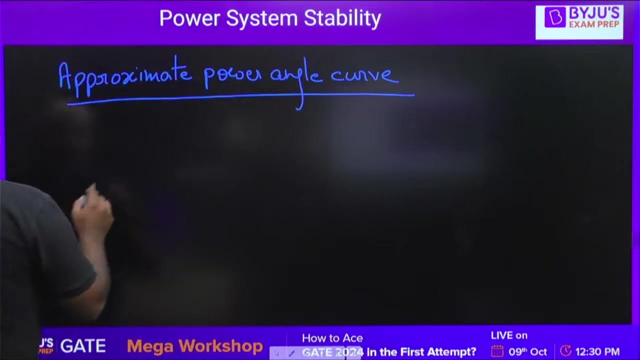 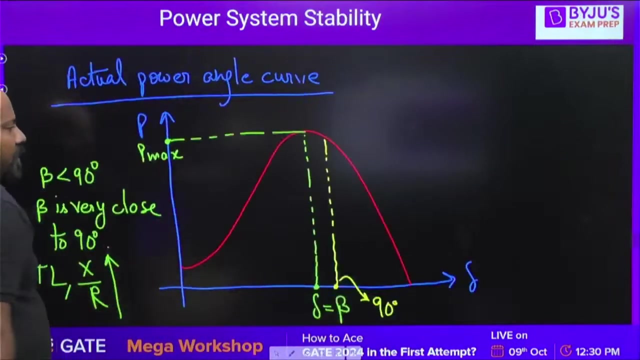 Sorry, approximate power angle curve. So let me draw for actual power angle curve. Approximate power angle curve. Now see here If you see the equation for approximate power angle curve. this equation is nothing but a pure sinusoidal function. 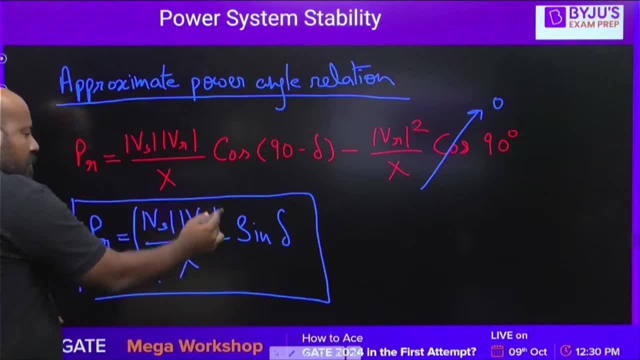 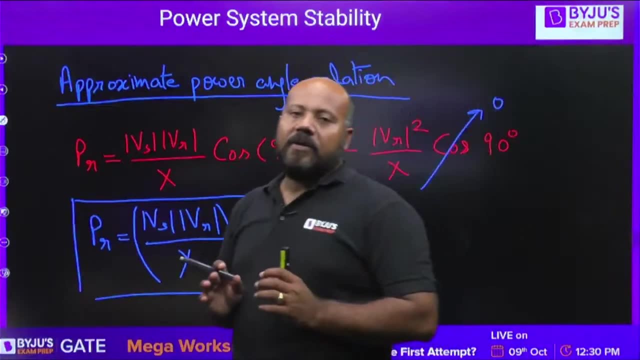 It is a pure sinusoidal function. This is the magnitude. This is the magnitude and this is the sine function, sine del So, some magnitude with the sinusoidal function. It is going to be a purely sinusoidal function And you can very easily draw it like this: 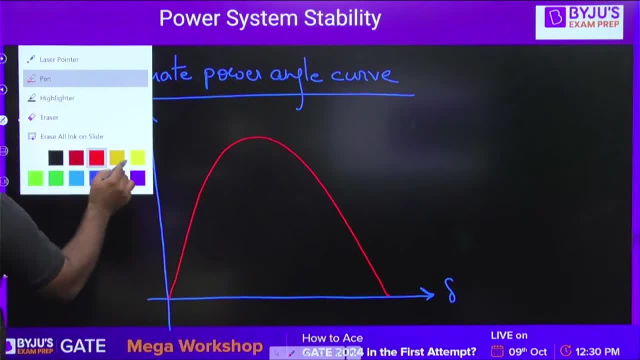 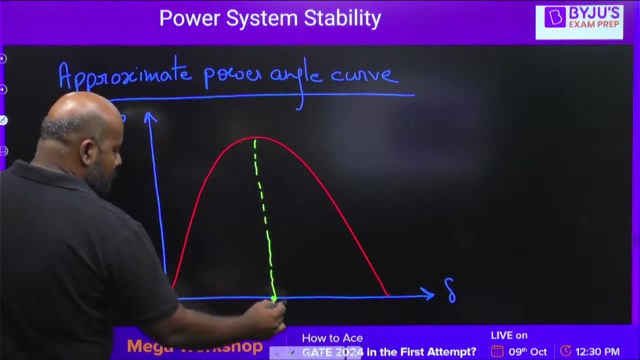 Now let us see when you are going to get the maximum real power received condition. The maximum real power received condition is going to be: del is equal to 90 degree And this is your P max value, Yes or no? In this question he is only talking about. 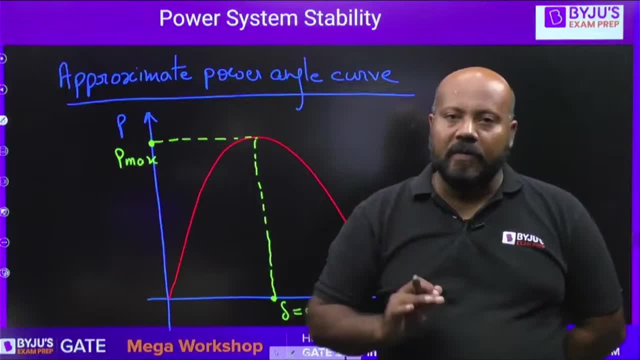 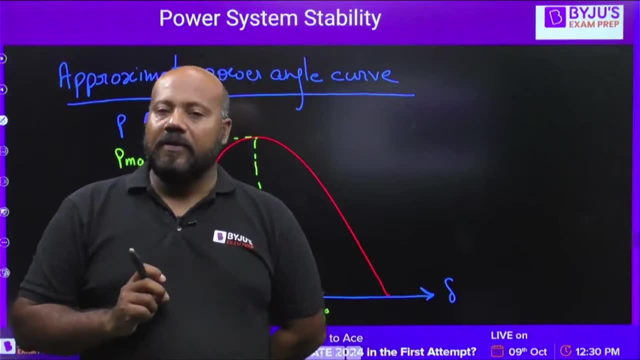 the P1 max and P2 max. But I will give you a little more information so that you get the complete idea of stability, especially steady state stability, when you are dealing with the actual power angle and approximate power angle. Okay, It is not related to the question. 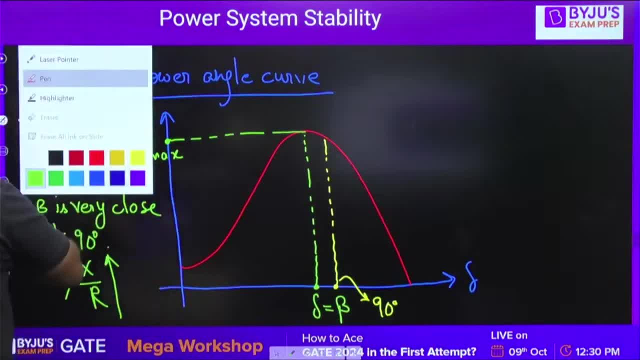 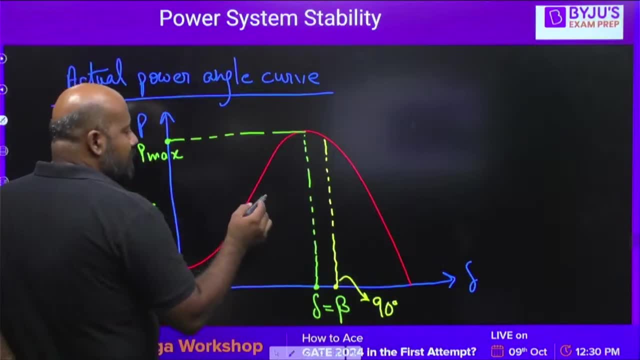 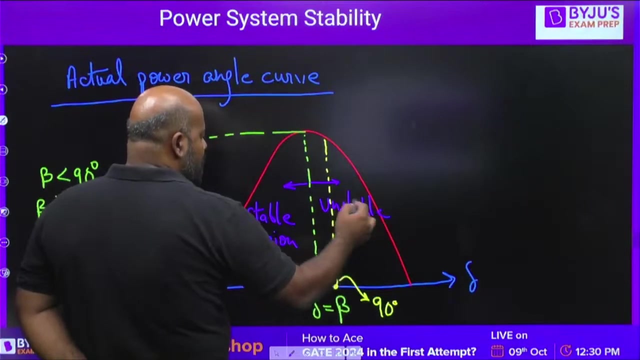 but still, I am telling you, If you observe properly, the stability regions are mentioned in the equation Like this. The stability regions are mentioned like this: This region we are defining as a stable region, This region we are defining as unstable region. 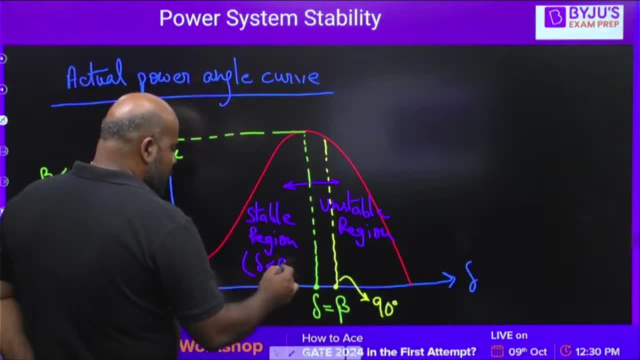 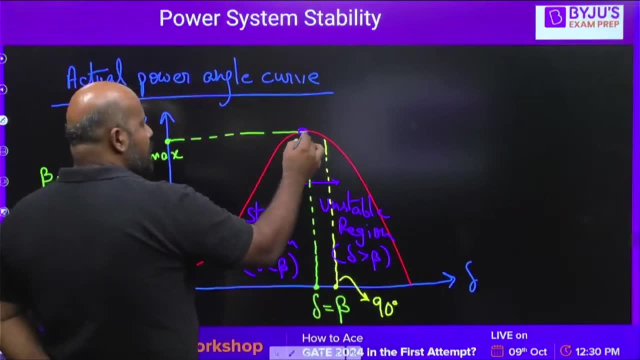 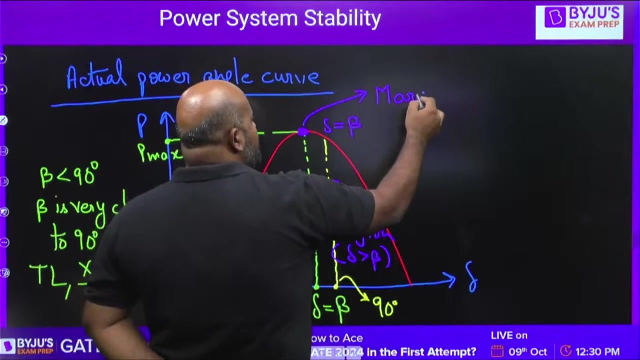 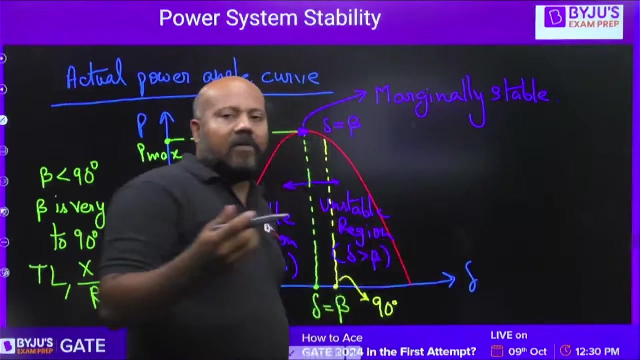 It means del less than beta is the stable region and del greater than beta is the unstable region, Whereas del is equal to beta is the marginally stable point. In brief, you can understand what is marginal stability At any point of time. 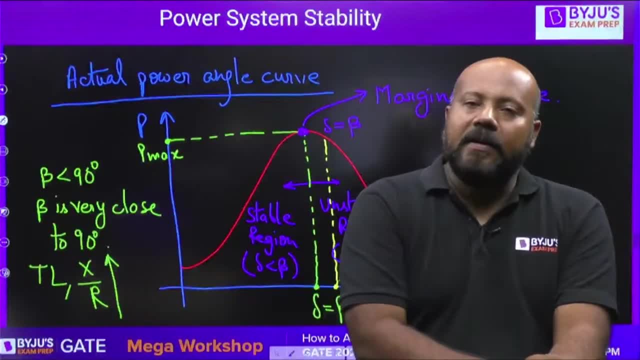 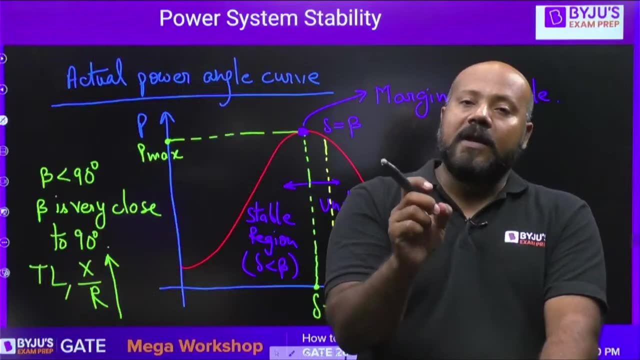 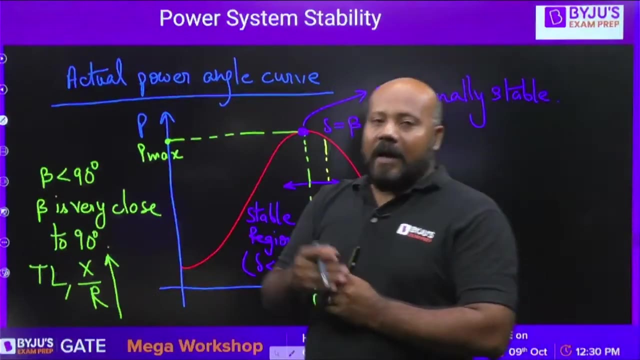 if you try to run your machine at the P max condition- it means the maximum real power received condition- then your machine is at the verge of stability. You cannot predict its behavior After that instant. it may become a stable also and it may become unstable also. 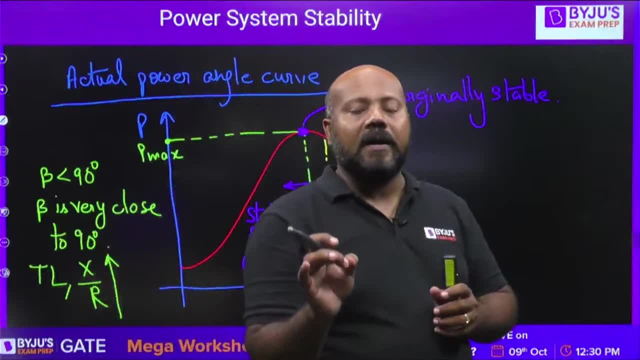 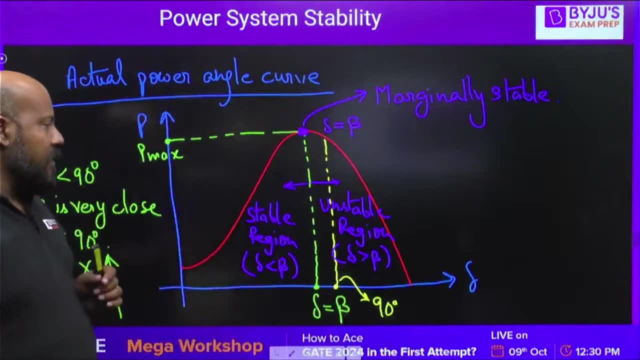 And, because of this, this operating point we are defining as the marginal stability. I hope you are getting this How we are defining the stability. What is the criteria for instability? You can understand Again. I'm using another color. Let me use white color. 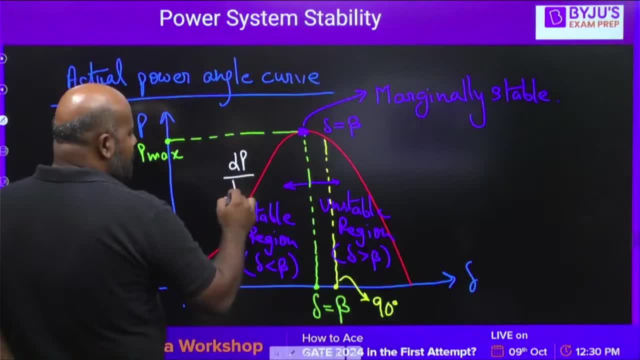 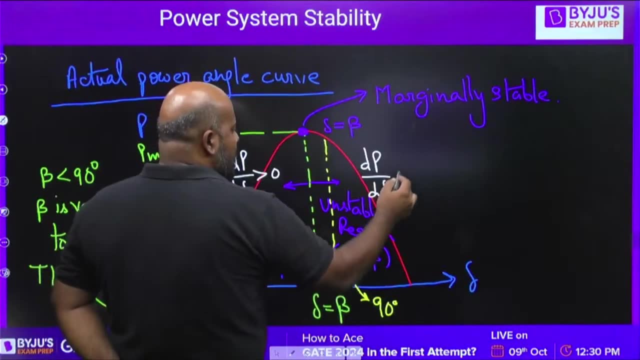 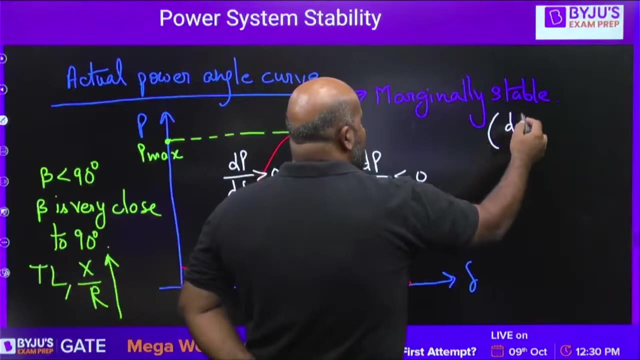 In the stable region, the slope of the curve is going to be positive. In the unstable region, the slope of the curve is going to be negative. Whereas at the marginal stability point, del is equal to beta. the slope of the curve 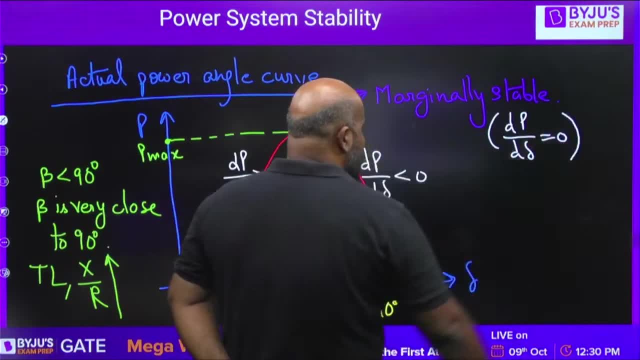 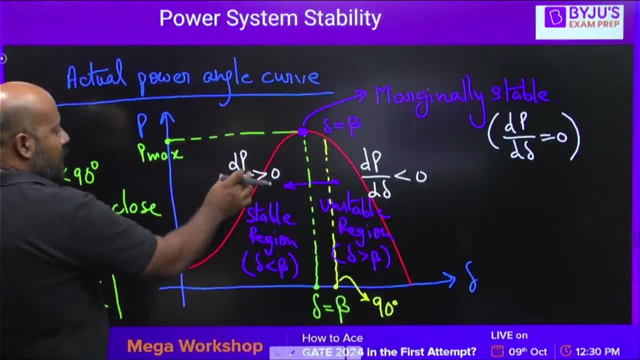 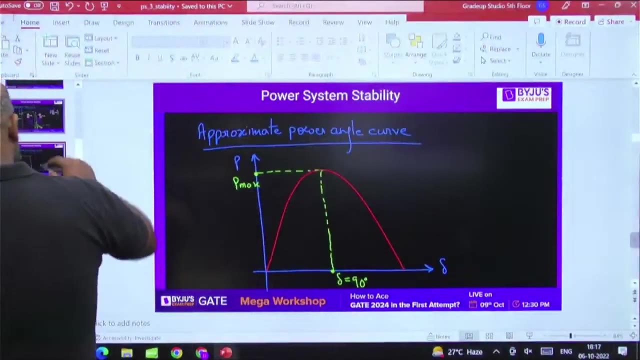 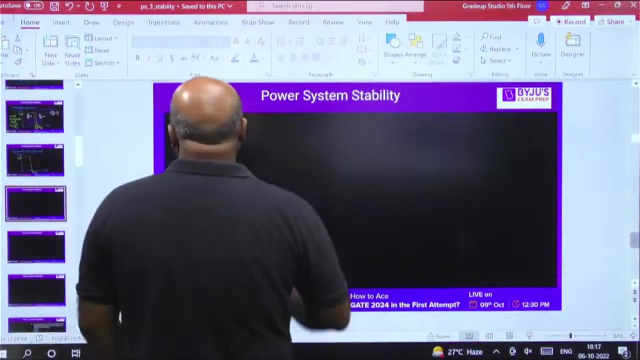 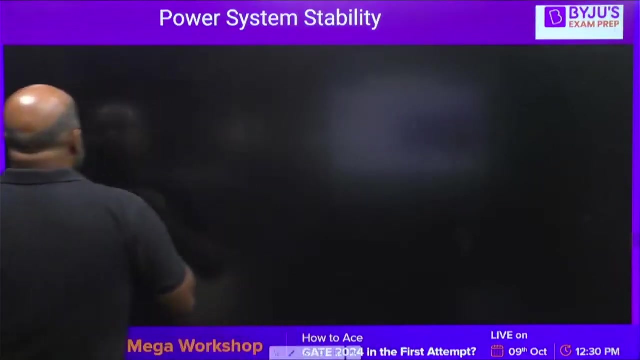 is going to be 0.. What is the meaning of slope of the curve? Let us try to understand. When the slope of the curve is positive. let me add another page here. Let me add another page here. If you define the stable region that the slope is positive, what does it mean? 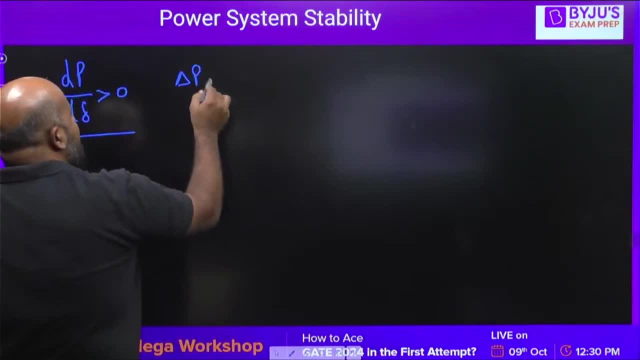 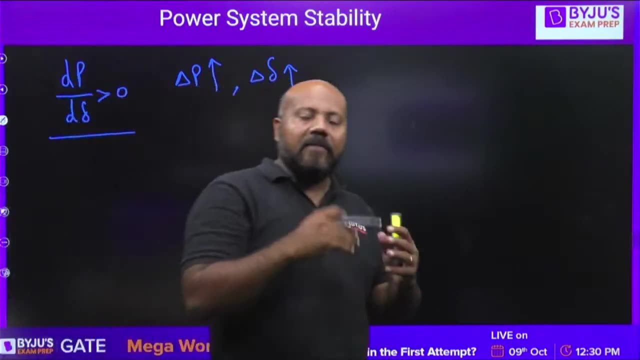 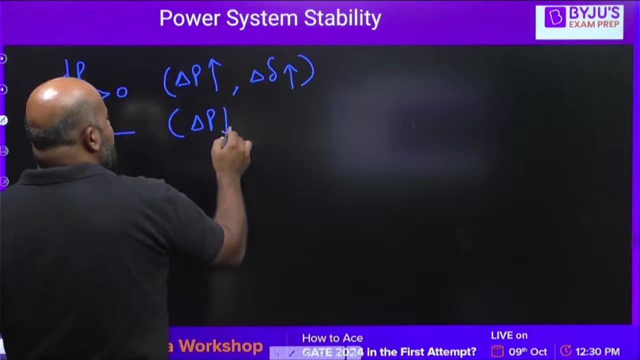 It simply means the change in P. if it is positive, then change in del is also going to be positive. It means if P is increasing, then del will also be increasing. In the same way you can say: if change in P is negative, then change in del is also negative. 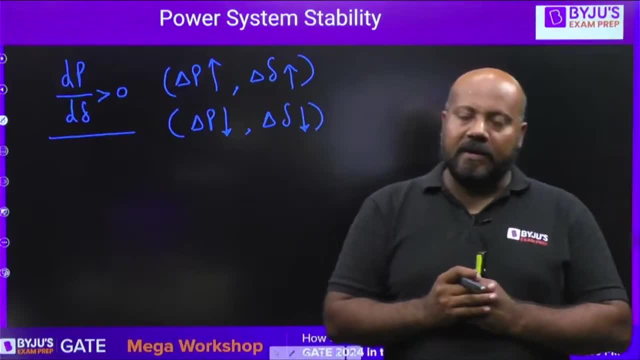 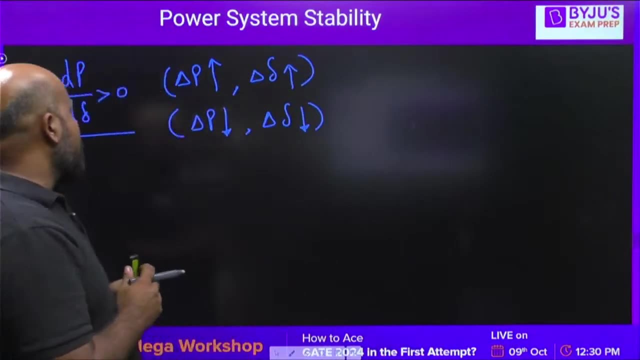 It means if P is decreasing, Del will also be decreasing. And this is the reason we define the slope positive region as the stable region, Because please try to understand what is the meaning of increasing the power demand. If you increase the power demand, what will happen? 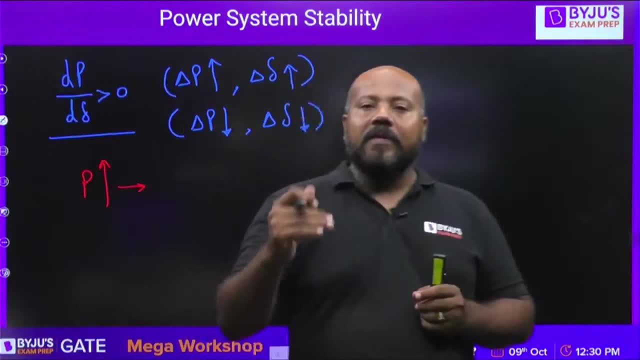 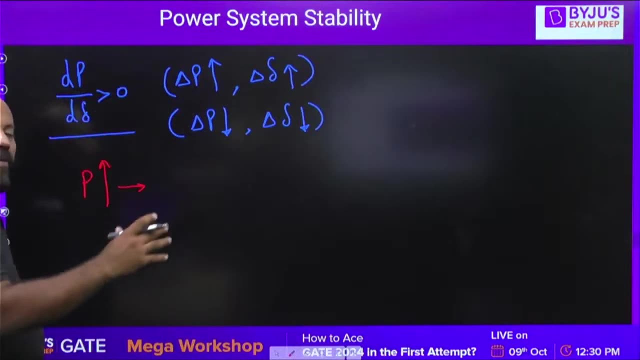 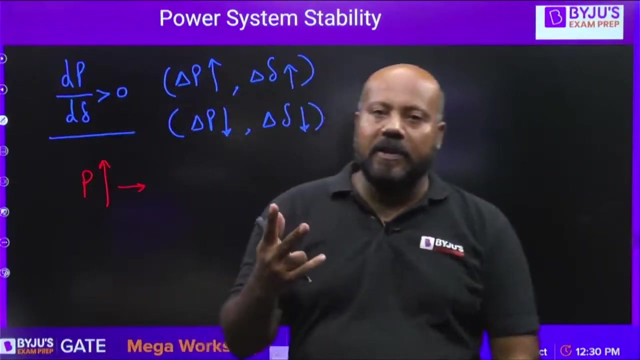 Just try to understand. If you increase the power demanded, then what will happen? In order to supply more power, you must get more steam, Yes or no? If you want to generate more power, there are only two possibilities with your generator. 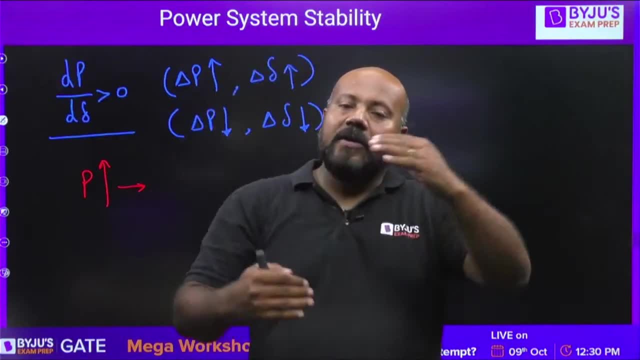 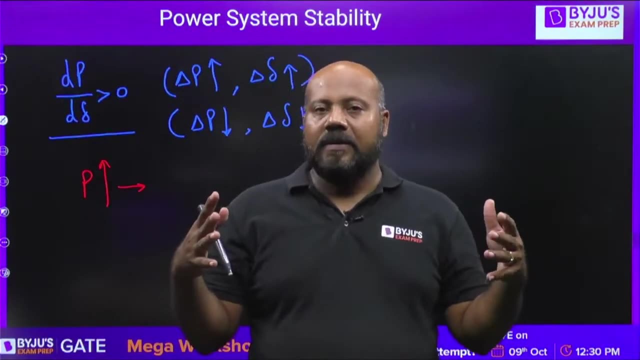 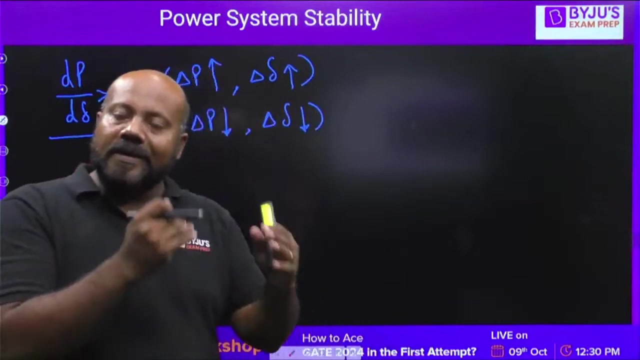 Either you increase the flux or you start rotating your generator with more, higher speed. Yes or no? Now, flux, you are not changing because it will be very complex and there has limitations also. So, flux, you are not changing What you are doing. 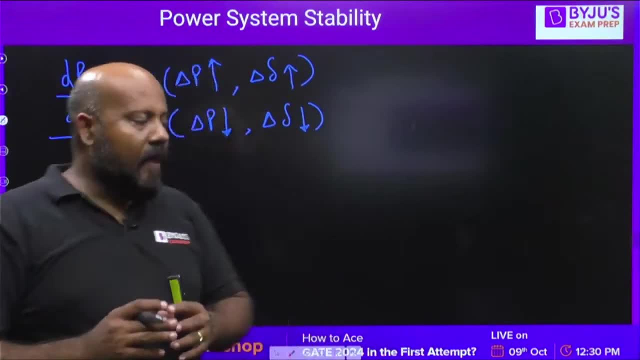 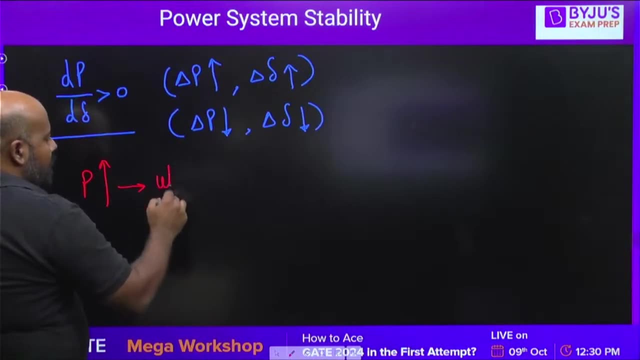 You are increasing the speed of the generator to generate more power and supply more power. So for the load frequency control, Yes or no. For the load frequency control, you can understand: if you increase the power demand, then you give up command. 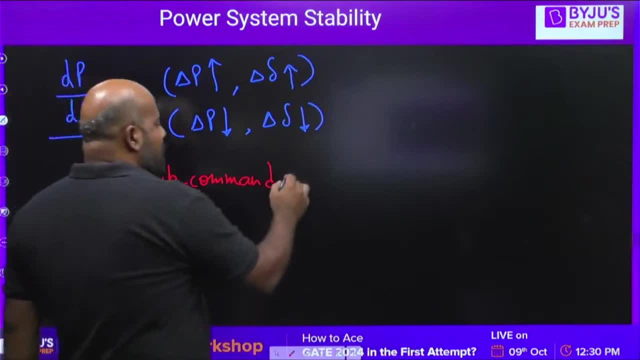 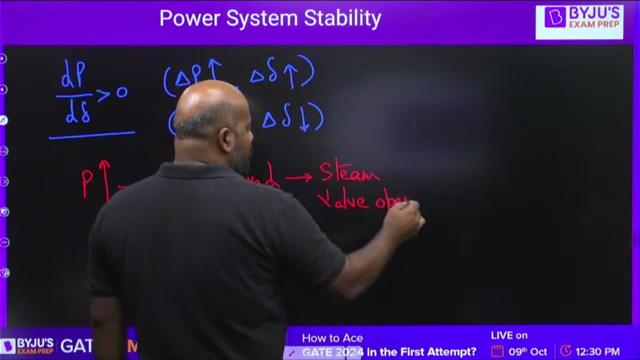 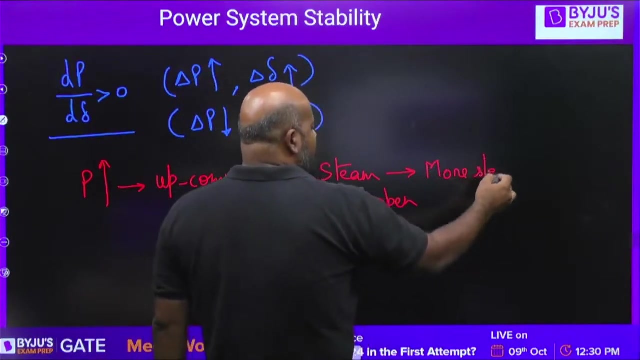 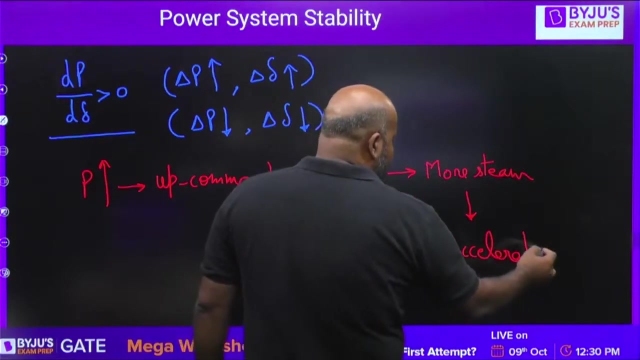 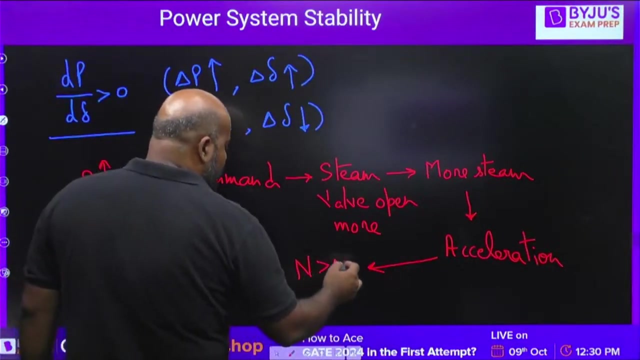 What will happen to the up command? If you give up command, the steam valve will open. It will be opened more, So you will get more steam. More steam means you get acceleration, Yes or no. And when you get acceleration you get speed more than synchronous speed for the time being. 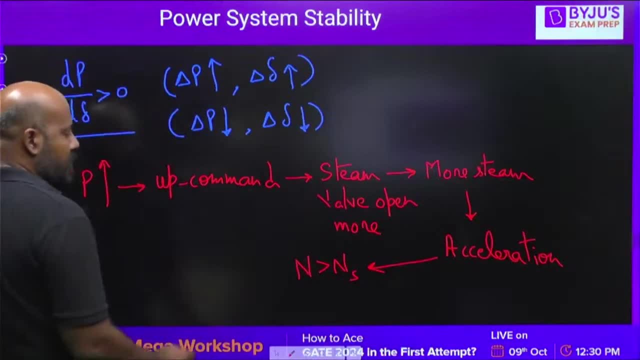 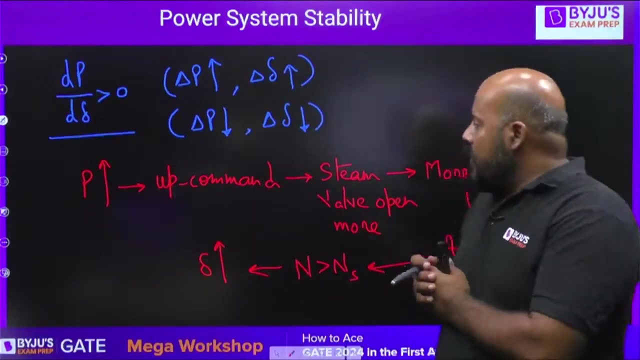 For the time being, Okay, That previous speed is speed more than synchronous speed. So you are getting more power, or you can say more power angle depth. Is it clear everybody, Yes or no? Yes or no, It means when the power demand is increased, the del value has to increase. 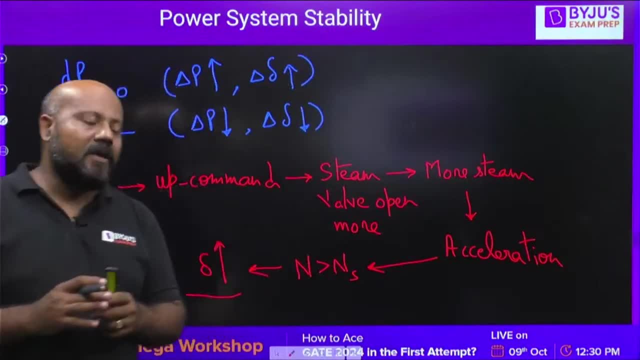 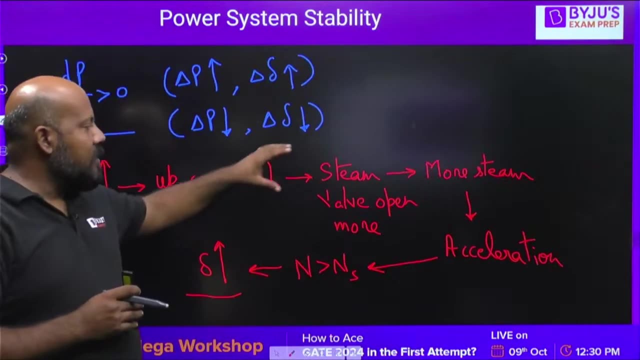 If both these conditions are fulfilled, then you say that your system or your machine is stable. You can also follow the reverse case. when the power demand is reduced, there is a down command. Down command means steam valve will start closing so that less steam is coming and there. 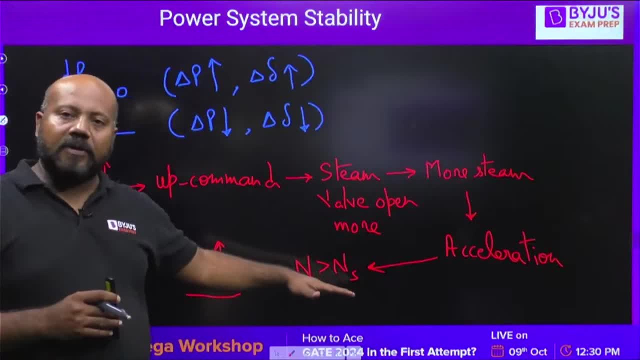 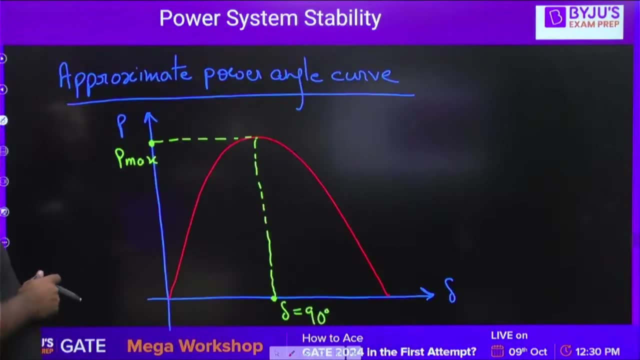 will be deceleration, so that the speed becomes less than the present speed or the synchronous speed, And del is also going to reduce. Is it clear everybody? Yes or no? Yes or no. Yes or no. Yes, that's correct. 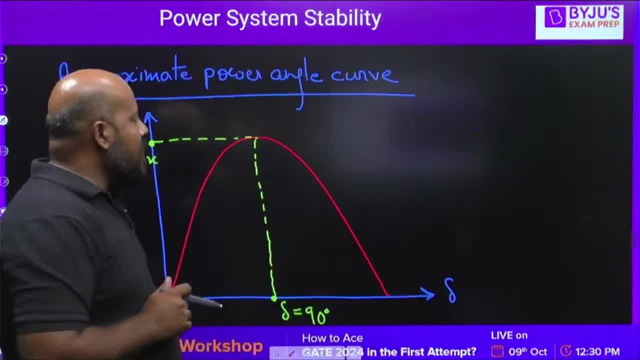 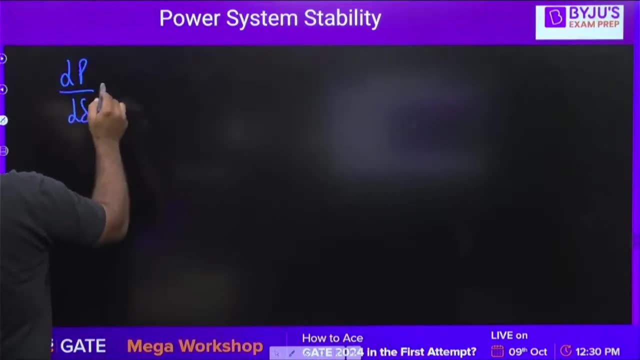 So you can very easily understand about the unstable region. because of the unstable region, what will happen When the slope is less than zero? It means if the change in power is positive, the change in del is going to be negative, or when the change in power is less, then change in del is going to be positive. 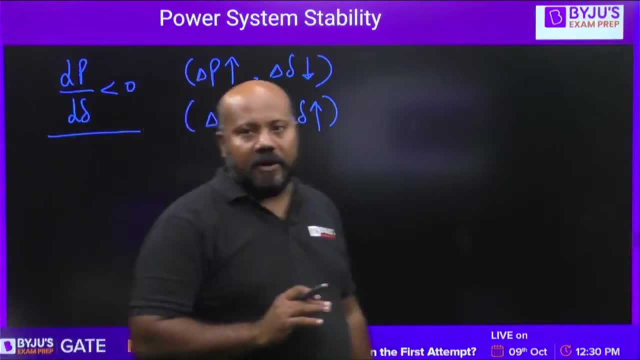 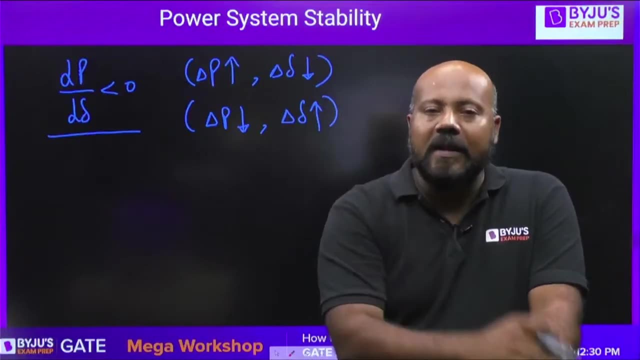 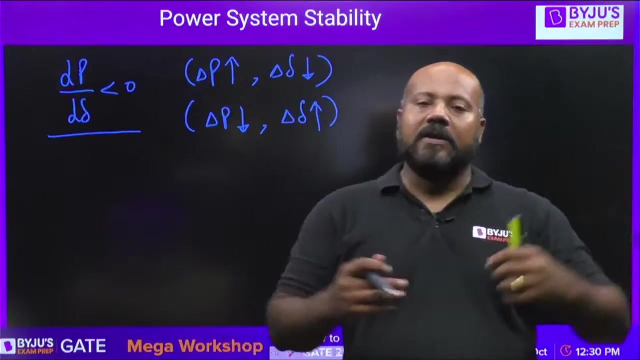 Okay, This is the unstable condition. What is happening? You want to supply more power, but your generator is refusing to take the load, So it is further reducing the power it is being supplied. You want to increase the power: it is reducing its power. unstable condition. 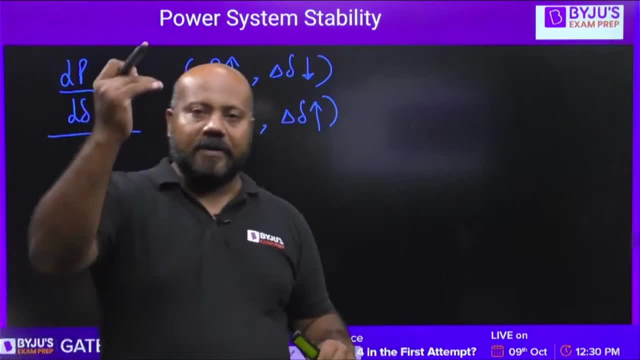 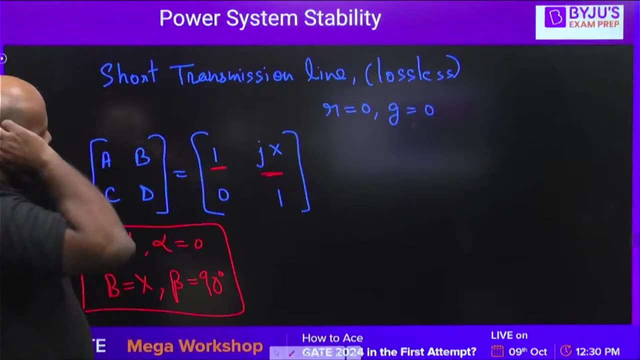 At the same time, if you want to reduce the power, it wants to increase it. So that is the unstable condition. Now, if you see, as per the demand of the question, he is saying when P1 max and P2 max is going, 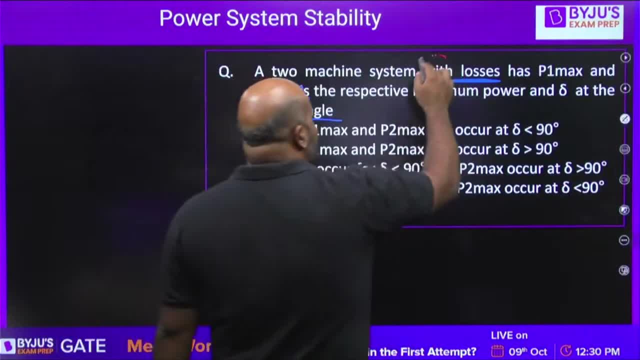 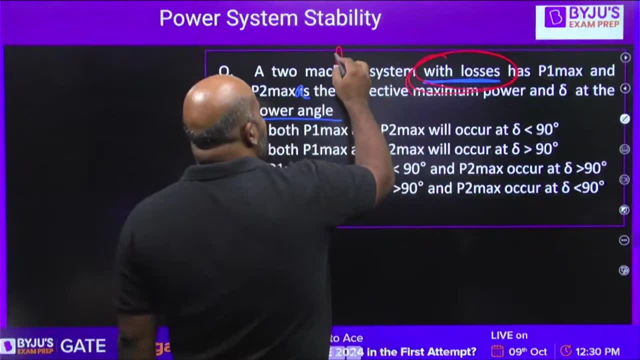 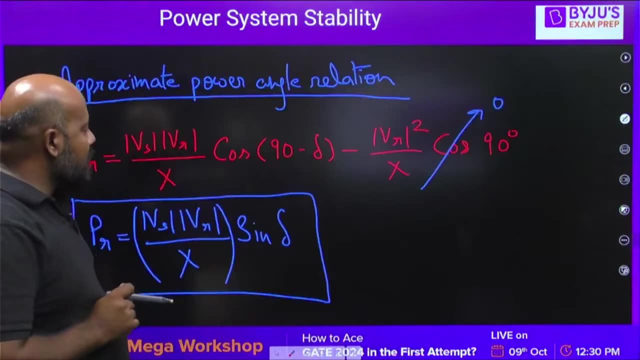 to occur. Because in the question he has mentioned about the losses, he is saying there are losses in the system. When there are losses in the system, then you have to use the actual power angle curve and actual power angle equation. In that case you have to follow this curve, yes or no? 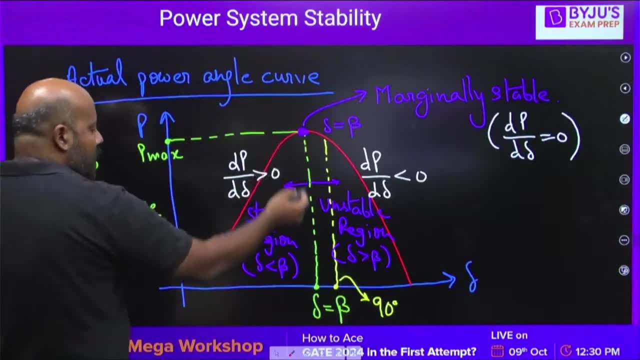 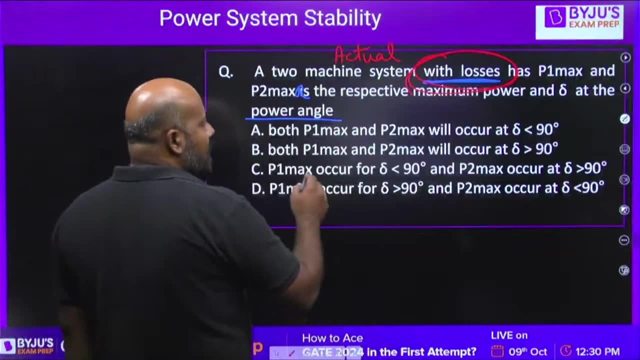 So this curve, you can very well understand that P1 max or P2 max, both are going to occur. P1 max is going to be at angle del, which is less than 90.. For both of the cases it is going to be less than 90.. 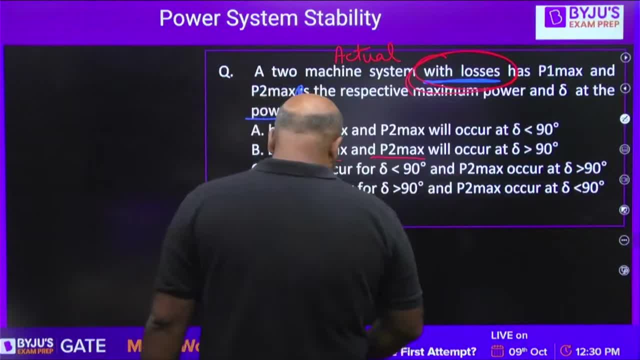 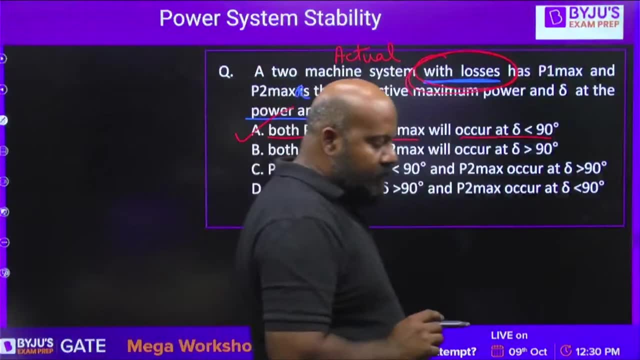 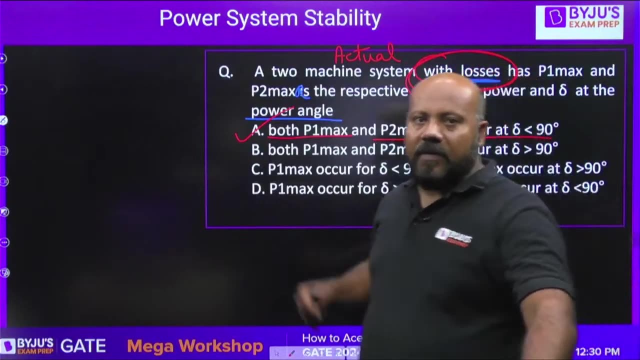 So both P1 max and P2 max will occur for del angle less than 90.. What is the correct answer? A is the correct option. Is it clear? everybody, Everybody who is joining me live, just quickly confirm: are you able to follow this or not? 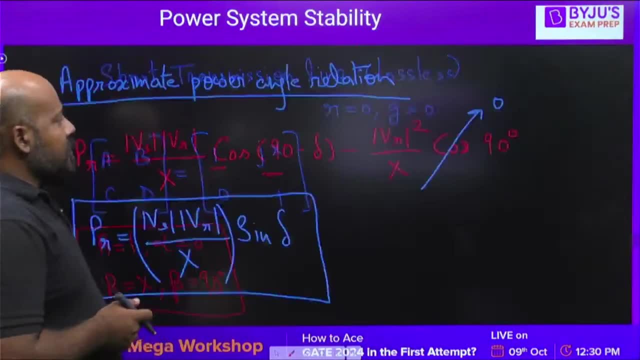 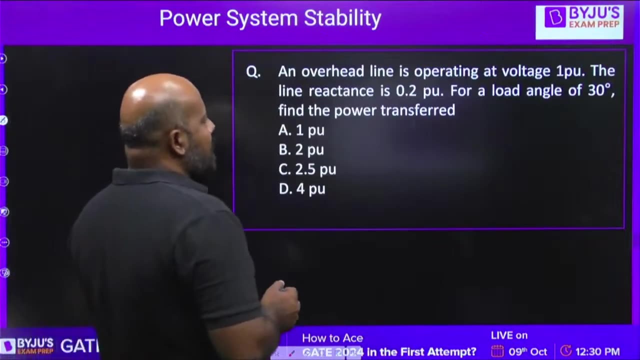 Any doubt you can ask me. Let us go to the next question. An overhead line is operating at a voltage 1 per unit. The line reactance is 0.2.. For a load angle of 30 degree, find the power transferred. 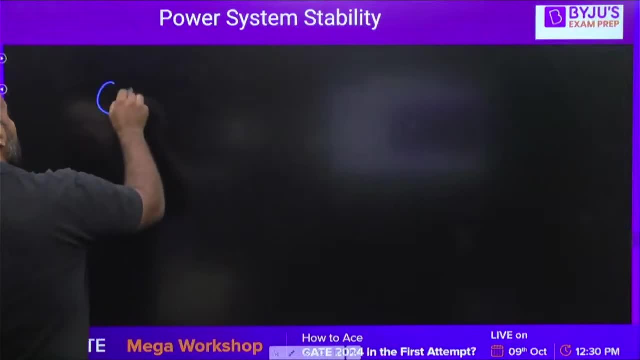 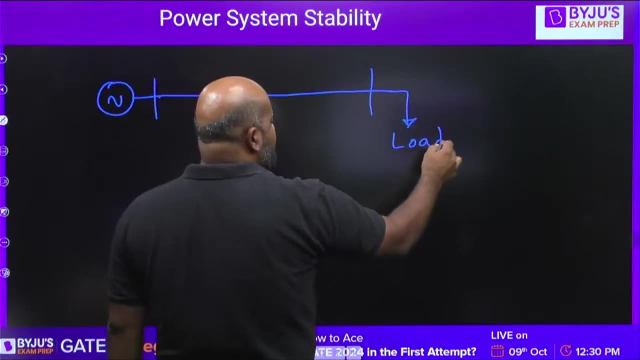 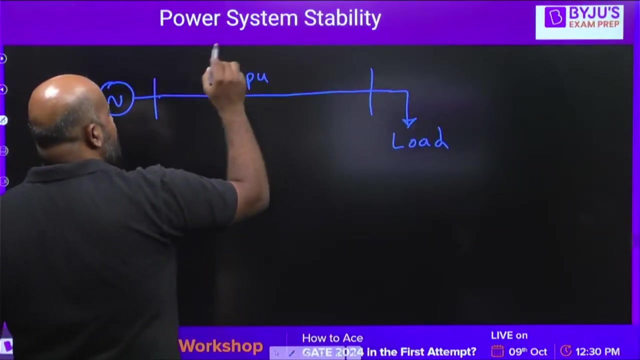 The situation is something like this: This is a generator, this is a generator side and this is the load side. He is saying: overhead line is operating at voltage 1 per unit, So it is operating at voltage 1 per unit. It is operating at 1 per unit voltage. 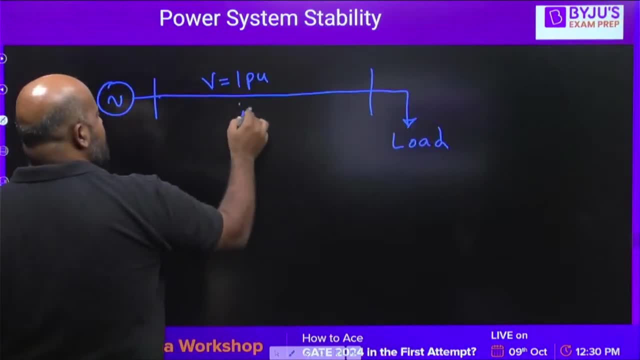 He is saying the line reactance is 0.2.. Line reactance is 0.2 per unit And he is saying: for a load angle of 30 degree, find the power transferred. Suppose this is going to be Vs angle, 30 degree, because del angle is given as 30 degree. 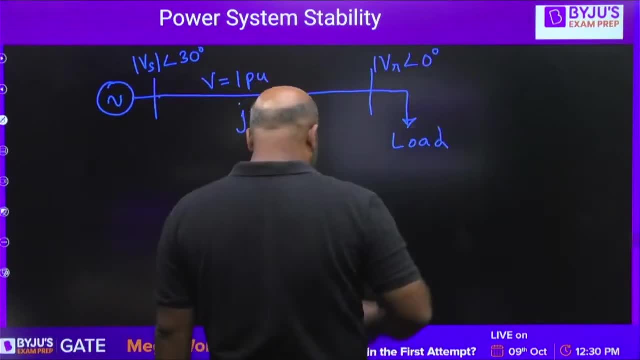 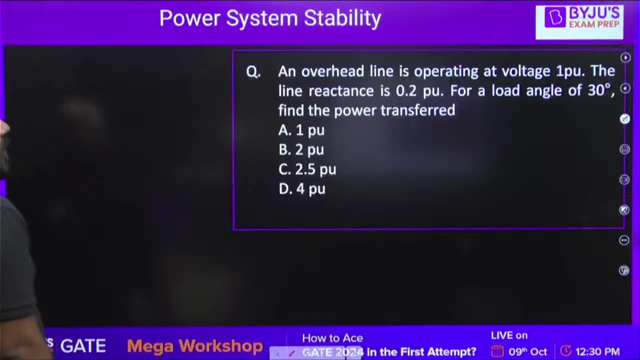 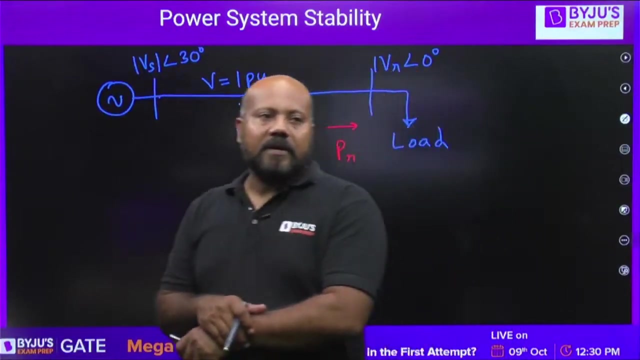 And suppose this is Vr angle 0 degree. He is asking: What is the power transferred? He is interested in the real power. He is interested in the real power. Now, please try to understand in this question. Yes, Vishwanathan, listen, listen. 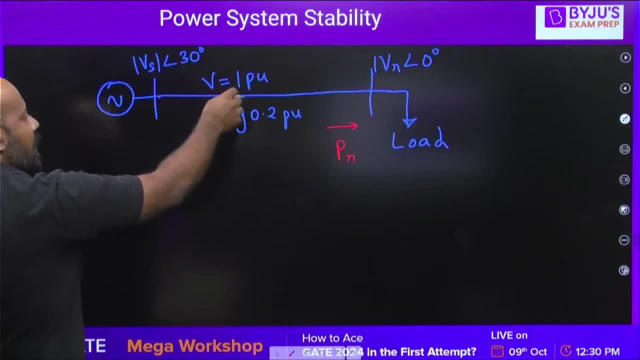 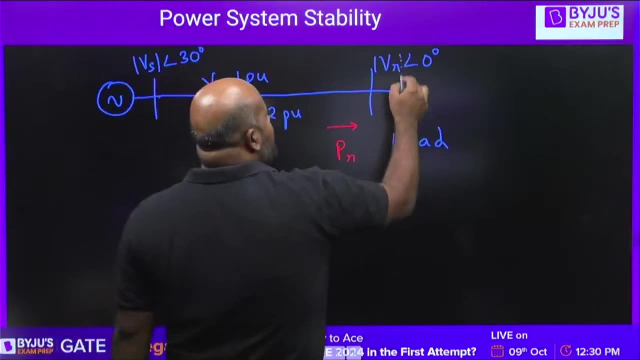 In this question he is giving you the operating voltage of the line, but he is not giving you the values, magnitude of the voltages for the sending end and the receiving end. So how you are going to solve this question? Because the real power received. 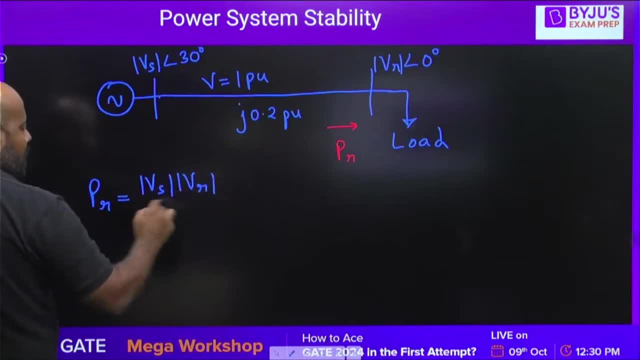 Is going to be mod Vs, mod Vr upon x, And this is sine del, and sine del is going to be sine 30, because del is given as 30. But we do not know the values of Vs and Vr. Now please try to understand. 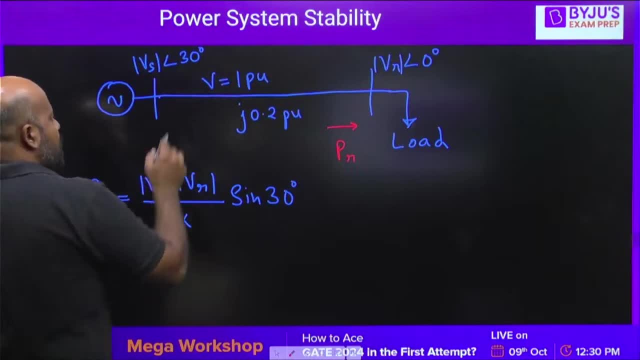 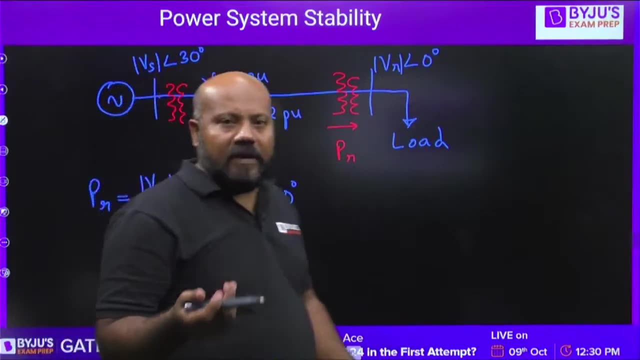 When you are saying the operating voltage of the line is 1 per unit and suppose there are two transformers are also there. Let us make it more general, Otherwise it is going to be very simple, direct. Let us take two transformers, also One at the generating end. 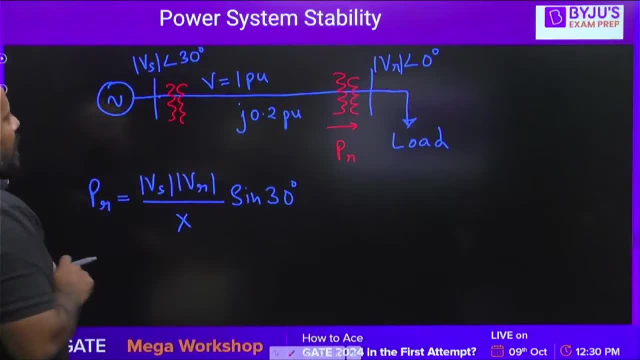 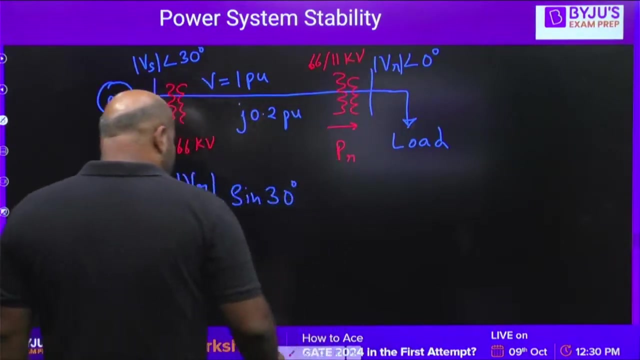 One at the sending end, One at the sending end and one at the receiving end. Now suppose if the voltage here is 11 kilovolt and here the voltage is 66 kilovolt. And suppose here we are taking it 66 kilovolt and here it is 11 kilovolt. 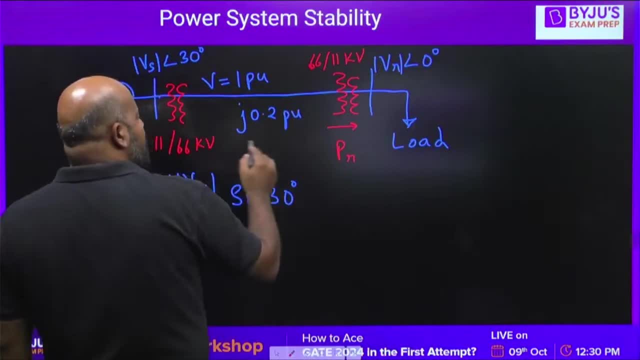 And you are saying, sir, the transmission line is going to be operating at 66 kilovolt, Yes or no? If this transformer is saying 11 of the 66, this is saying 66 of the 11.. So this line is must be operating at 66 kilovolt. 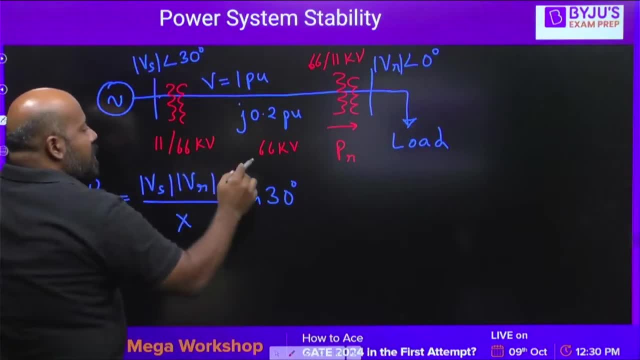 Now in the question you are saying the operating voltage of the line is 1 per unit. It means the actual voltage is 66. Then only you are getting 1 per unit. It means if the line is operating at 66 kilovolt, what about the generator side? 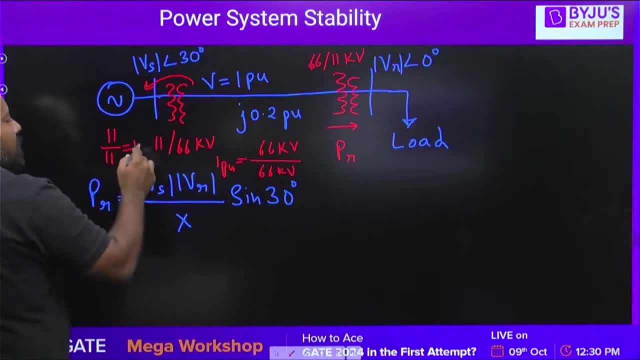 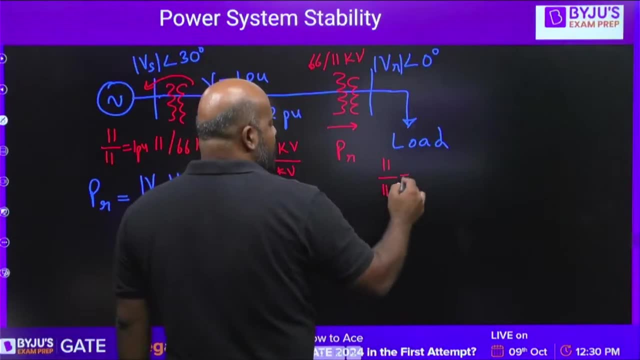 Now, generator will be operating at 11 kilovolt, So this is also 1 per unit, And the load side also, it is operating at 11 kilovolt, So this is also 1 per unit. What I wanted to tell you: if the operating voltage of the line is given as 1 per unit, 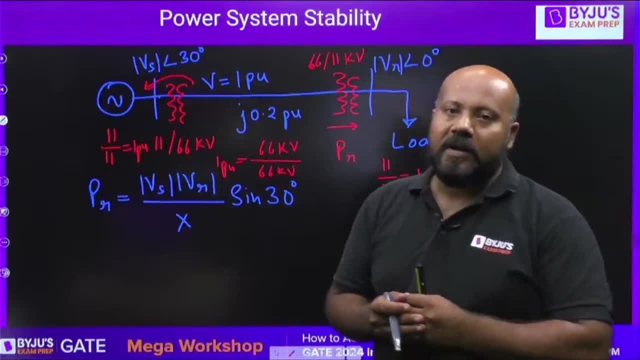 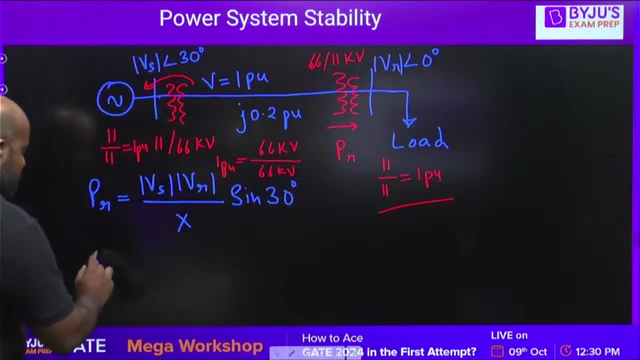 then you can take both the sending and voltage and the receiving and voltage as 1 per unit in magnitude. Is it clear? everybody Just put the values. So this is going to be 1 into 1.. What is the x value? It is 0.2. 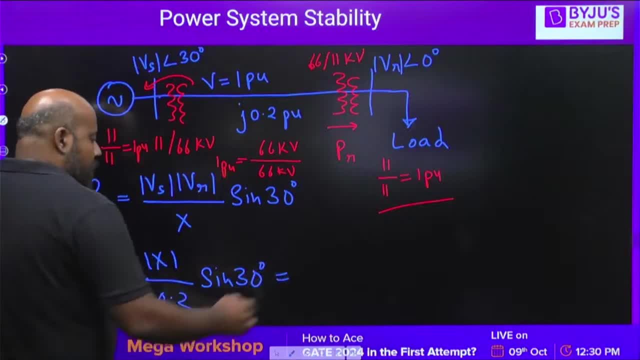 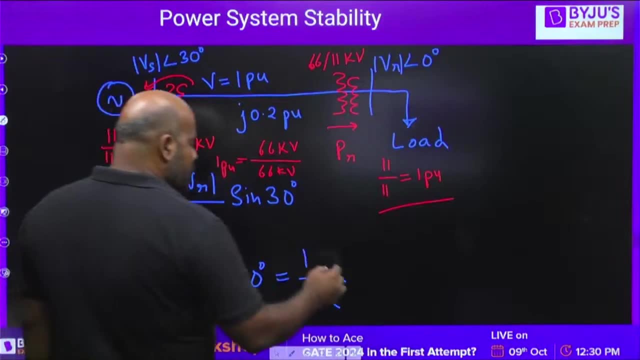 And this is sine 30. It is going to be 1 upon, or simply it is going to be 0.2.. 1 upon 0.2.. What is sine 30? Sine 30 is going to be 1 by 2.. 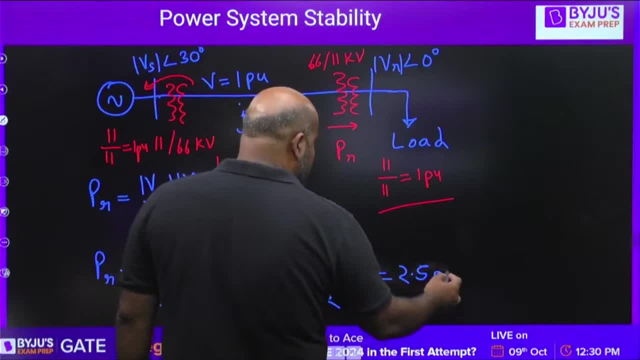 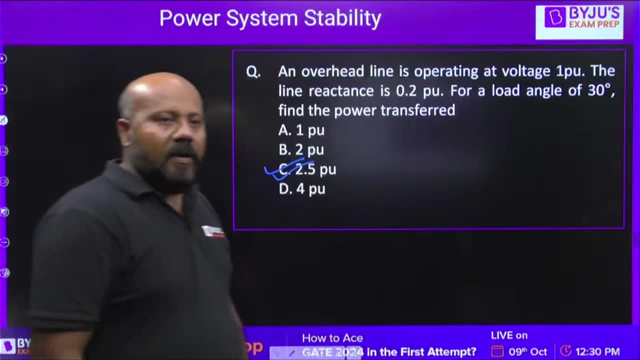 This is going to be 10.. This is going to be 2.5 per unit. So what is the correct answer? Correct answer is going to be C, 2.5 per unit. Only one candidate is answering, no problem. 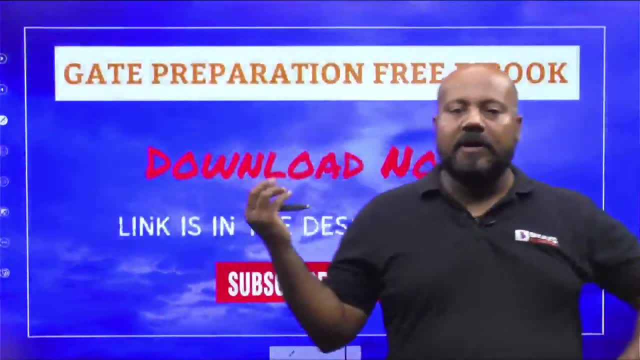 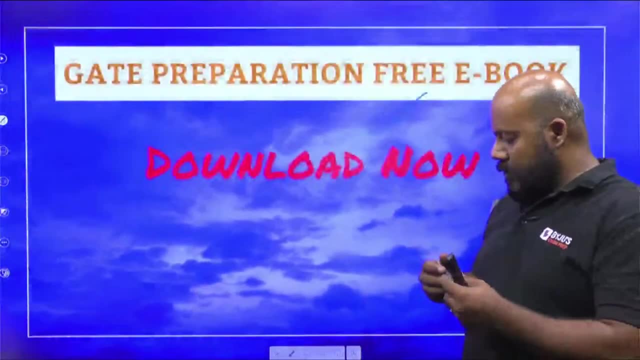 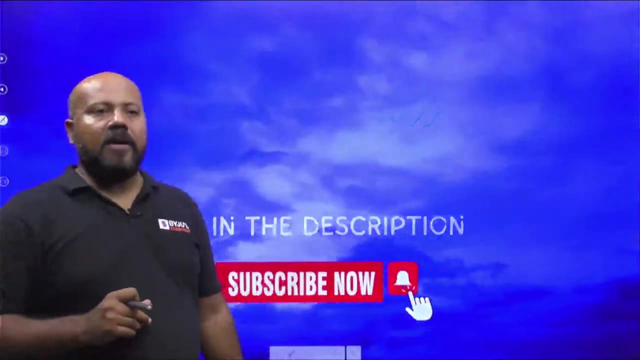 Now please try to follow this description link. If you want free e-books, Okay. If you want the soft copy of, if you want the soft copy of e-books, then you can follow the download link which is given in the description of this video. 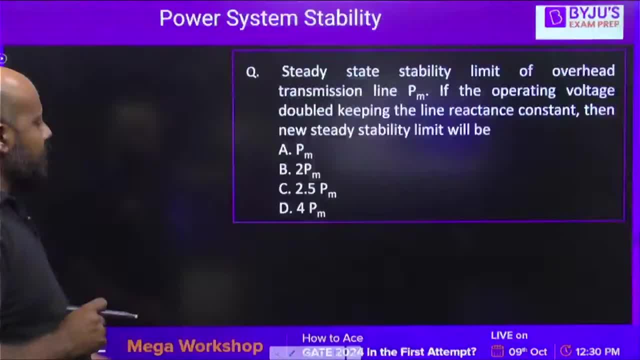 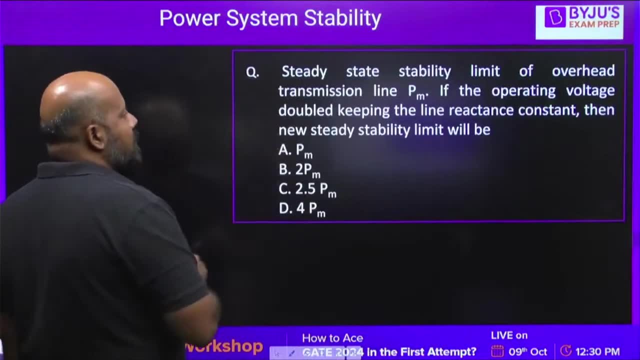 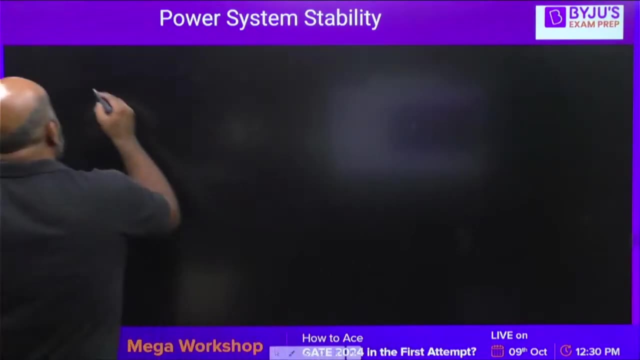 And you can enjoy those session, those books. Let us do the next question. Steady state stability limit of overhead transmission line is Pm. What is a steady state stability limit? Let us try to understand Steady Stability Limit. 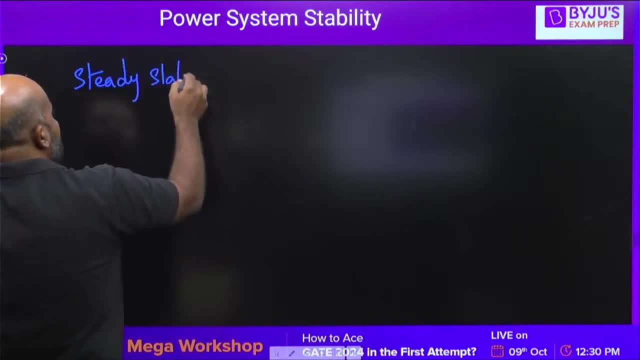 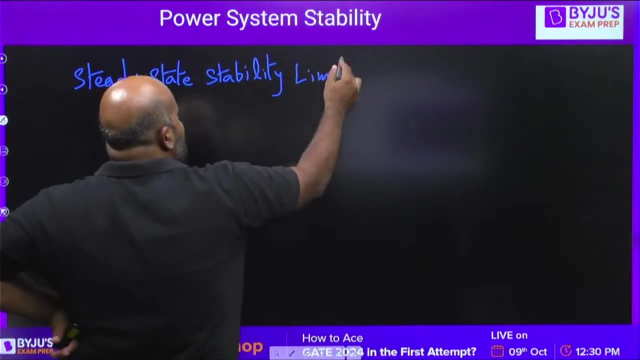 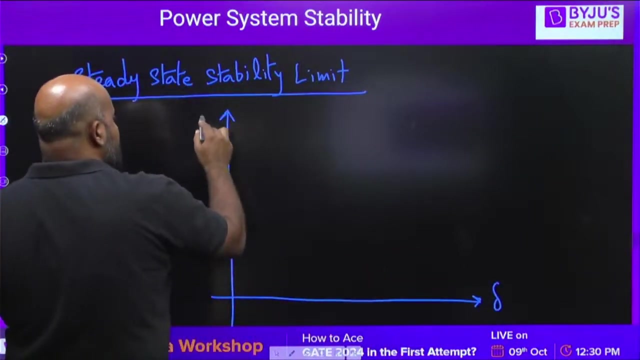 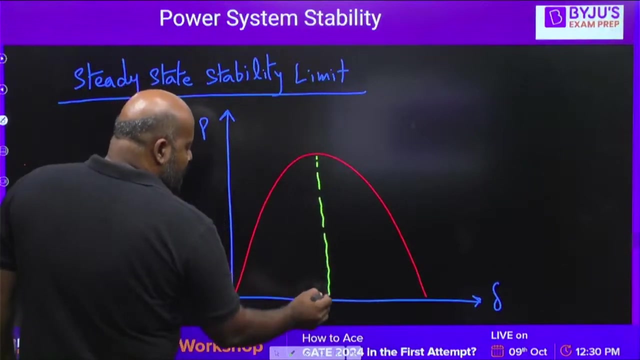 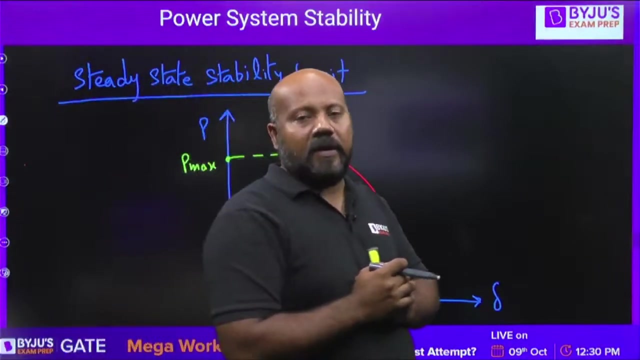 A state, a stability limit, How it is defined. This is del, This is P. Yes, All right. Okay, You get the maximum power at del is equal to 90. Now this P max we are defining as the steady state stability limit, because this is the maximum power which you can transmit. 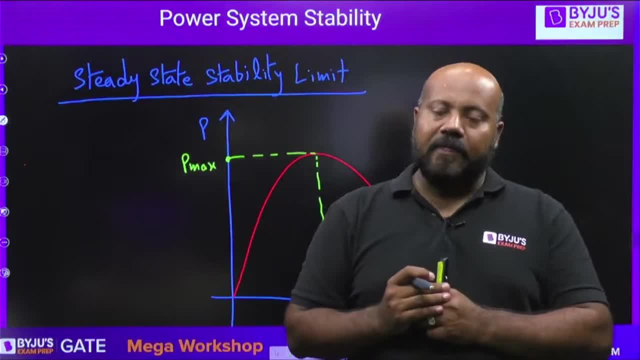 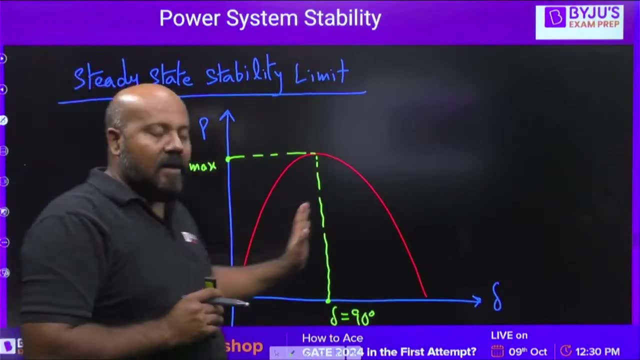 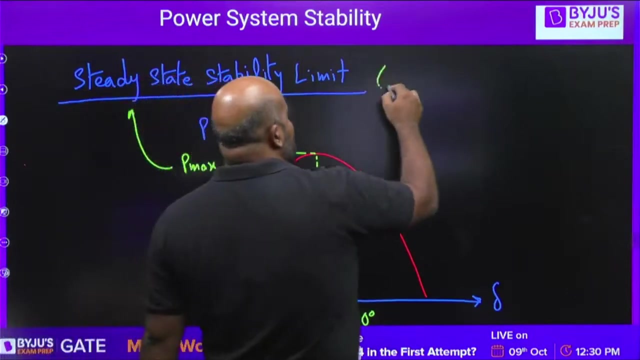 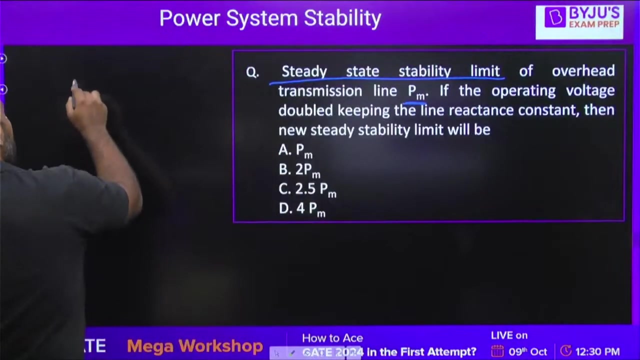 without losing your system stability At any point of time. if you want to transfer more than this power, then you will be falling in the unstable region. So this P max we are defining as steady state stability limit. So in the question he is saying this P max. 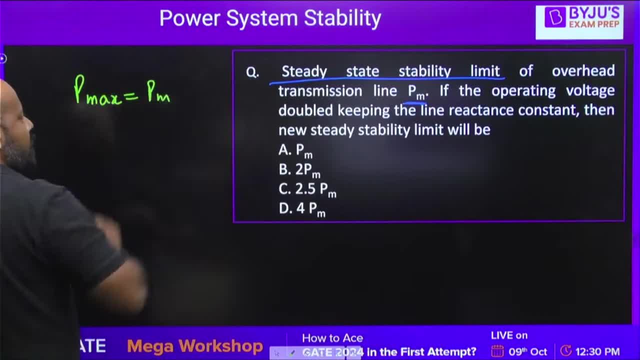 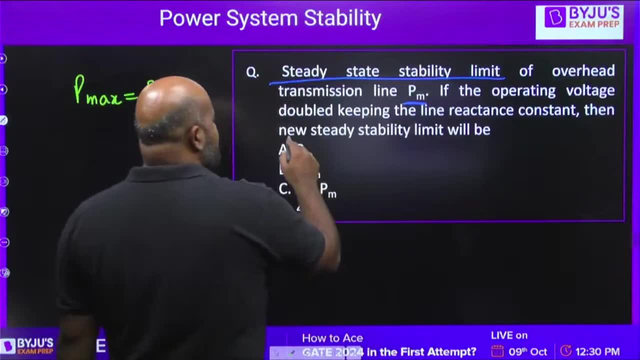 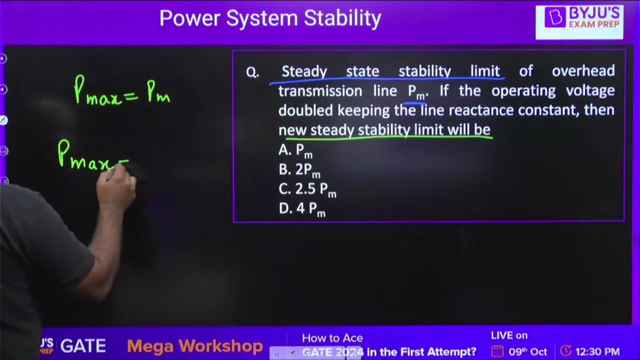 is given as P m. He is saying: if the operating voltage is doubled, keeping the line reactance constant, then what is the new steady state, stability, Stability limit? you must be knowing that P max you are defining as mod, Vs, mod Vr on X, because sine del is 1, del is 90 degree, yes or no? Now suppose we are assuming Vs and 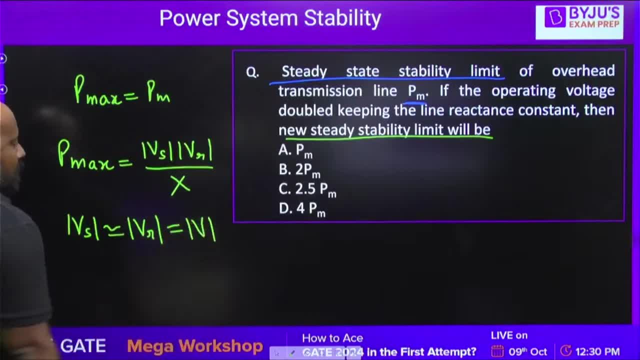 Vr. they are approximately equal and they are equal to mod V. So can I write that P max is directly proportional to the square of the voltage? Yes, Why? Because this X is given as constant. This X is constant Now, if you do the relation. 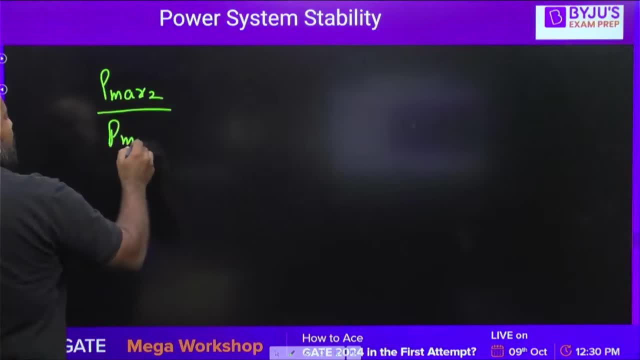 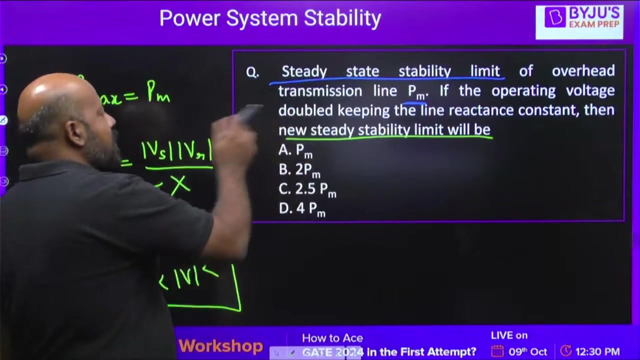 P max 2 upon P max 1. this is mod V2 upon mod V1. this is a square. If you put the values he is saying, the operating voltage is doubled. It means V2 is equal to mod V1.. This is a. 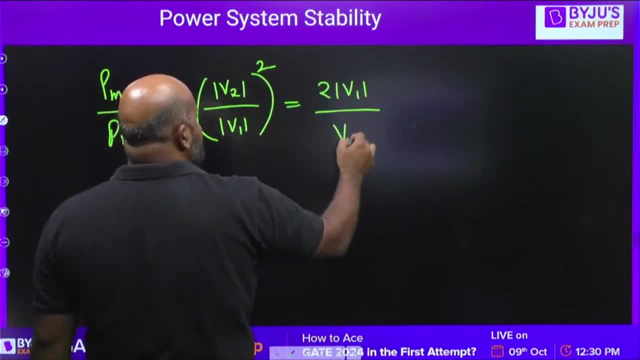 double. So if you put the values he is saying, the operating voltage is doubled. It means 2 has become 2 times v 1 and this is also v 1. this is holy square. so v 1, v 1 cancelled and you will. 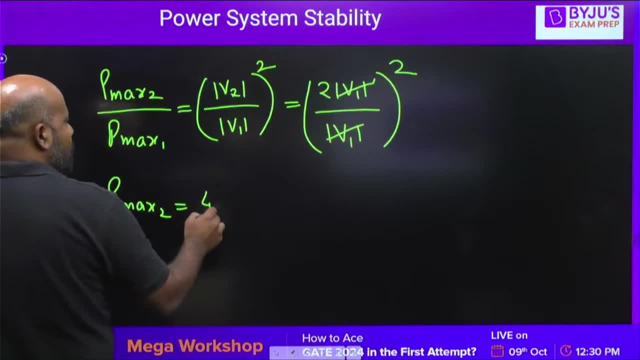 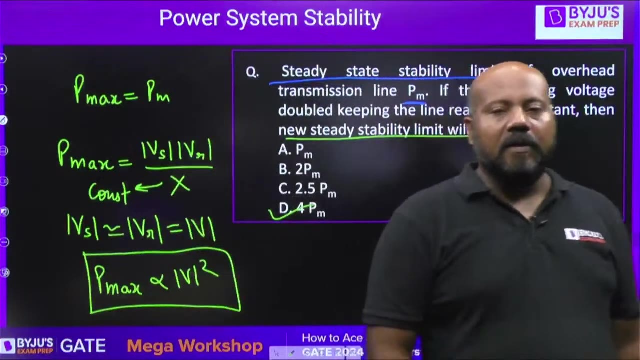 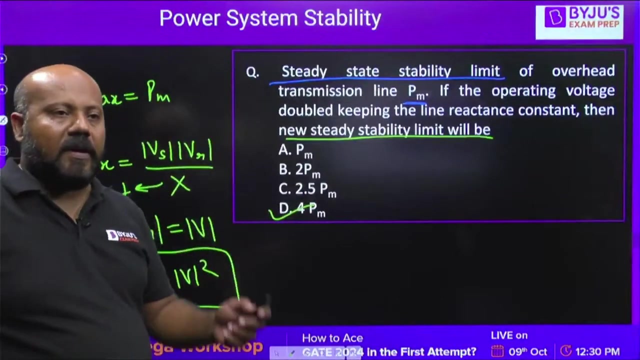 get p max 2 as 4 times p max 1. i hope it is clear for everyone. so what is the correct answer? d, it is 4 pm. everybody. just tell me. are you able to follow this just comment? are you able to follow this or not? if you have any doubt, you can ask me. see the next question, the steady state stability. 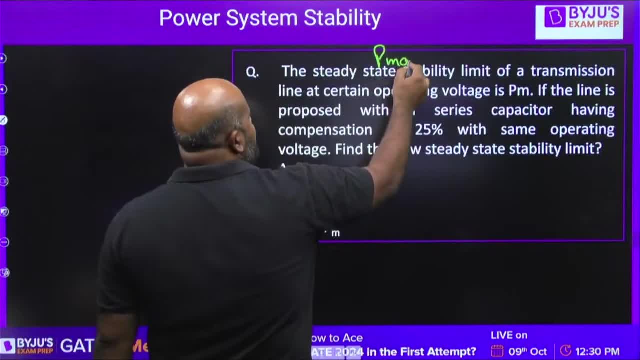 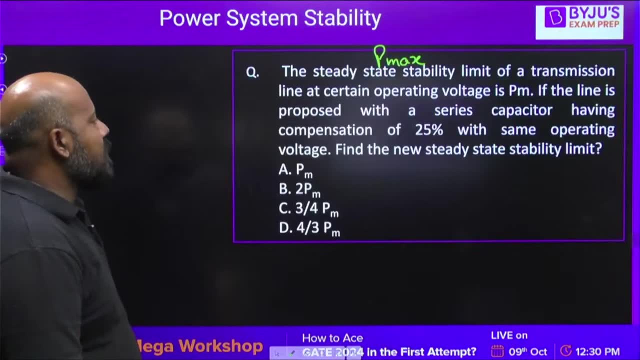 limit. again, that is nothing but the p max. p max value is saying at a certain operating voltage it is pm. if the line proposed with a series capacitor having a compensation of 25 percent with the same operating voltage voltage, it means now the voltage is constant but because of the series capacitor compensation, what is happening? there is 25. 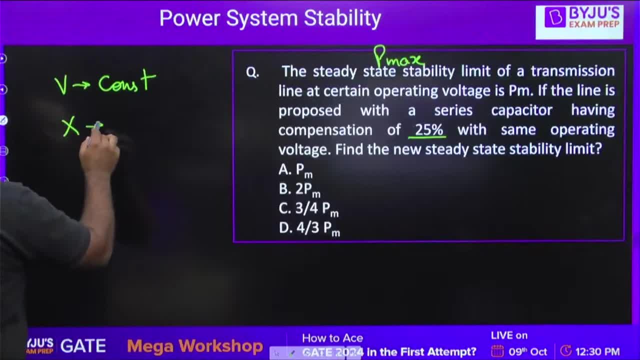 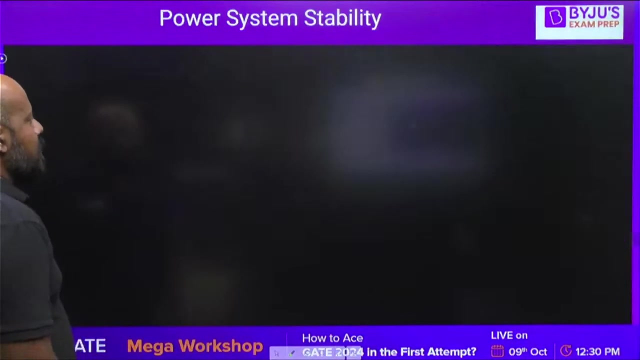 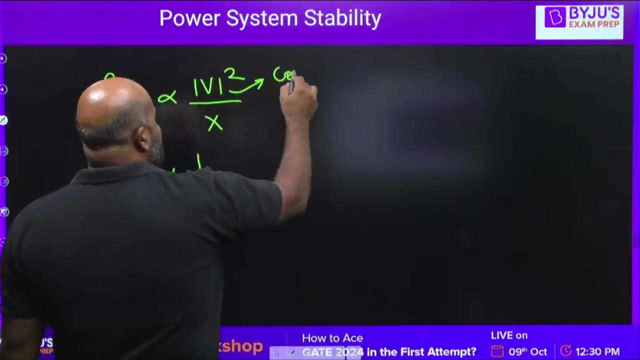 compensation. it means if this is the x initially, then after compensation, because 25 is compensated. so what is the remaining one? the remaining one is 0.75, 0.75 of this capsule and then, up to tim, a given voltage, max or p of someone in. you can say p, max, capital, point x, because the guarantee of t is γ, that's. 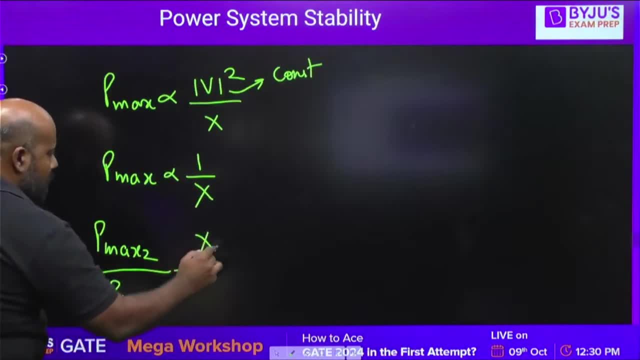 free and you know it is stable and the mark- expectancy: this: now you know that p max is directly proportional to mod v squared upon x. or you can say p max is inversely proportional to x. why? because voltage magnitude is constant this time. so you can write p max 2 on p max 1, is x2 upon x 1. there are two models on the boundary and a big deal is in the underlying set. is there? it was такую c16, couponsome Nobel economic. 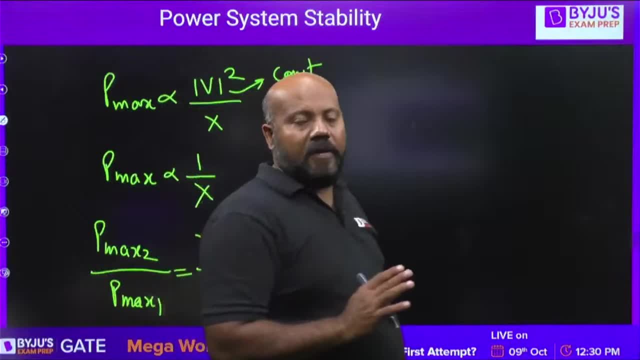 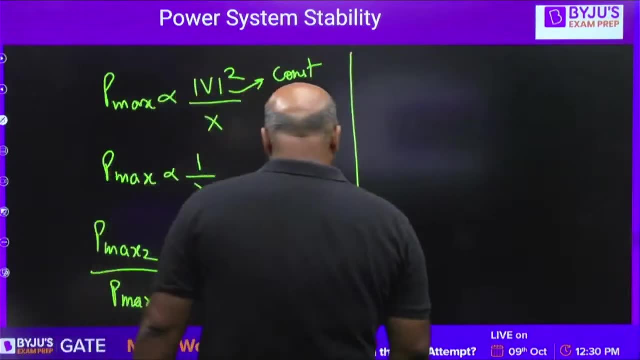 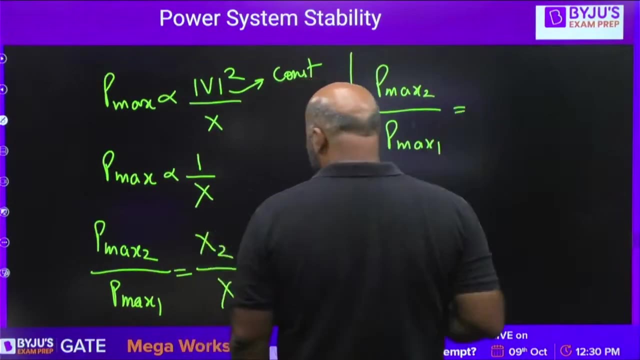 that is the x in the first case, without compensation, and x2 is x in the second case with 25 series capacitive compensation. so if you put the values p max 2 upon p max 1, x2 is 0.75 x and x1 is simply x. so if you relate, it x cancelled, so you can write p. 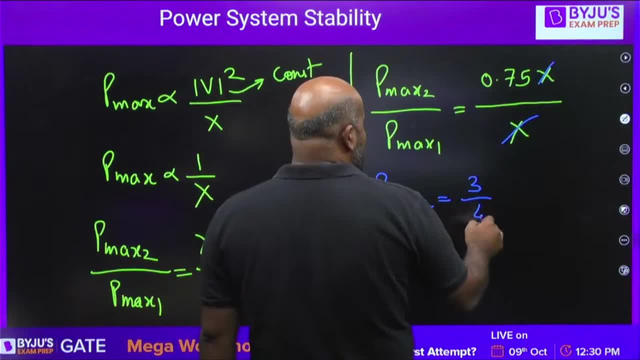 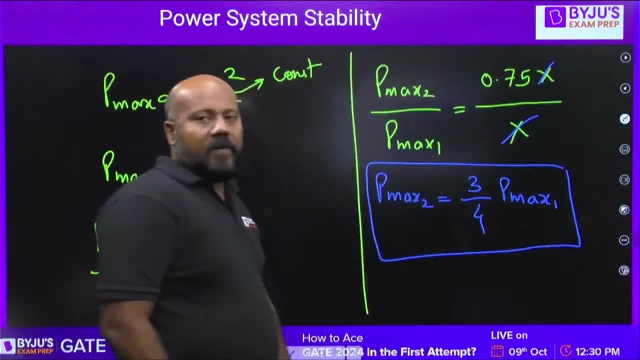 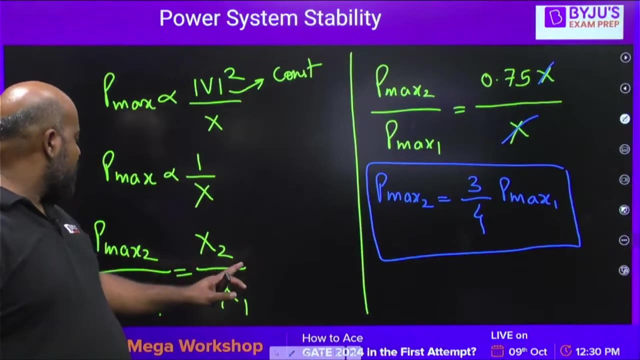 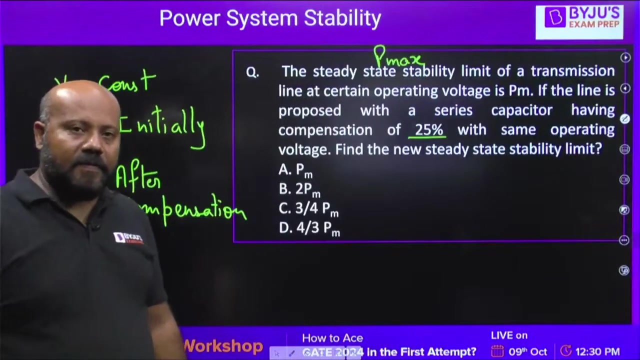 max 2 is 3 by 4 and this is p max 1. is it clear? everybody wish not. is there any doubt? i am doing it correctly now. p max 2 upon p max 1. is it clear why you are writing 4 by 3 pm? 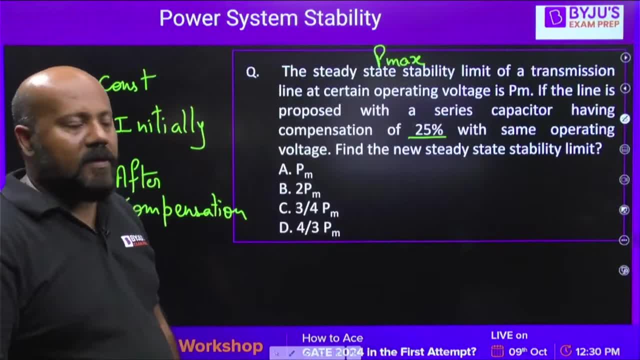 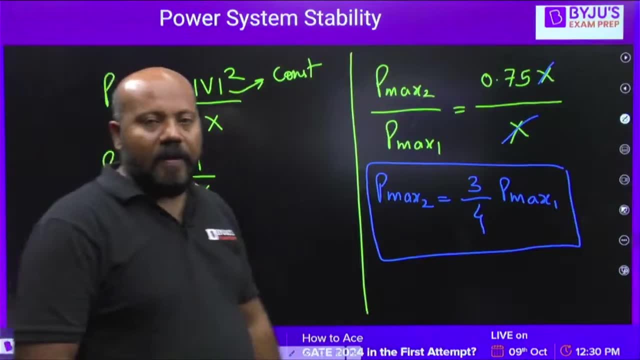 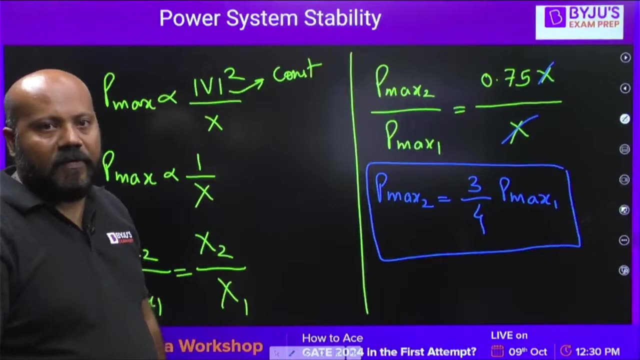 yes, there is the inverse relation. p max is inversely proportional to x. are you getting that? so you are getting 0.75. 0.75 is nothing but 3 by 4, not 4 by 3. 4 by 3 will become a different thing. 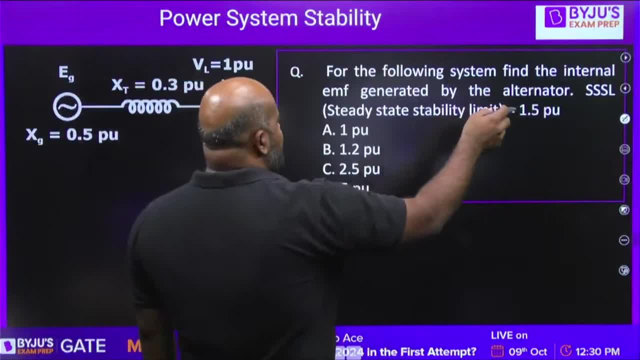 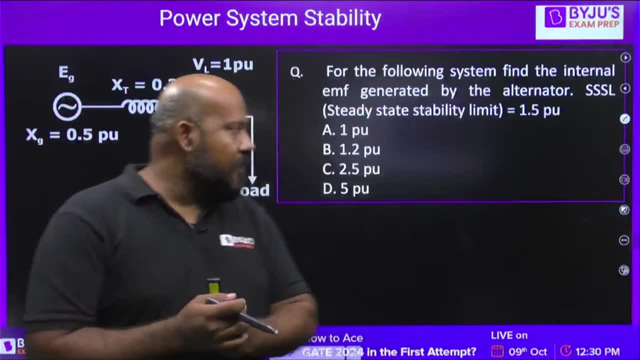 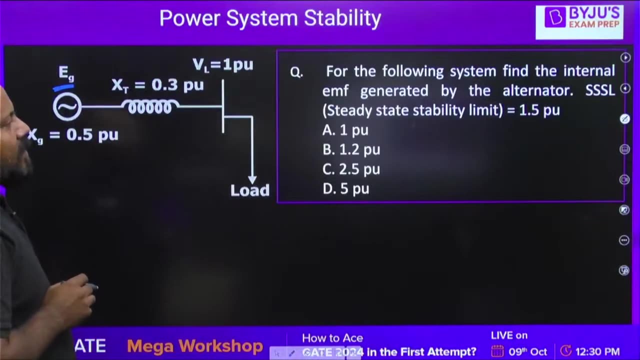 see the next question for the following system: find the internal emf generated internally. emf generated is the excited excitation emf of the synchronous generator. so basically he is asking you this: eg value. the steady state stability limit is given as 1.5 per unit. now please try to understand. he is giving you p max. that is steady state. 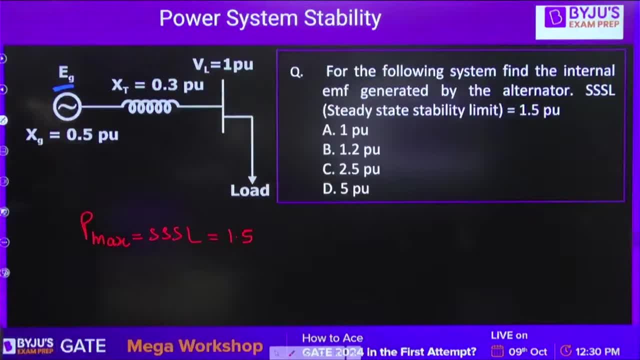 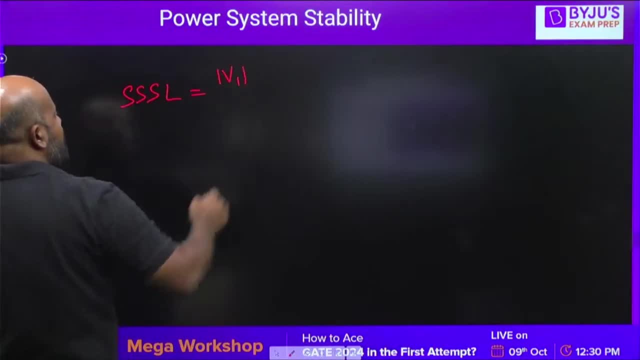 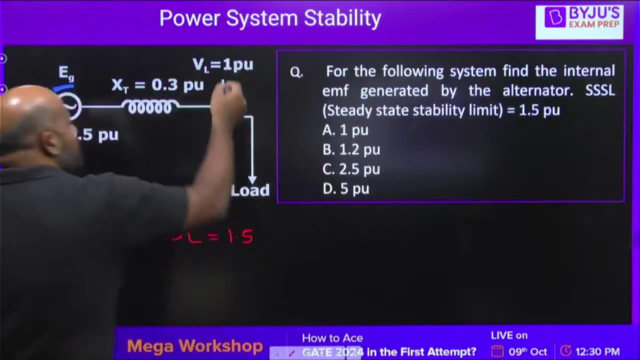 stability limit as 1.5. and what is this steady state stability limit? a steady state stability, it is mod V1. okay, it is given in excitation emf, so this is excitation emf, terminal voltage, load side. so this is VL. in between these two points, what is the total series reactance? 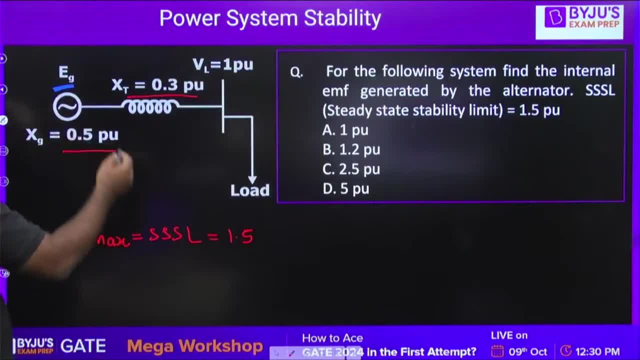 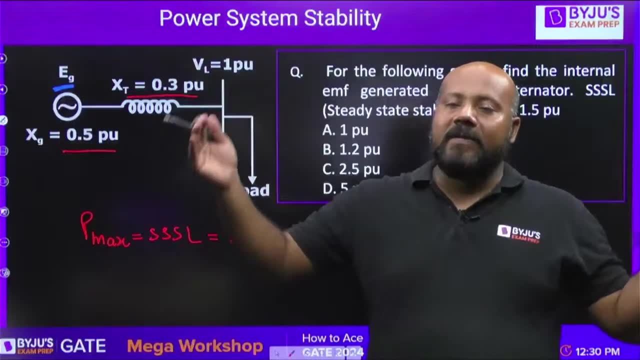 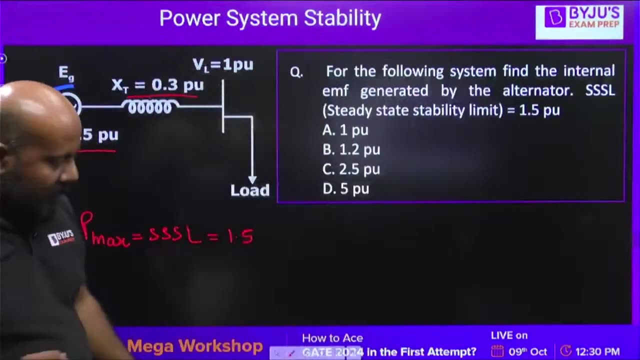 that is 0.3 plus 0.5, because generator reactance will also add up. because generator reactance will also add up. now you have to find that total effective series reactance between the sending in and receiving it. that is what you have to write in place of X. so this is 0.3. 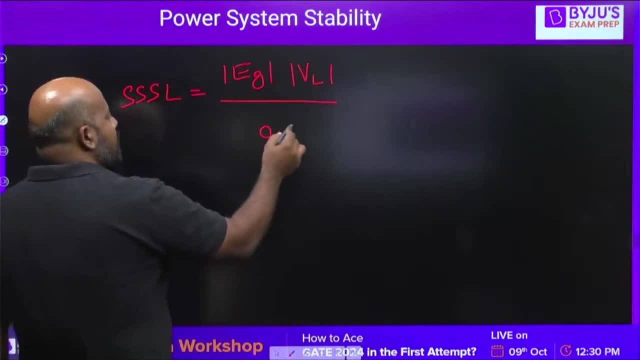 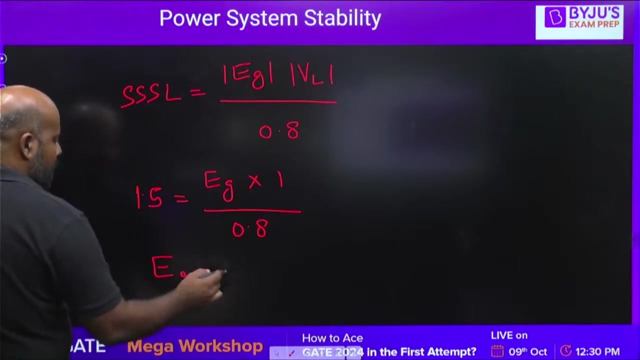 plus 0.5, that is 0.8. it is 0.8. it is given as 1.5. this is EG. what is this VL? this VL is given as 1 per unit in magnitude, so if you write it, you will get the generator emf. 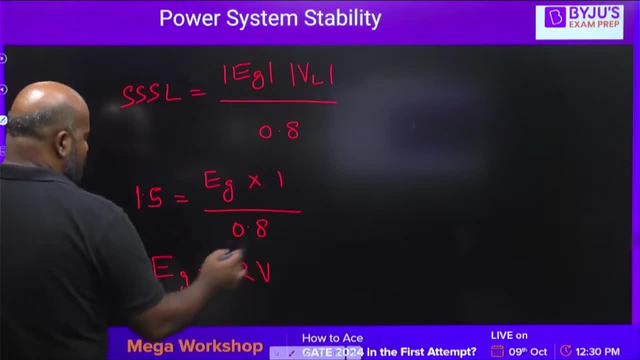 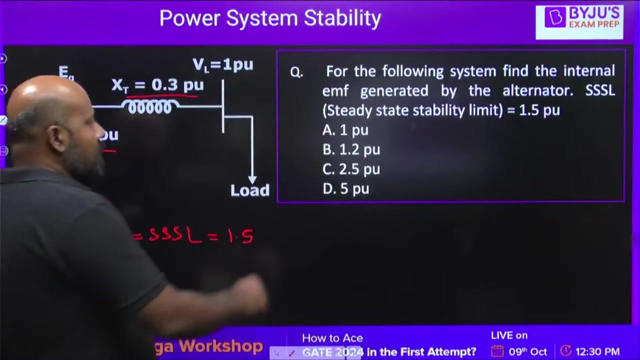 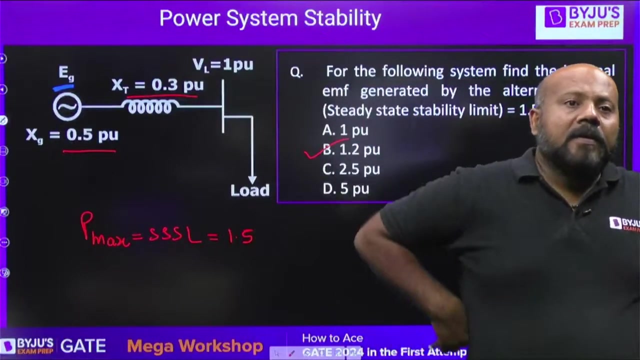 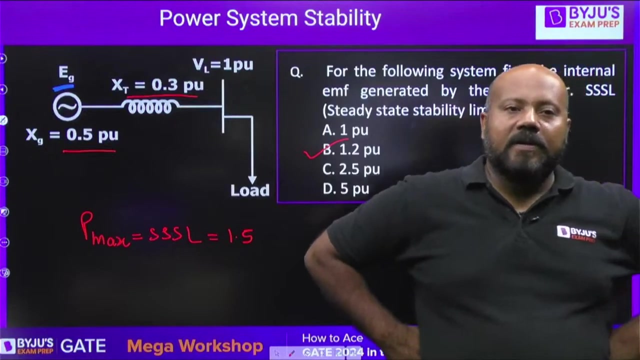 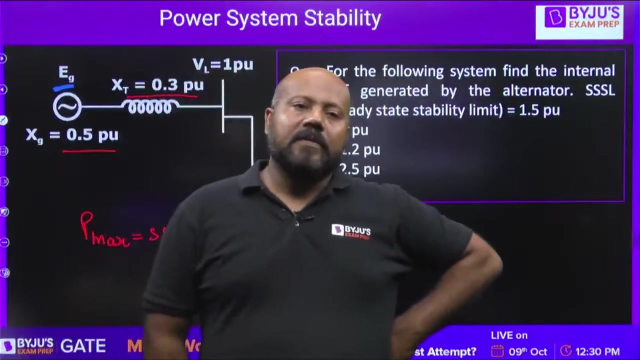 as 12 volts. sorry it is. I think it is 1.2, yes or no? yes or no, I am not sure about it. ok, I think it is some of the streams. ok, some of the papers: MSC candidates are eligible. you please check it ok. 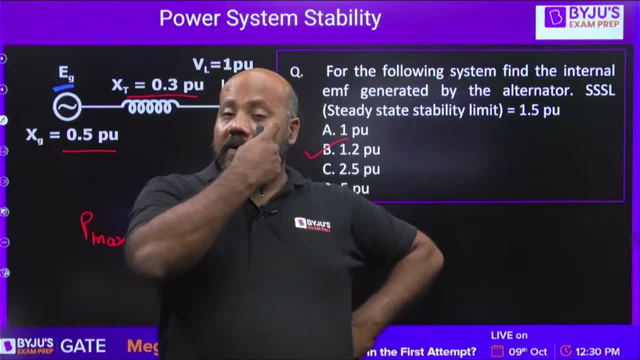 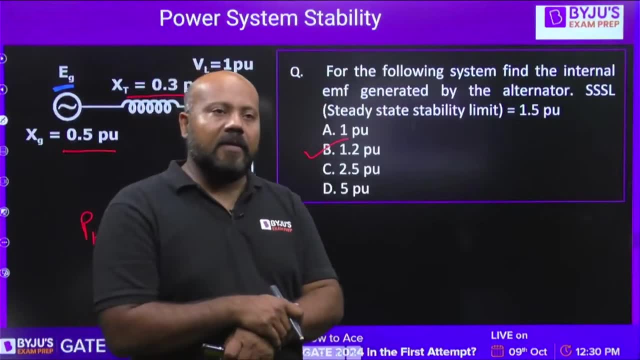 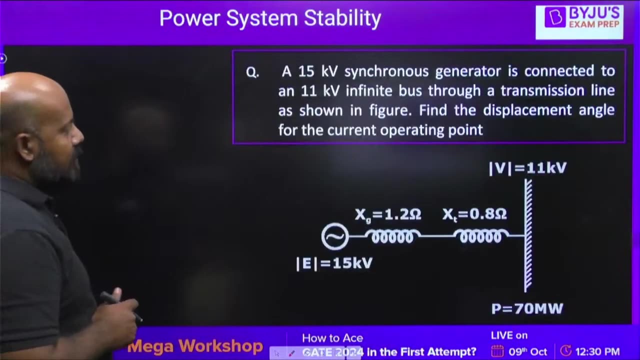 I have to see it. so what you can do is you just drop a message on my personal telegram channel and tonight itself I will just check and revert back to you, because I cannot give you the wrong answer now. is it clear? everybody see the next question: a 15 kilo volt synchronous generator. 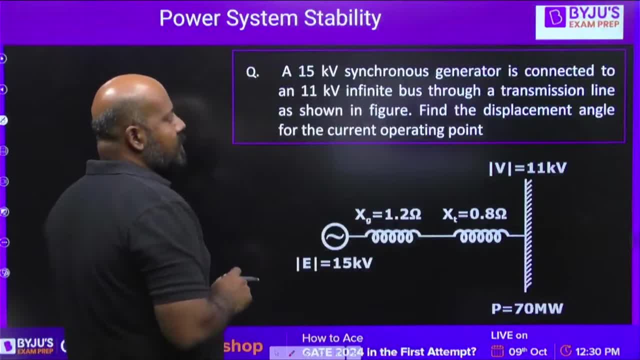 is connected to 11 kilo volt infinite bus through a transmission line as shown in the figure. find the displacement angle for the current operating condition. excitation. EMF magnitude is given, infinite bus terminal voltage is given, but the del angle is not mentioned. that is what he is asking. 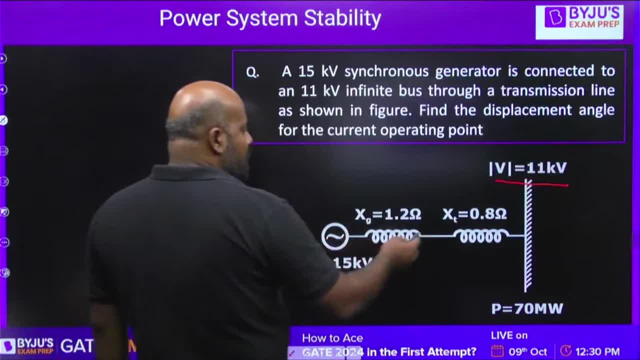 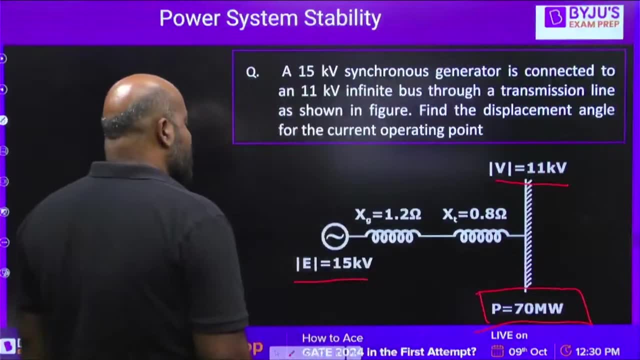 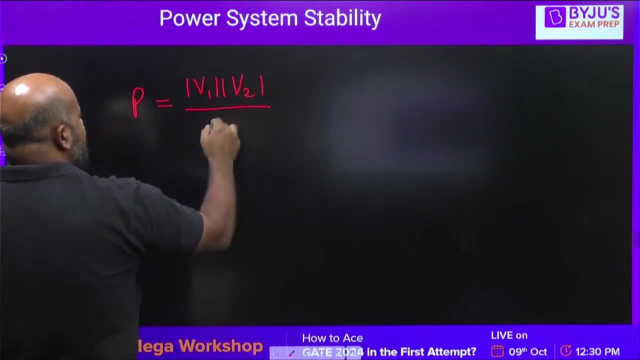 the generator reactance is given, the line reactance is given and the total real power received at the infinite bus is also given. so you can directly write it: P is equal to mod V1, mod V2 upon X. this is sine del. what is P? it is given as 70 megawatt. 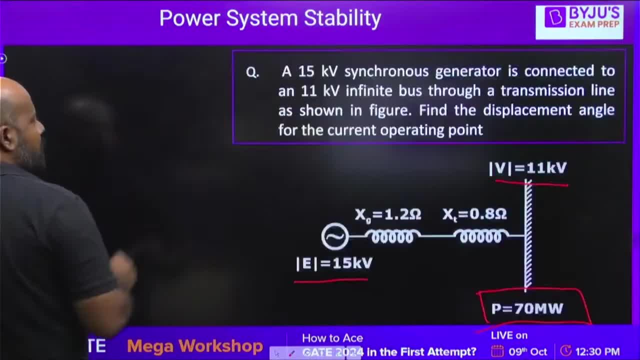 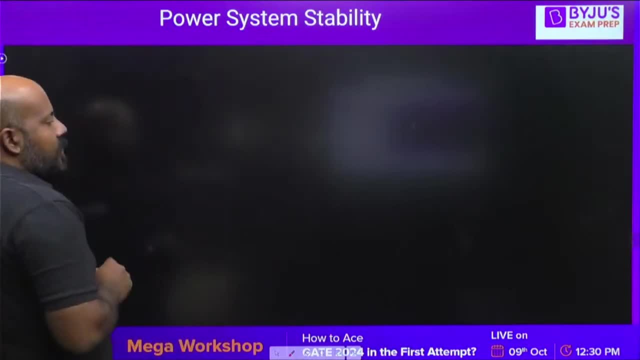 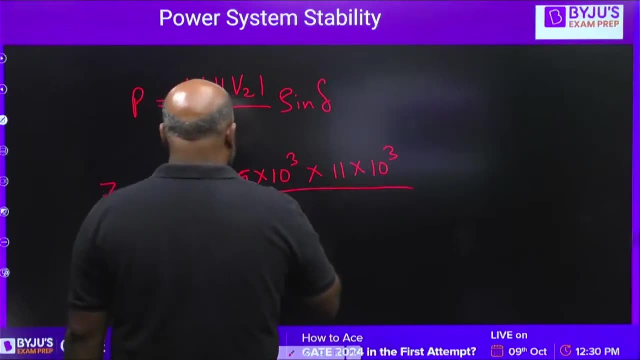 what is V1? it is 15 kilo volt. what is V2? V2 is 11 kilo volt divided by X. what is X? X is going to be 1.2 plus 0.8, because you have to add up to the. 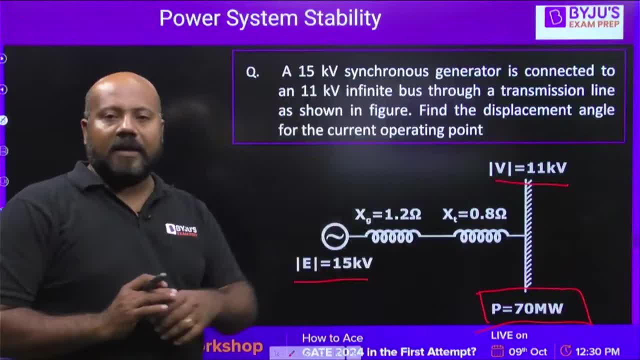 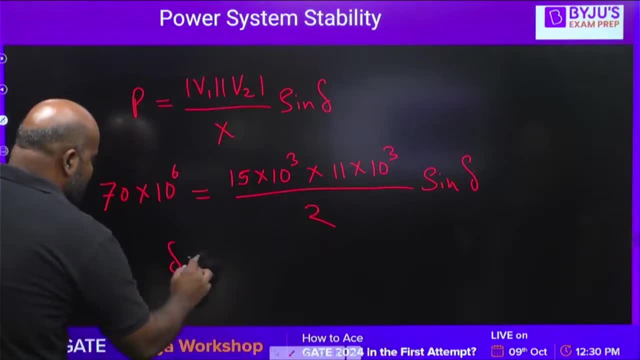 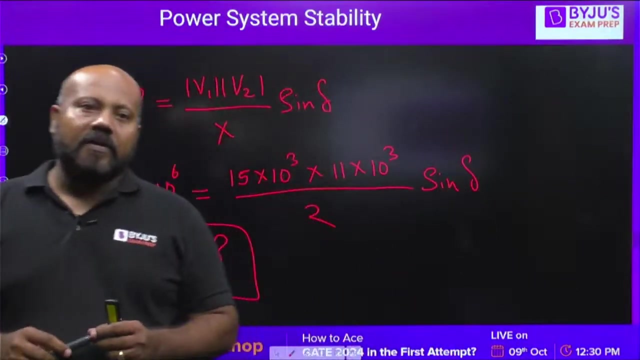 and you will be getting the value of 2 andlagen, that is, del. tell me, what value are you getting? so tell me, friends, what is the value? is del, what is the value? are you generating del? somewhere around 59, 59, yes, 58.047. 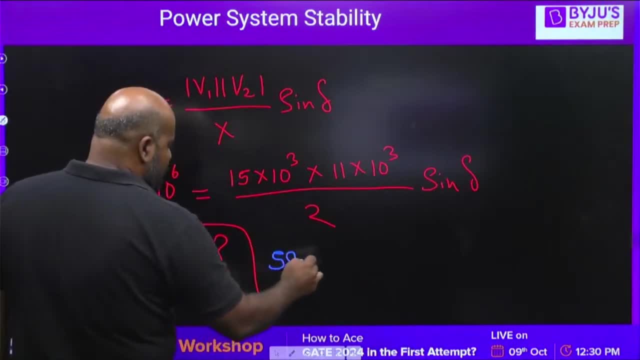 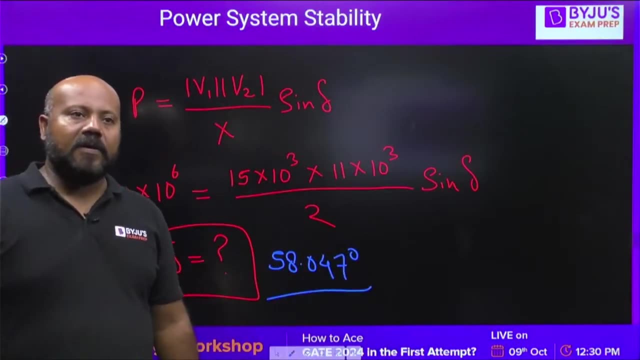 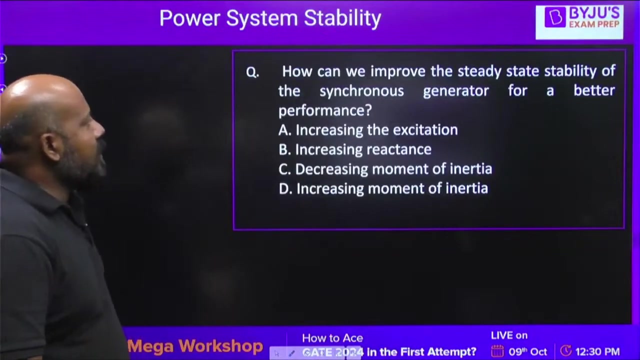 perfect, 58.047. everybody. please cross checking this value because don't have reference. i am from- just for just for following Murli's comment- the only candidate who is responding. Next question: how can we improve the steady state stability of the synchronous generator? 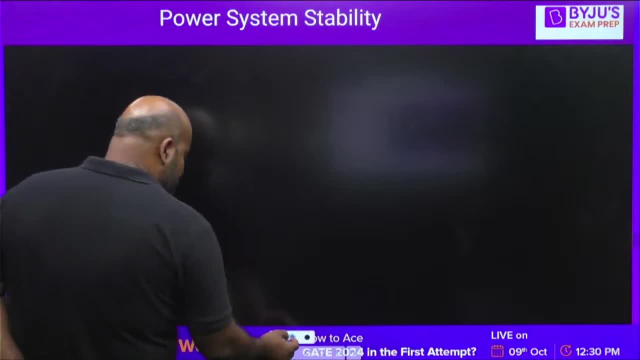 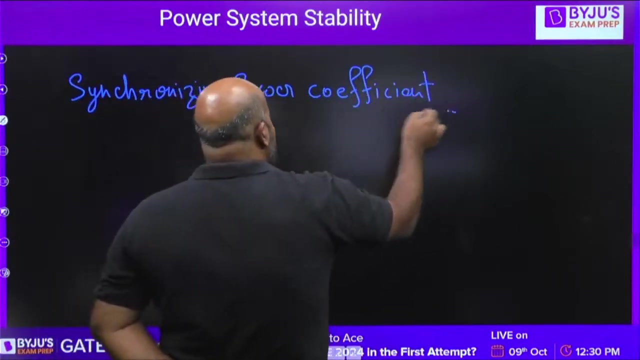 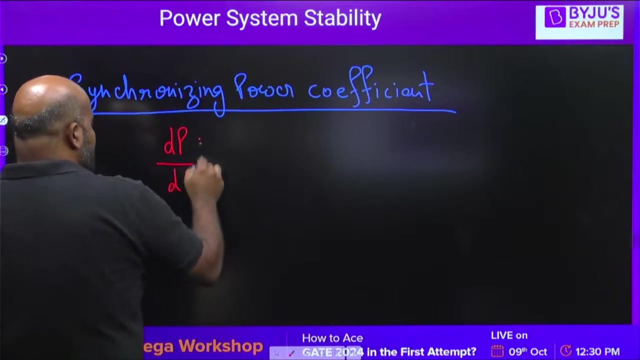 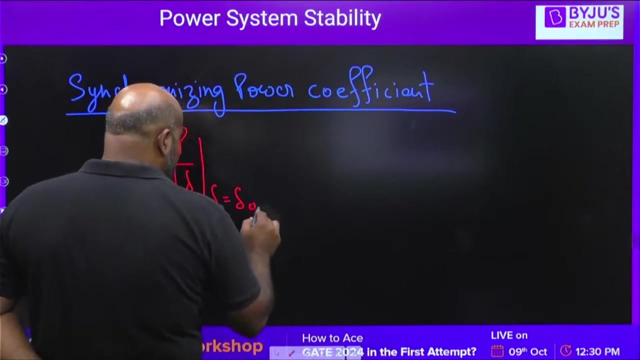 for a better performance. Now please try to understand Synchronizing power coefficient. synchronizing power coefficient: how we define synchronizing power coefficient? we are defining synchronizing power coefficient as dP by d del. at del is equal to del naught, yes or no. at del is equal to del naught. dP by d del. 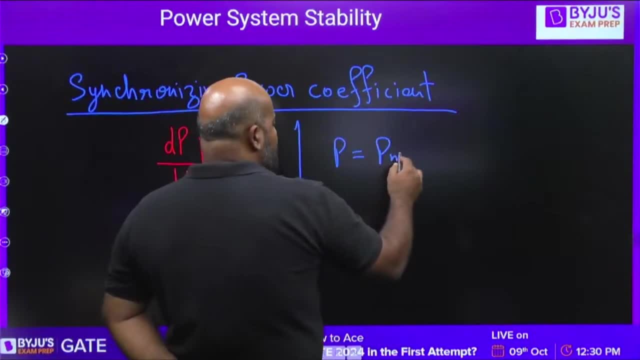 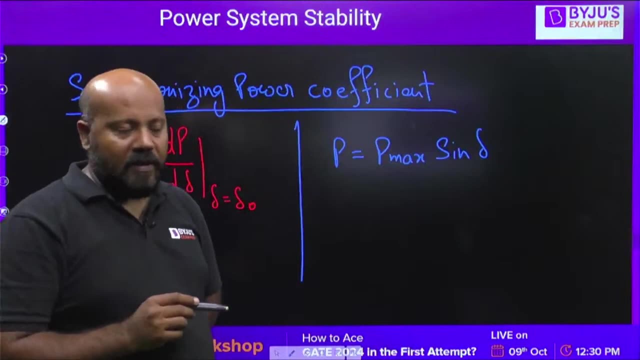 What is this? If you have P is equal, to suppose P max sin del. okay, I am writing this V1, V2 upon X as P max. Then what is going to be dP by d del? Just differentiate it. 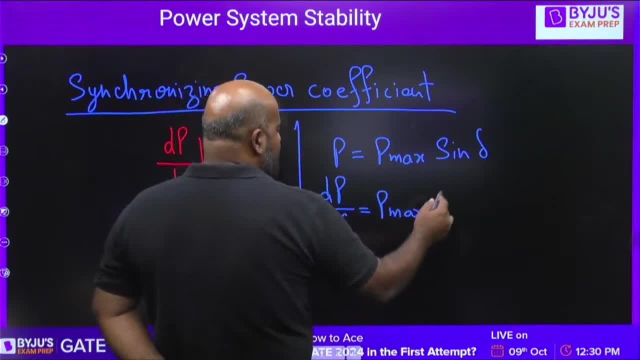 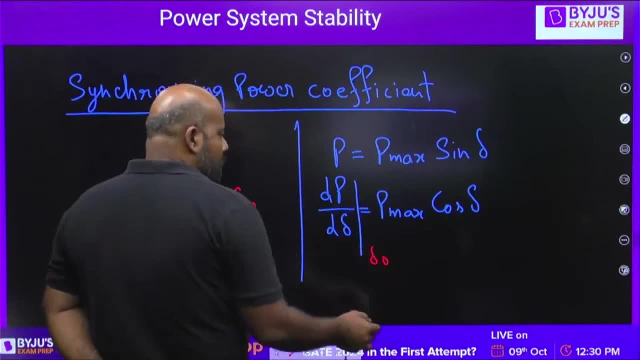 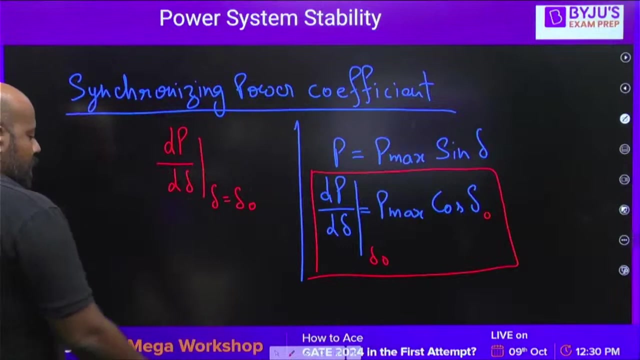 Just differentiate it with respect to the del angle, so it will become P max. This is cos del, And if you want to put del is equal to del naught, then you put del is equal to del naught. So this is going to be your synchronizing power coefficient. 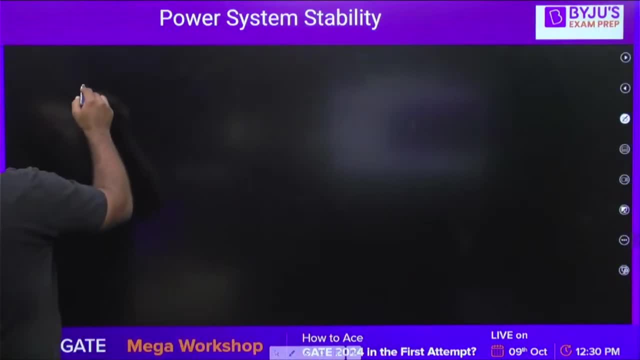 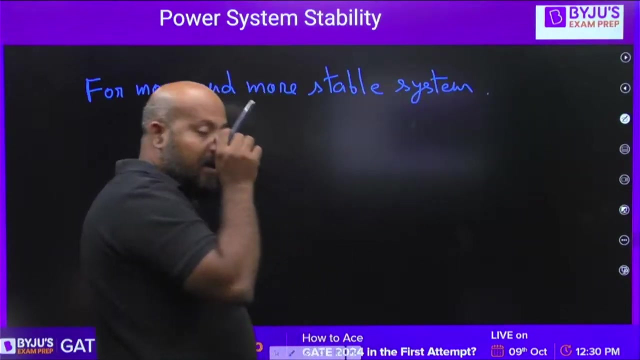 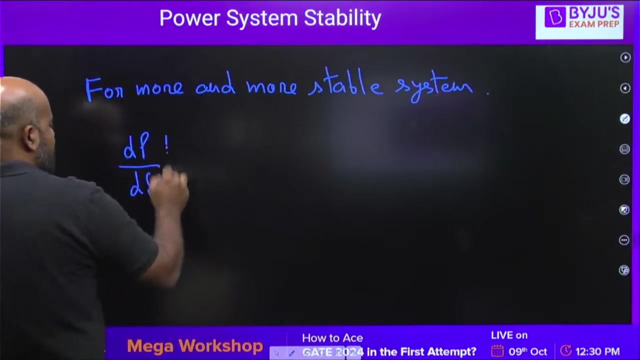 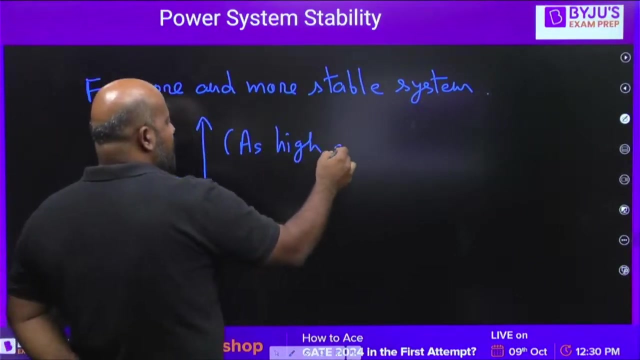 We are defining that for more and more stable power. Okay, For more and more stable system, and we are talking about steady state stability. for more and more stable system, the synchronizing power coefficient should be as high as possible, As high as possible. 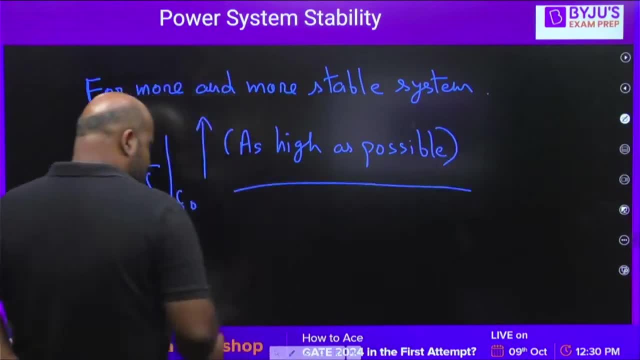 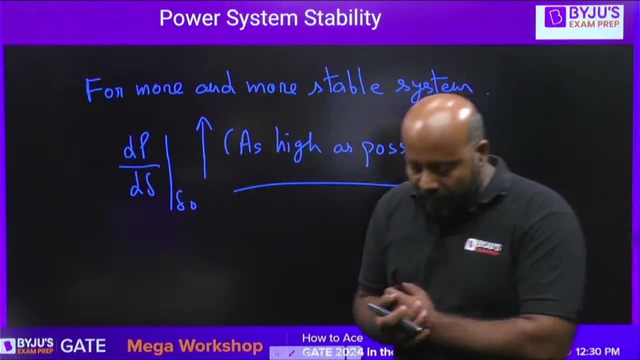 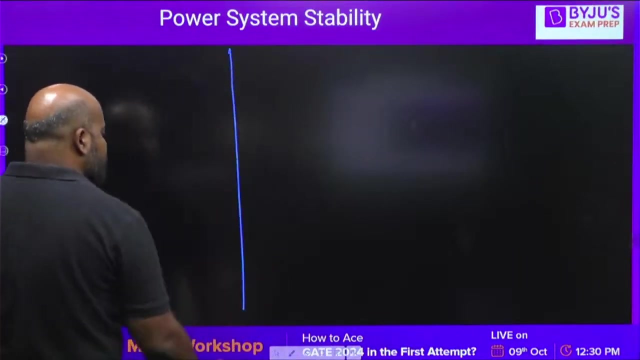 What is the reason? Can you tell me what is the reason Why synchronizing power coefficient has to be as high as possible For having more and more stability in terms of steady state stability? let us try to understand. This is del angle. 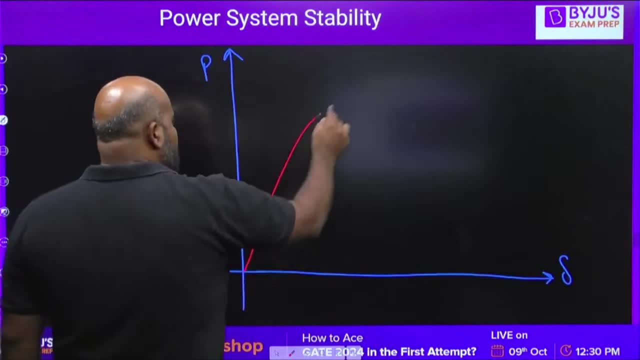 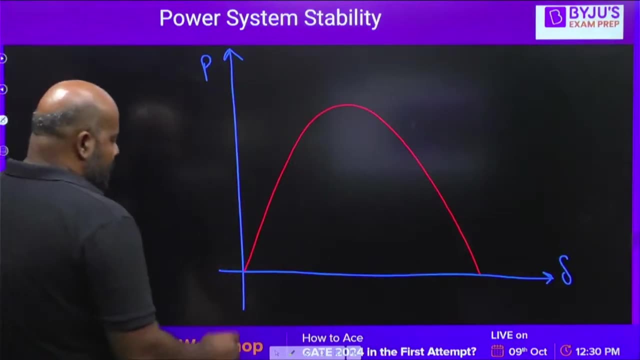 This is real power, Something like this. Now suppose I am giving you a condition. Suppose this is P max- Okay, P max, Okay, Pm. That is the earlier operating point And this is del naught, Yes or no? 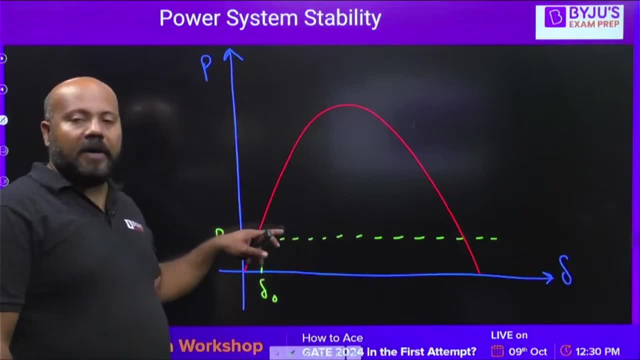 This is the del naught initial operating point And you are delivering Pm magnitude of real power. Now, because of some small disturbance, suppose. now because of some small disturbance, suppose you want to reach to a new position, Okay, 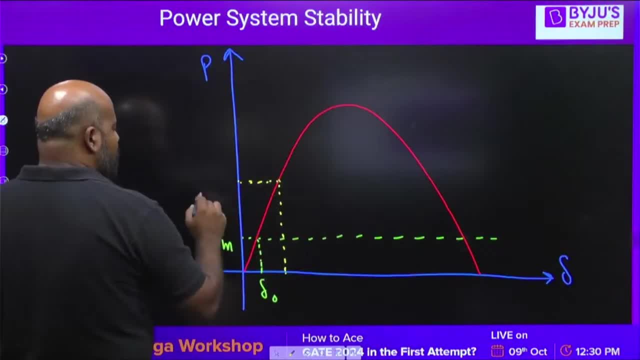 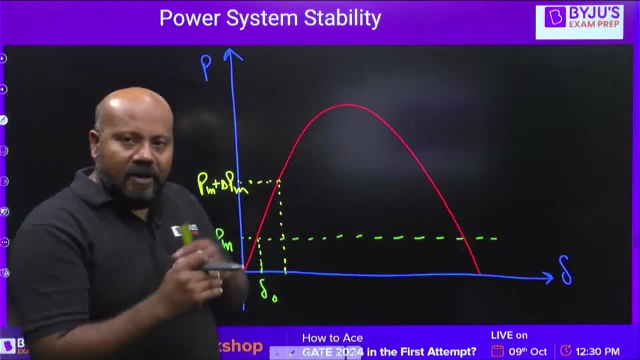 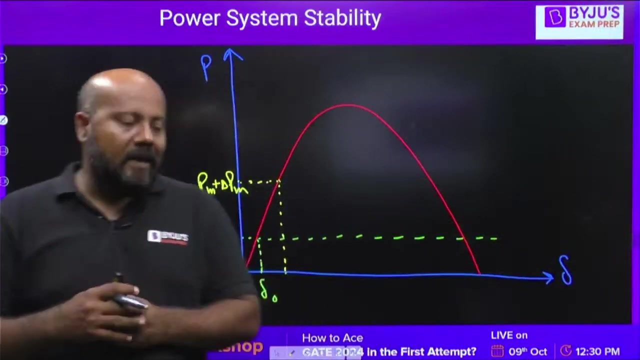 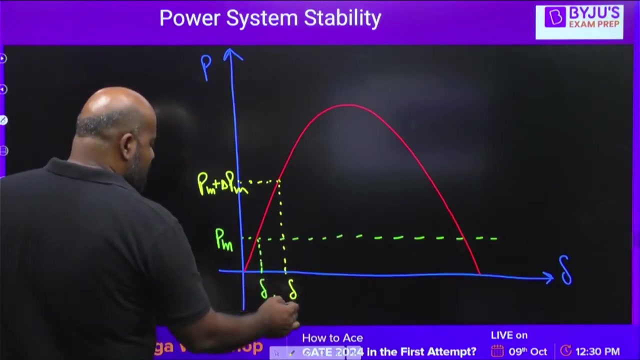 to a new position and you want to deliver more power. suppose this is pm plus delta pm. okay, some extra real power you want to transfer. for that purpose, you have to increase this pm to pm plus delta pm. now suppose this is the initial operating point del naught and this is the new. 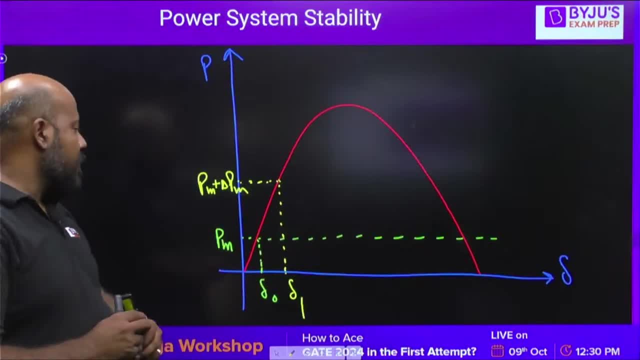 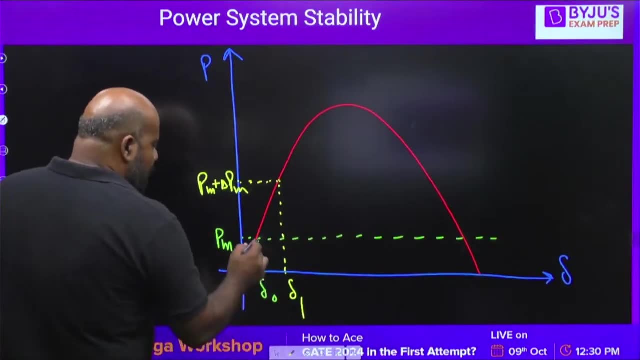 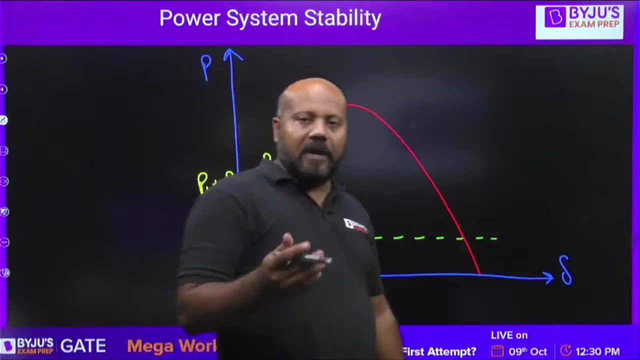 operating point del 1. this is the new operating point del 1. now please try to understand. basically i have to go from point a to point b, yes or no? what is the agenda if you want to increase the power from pm to pm plus delta pm, basically you. 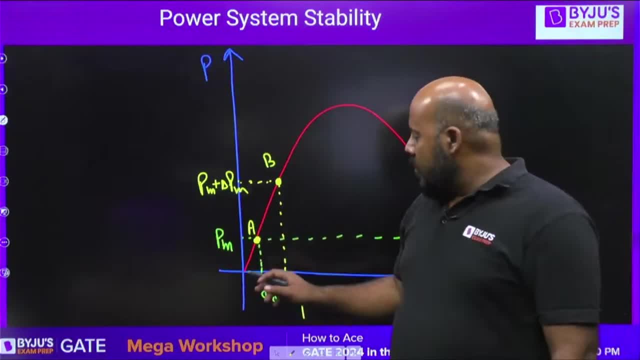 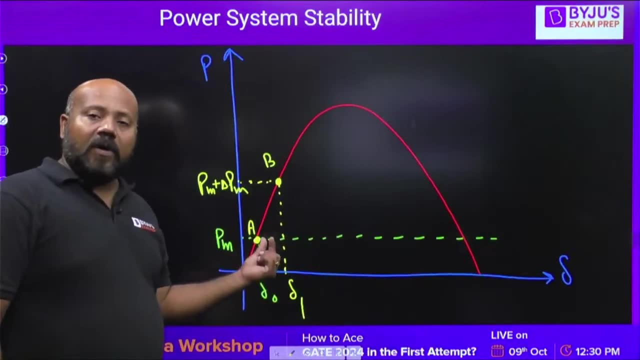 have to go from point a to point b, initial operating point, to the new operating point. now, the more and more less time is involved in this transition, the more stable is going to be your system. or you can say, less and less change in del is going to be involved. 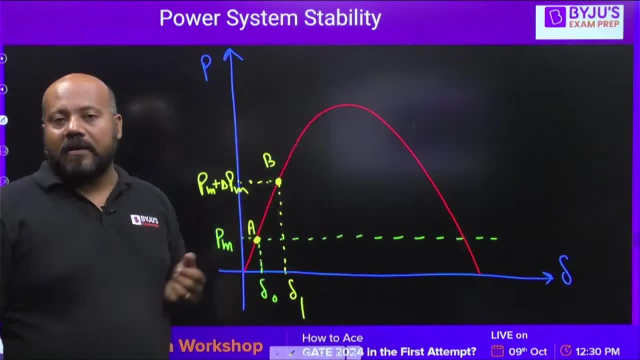 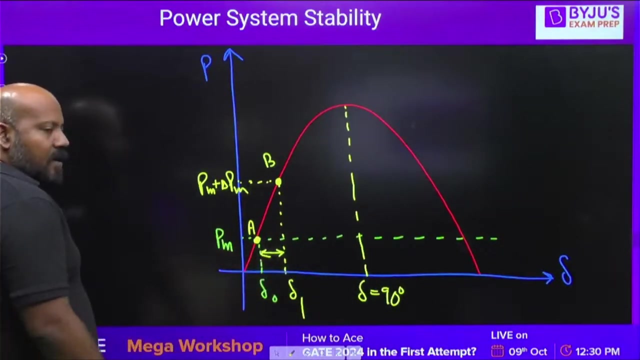 in this change, more stable is going to be your system, yes or no? when this distance is going to be less? because if you keep on increasing the del value, you will reach near to the unstable region that is. del is equal to 90, so we want this change in del has to be as minimum as possible. it is only possible if this graph 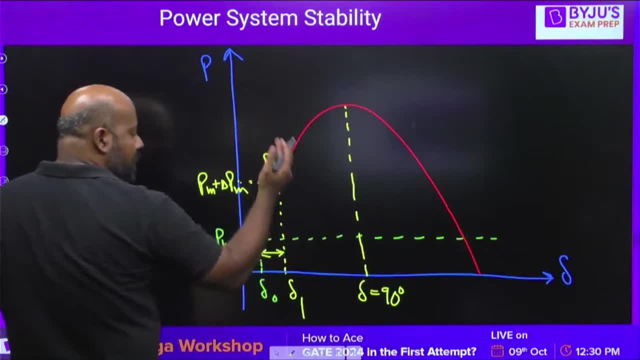 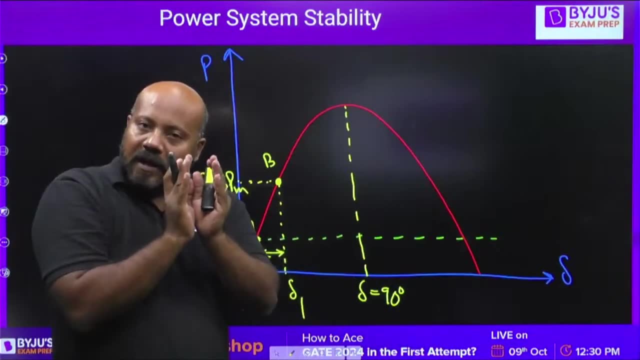 instead of like this, it is going to be like this: more and more slope, higher and higher slope means what? the change in y-axis is going to be more and the change in the x-axis is going to be less. are you getting this? you keep on increasing the slope. you keep on increasing. 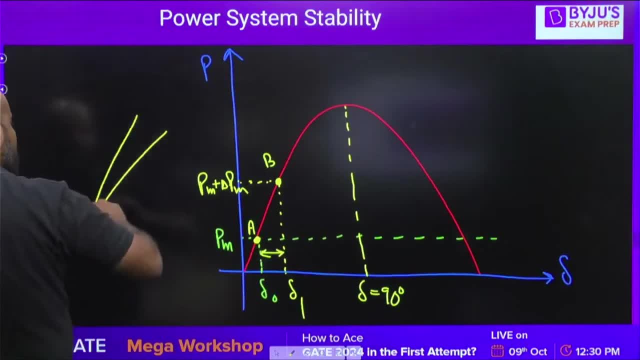 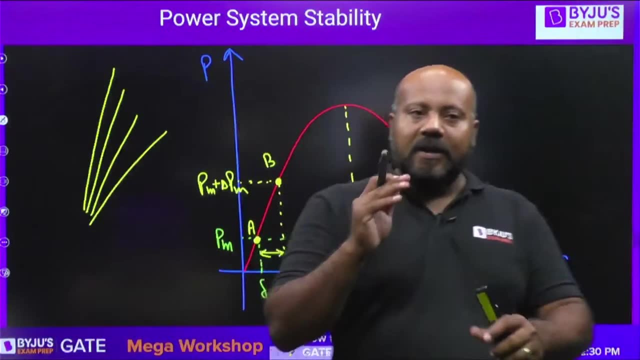 the slope. suppose the slope is like this. now you are saying, no, it is like this. no, it is like this, no, it is like this. are you getting this? so for a given change in the power, the change in del is going to be less for a higher slope and that is the reason for high and high, stable region. for 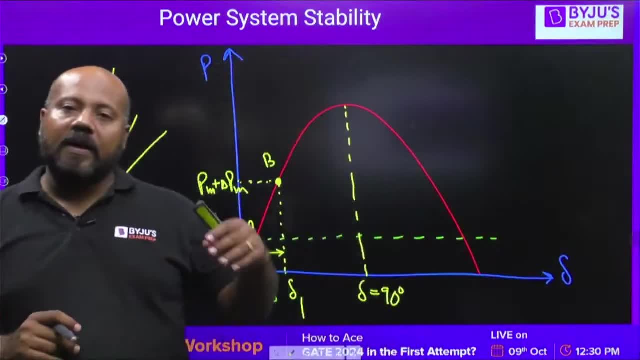 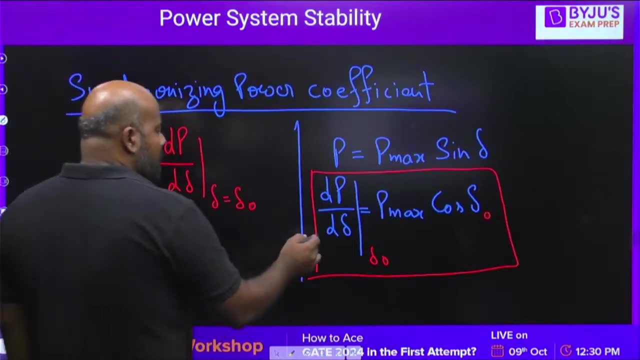 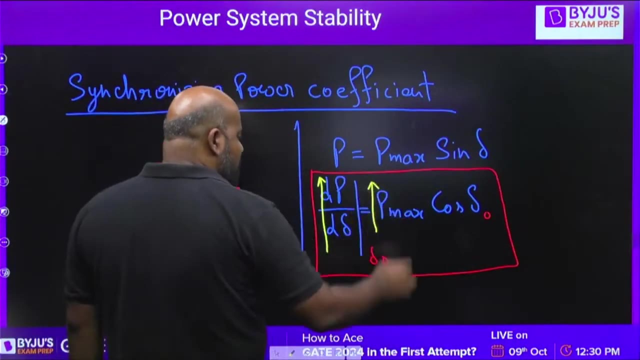 more and more stable region, we have higher and higher value of synchronizing power coefficient. now, if you want a higher value for your synchronizing power coefficient, it means there are two possibility: either p max has to be more than 0 and sin power is equal to 0.2, because 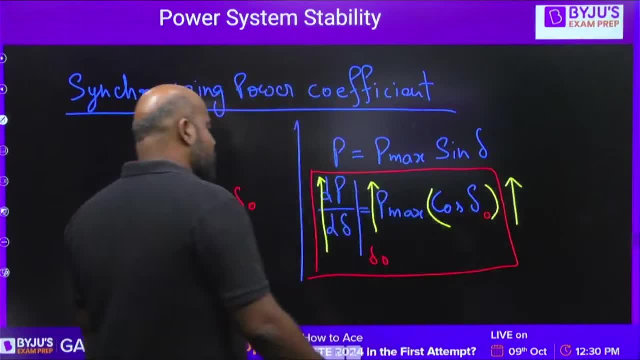 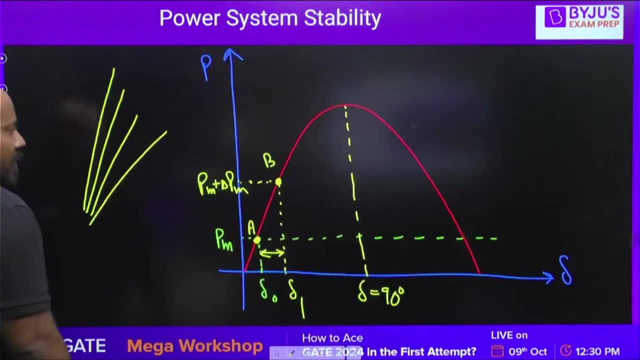 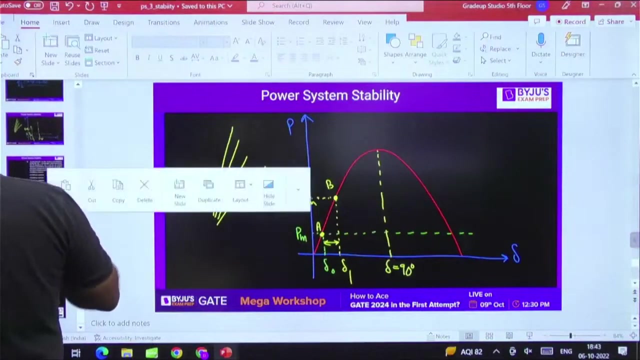 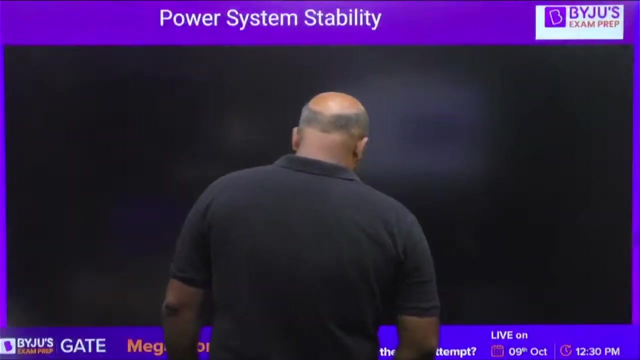 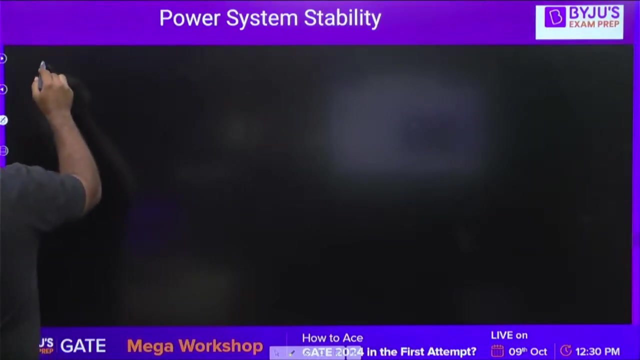 or cos del naught has to be more. Let us take the two conditions. Let me add some page here. Suppose you take the first condition. The first condition says that P max has to be maximum or highly stable system. What is P max? P max is mod V 1, mod V 2 upon x In more. 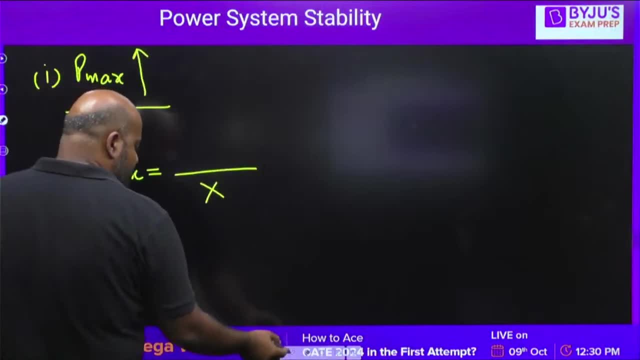 simple words You can write. it is simply mod V square. So if you want to increase P max, what are the possibilities? Possibilities is: either you increase the operating voltage or you reduce x. So one way is: voltage is increased. Now you have to reduce x. How you are going to? 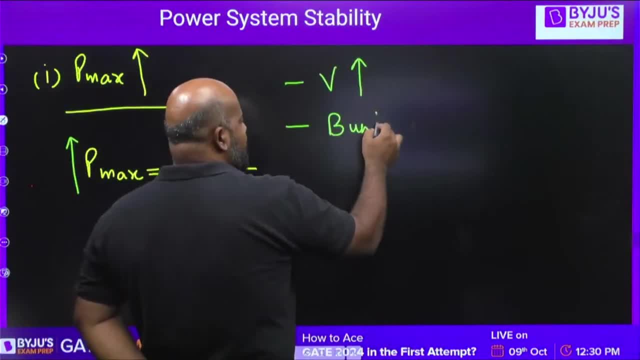 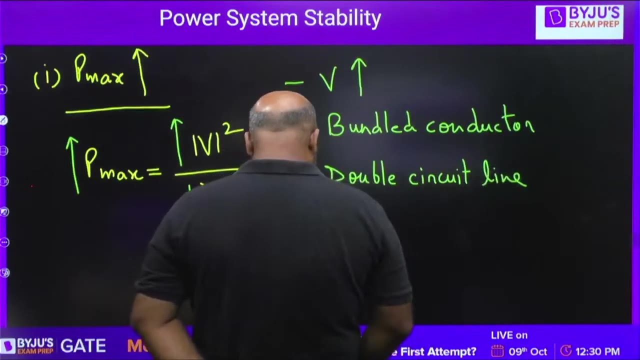 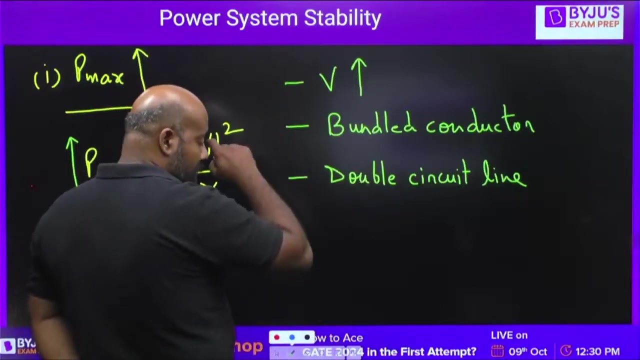 reduce x. You can use bundled conductor- Bundled conductor- Okay, Bundled conductor system. or you can use double circuit line. You remember, Yes or no? Bundled conductor and double circuit line. what is happening? Bundled conductor and double circuit. 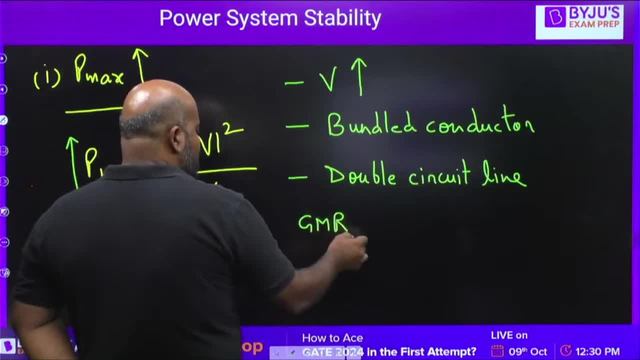 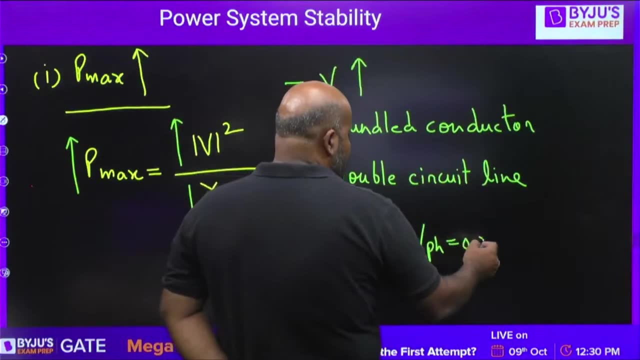 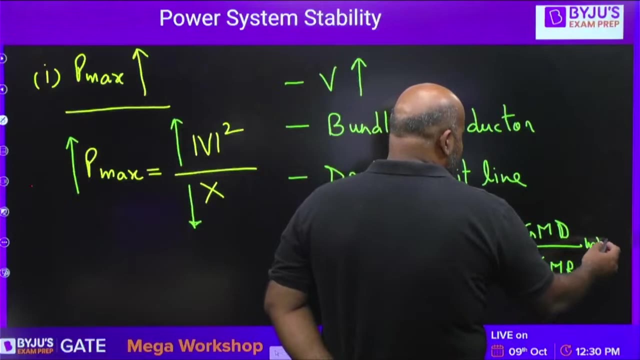 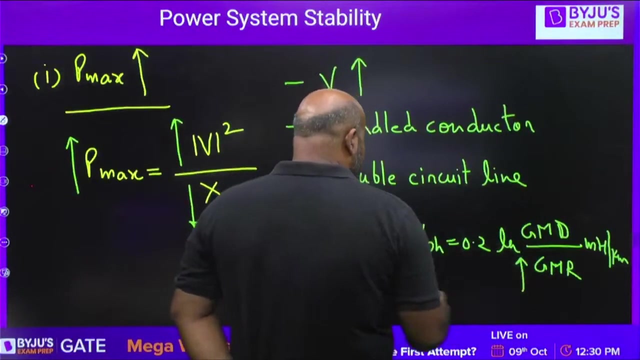 line. basically GMR is increased. When GMR is increased, what about inductance per phase? It is 0.2 ln. Okay, Gmd upon GMR, This is milli Henry per kilometer. So if you are saying, sir, GMR is increased. 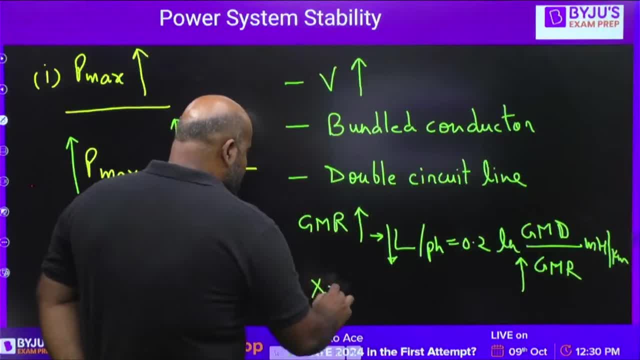 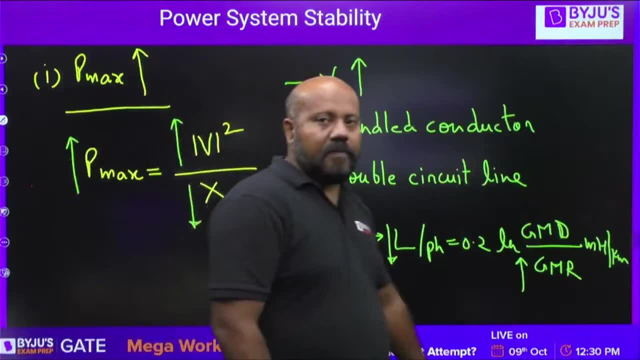 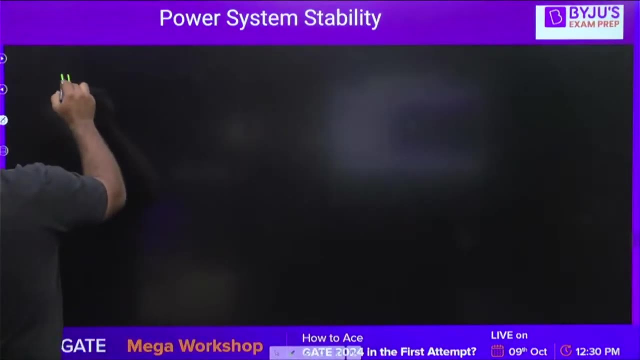 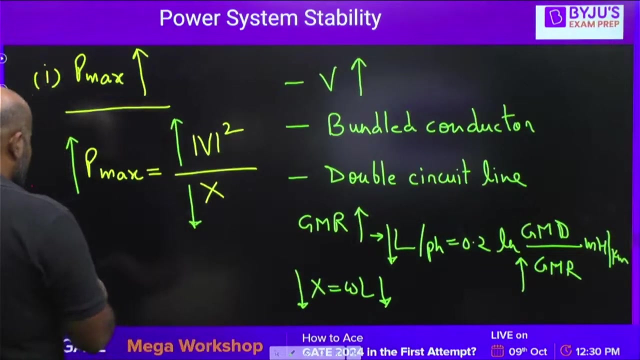 it means inductance per phase is reducing. It means x, that is omega L. If L is reducing, x is also reducing. Is it clear, everybody? This is the first case. Now the second case says That there is one more way of reducing x. How you can reduce x: You can use series. 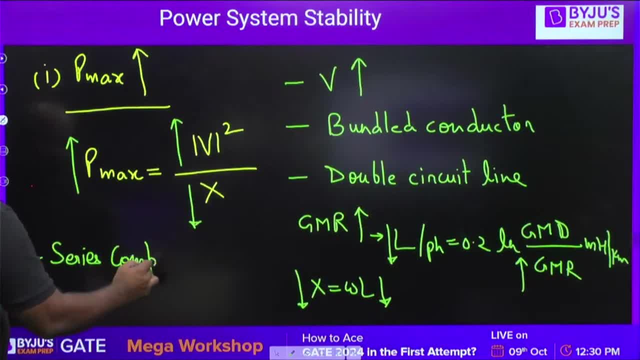 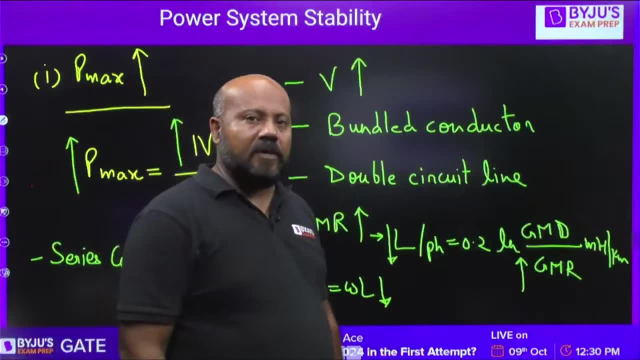 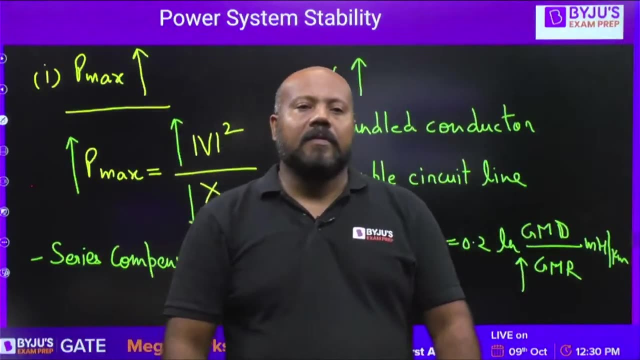 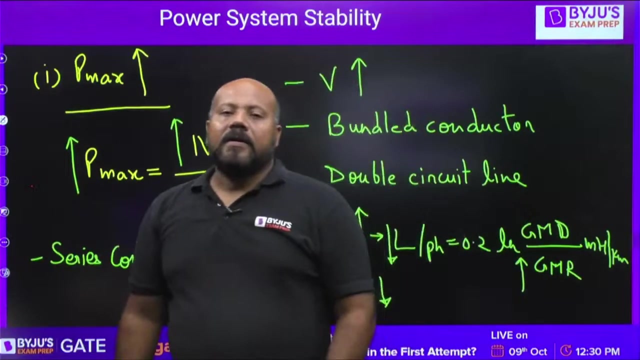 compensation. You can use series compensation, Yes or no, By compensating the series reactance, by using series capacitor compensation. Okay, Okay, What is the next step? Synchronizing torque is the same as the previous step. Now, if you are knowing, you can use. 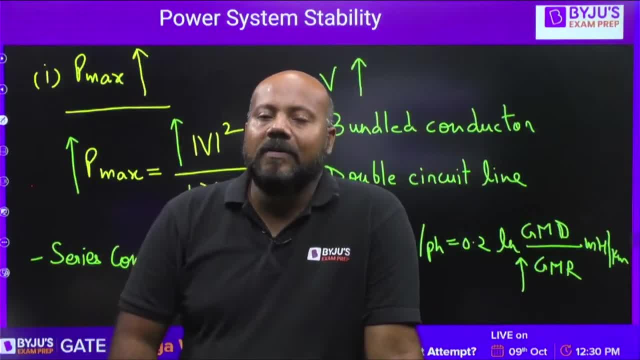 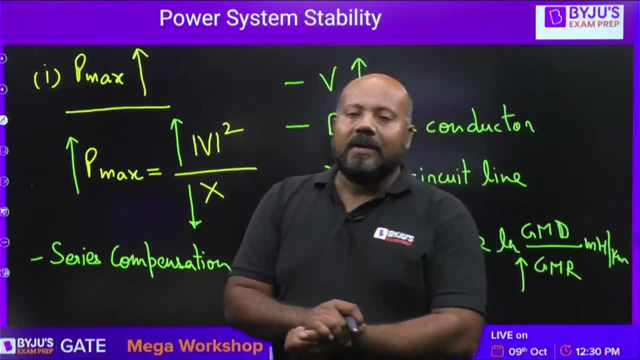 this method. The first step is the synchronizing torque. Now, the synchronizing torque is different concept. You can understand it that whenever there is a change, whenever there is a change, the synchronizing torque will come into the picture to get the machine again in synchronism. 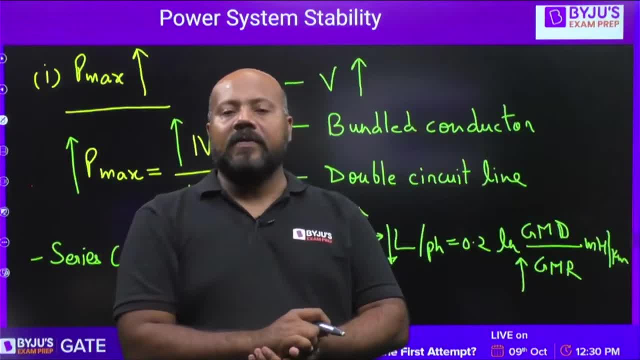 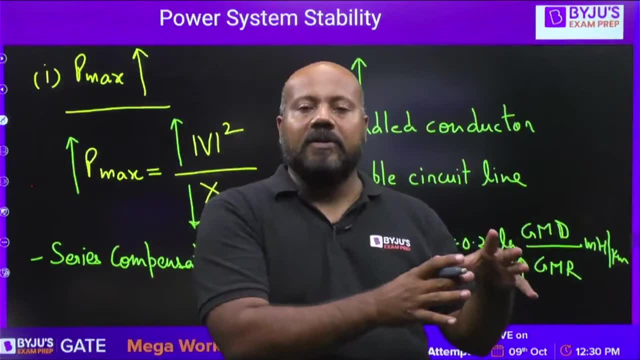 Okay, That is defined by using this synchronizing power coefficient also Okay, But this synchronizing machines, okay, in the machines, electrical machines. we will be discussing that. let us keep ourselves up to only synchronizing power coefficient in the power system when we are discussing. 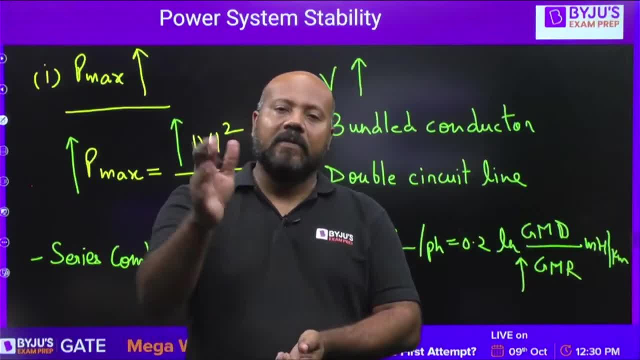 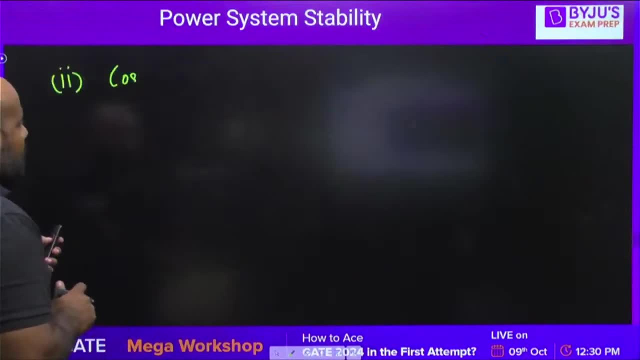 electrical machines, synchronous alternators. one day when we will be discussing then we can discuss that okay. the second point, that is, cos del naught having a higher value is going to be when del naught is going to have a lesser value, so you have a less operating value of the del. 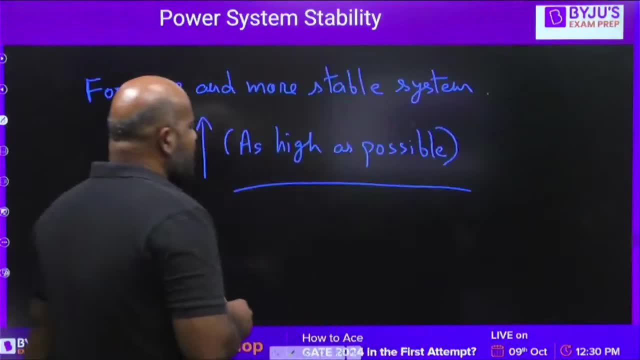 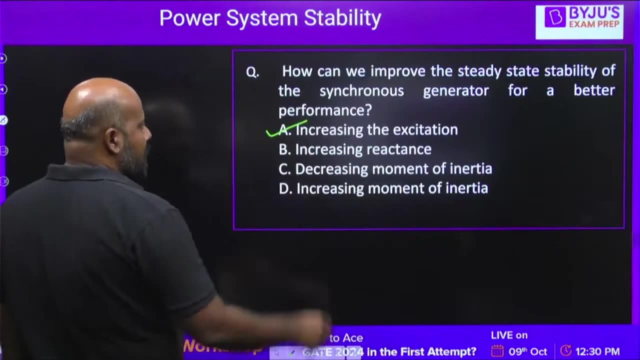 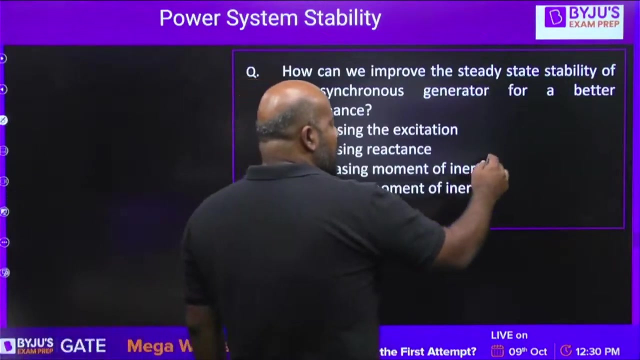 you have more stable system. so let us cross check what are the given options. increasing the excitation: it is right because you are increasing the voltage. increasing the reactance wrong. decreasing moment of inertia: increasing moment of inertia is wrong because movement of inertia deals with transient stability, not with the steady state stability. 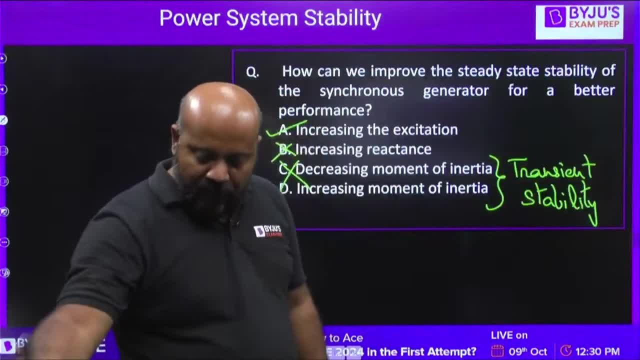 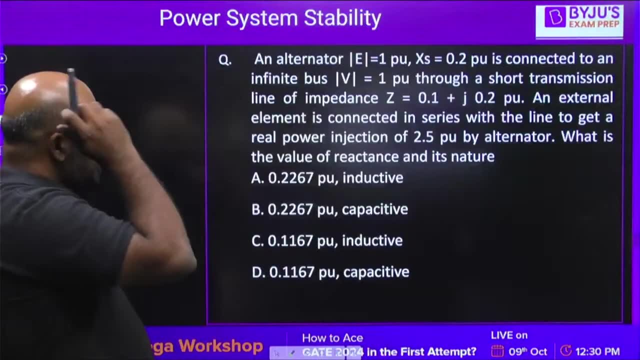 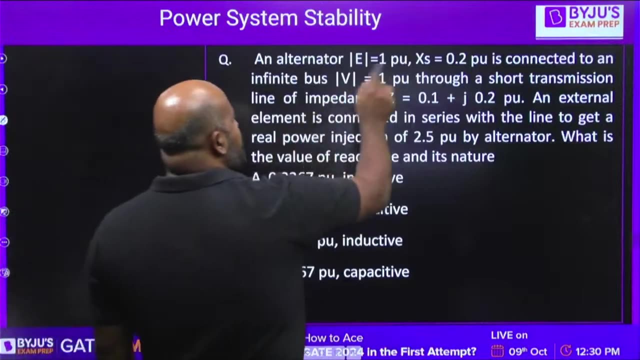 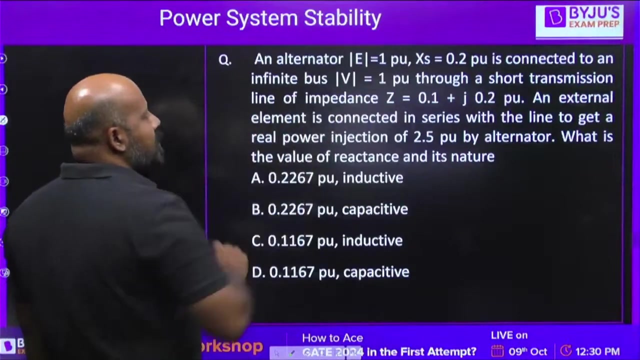 is it clear everybody? so a is going to be the correct option. let us talk about this question now. this is a very interesting question. an alternator having the excitation emf magnitude as 1, the synchronous reactance 0.2, is connected to an infinite bus where the infinite bus voltage 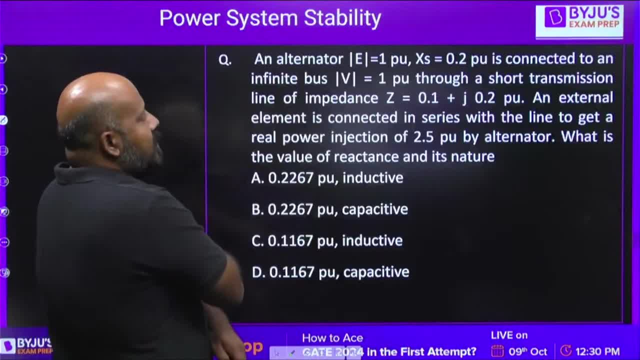 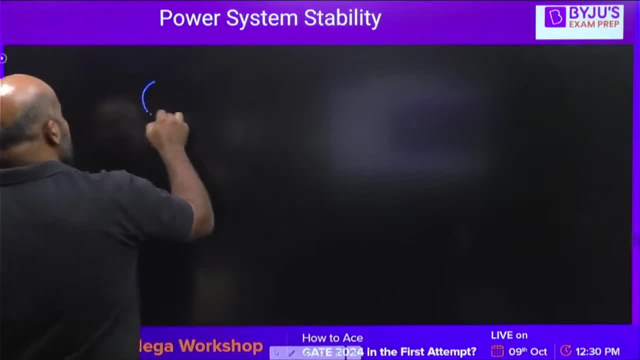 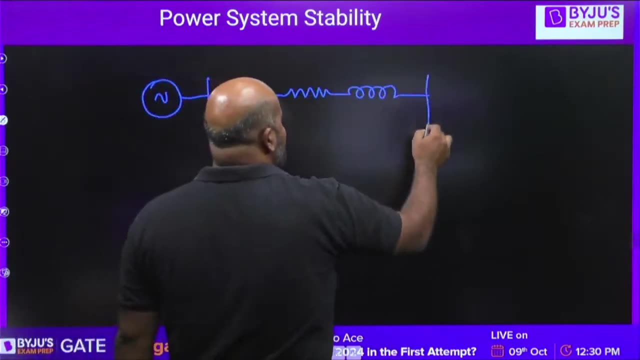 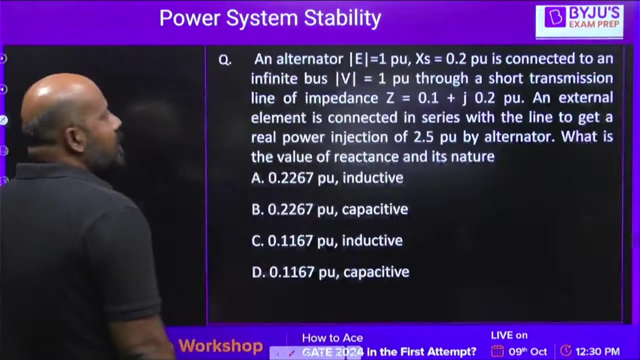 is mentioned as 1 per unit, through a short transmission line of impedance z 0.1 plus j's 0.2. so the situation is something like this: this is the alternator. okay now, this is a short transmission line and it is connected to the infinite bus, so e magnitude is given as 1 per unit. 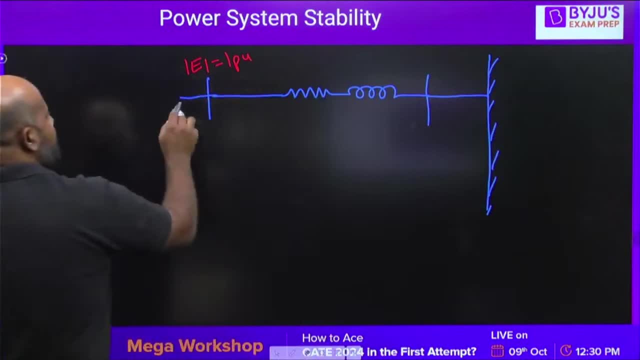 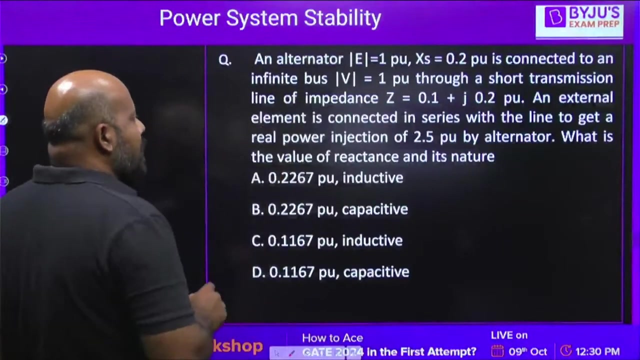 okay, so we have to draw. this is. wait a minute. suppose this is the generator. this is the generator, reactance like this. so excitation emf is given as 1 per unit. it is given as xs is given as 0.2. okay, the short transmission line impedance is mentioned as z. 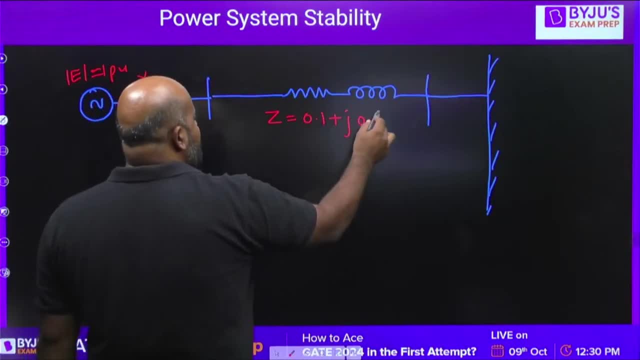 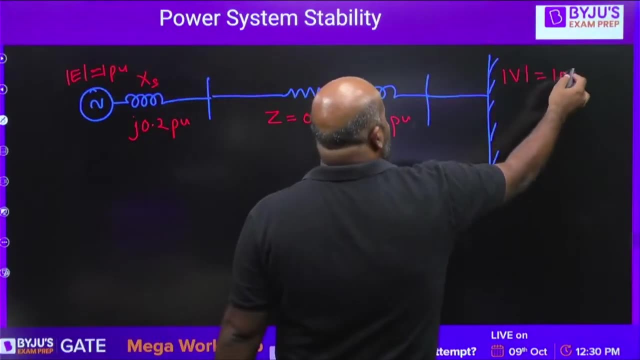 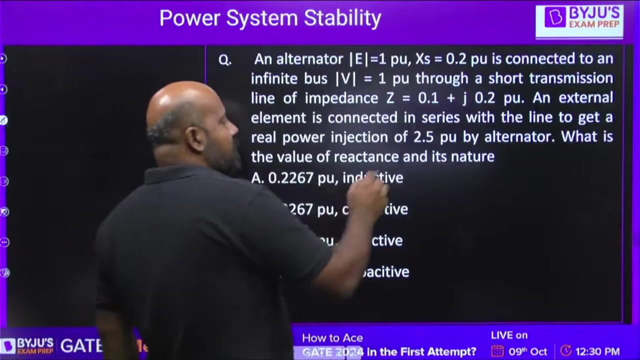 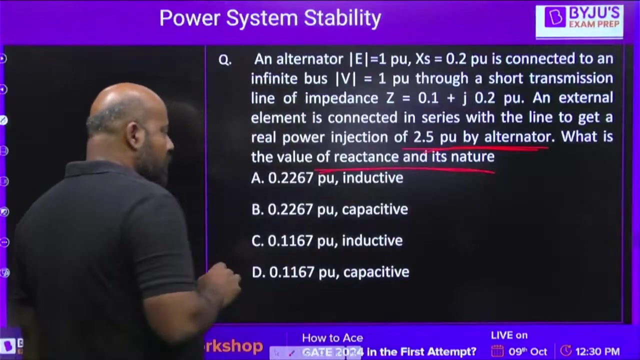 0.1 plus j, 0.2 per unit. infinite bus voltage is mentioned as 1 per unit. an external element is connected in series with line to get a real power injection of 2.5 per unit by the alternator. what is the value of reactance and its nature? what is the value of reactance and? 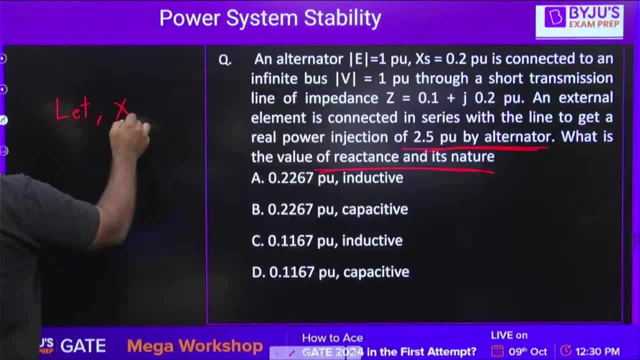 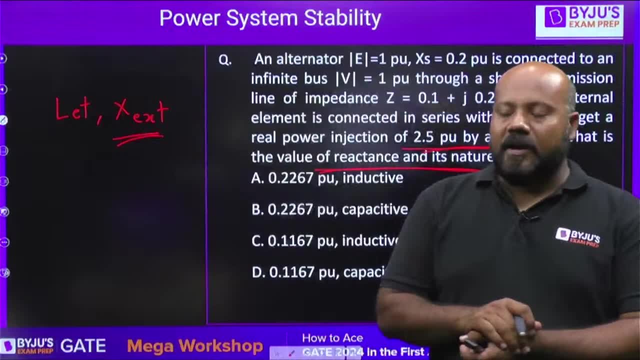 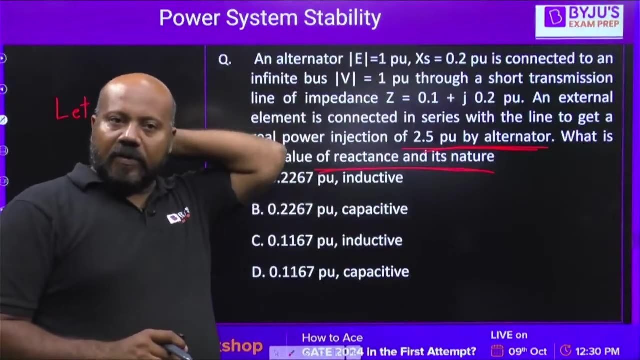 nature so let the external element added is having the reactance x external, yes or no? it is x external. now in this question, if you go in the direct way, okay, conventionally. if you go, it will be little difficult for you to reach to the final solution easily. 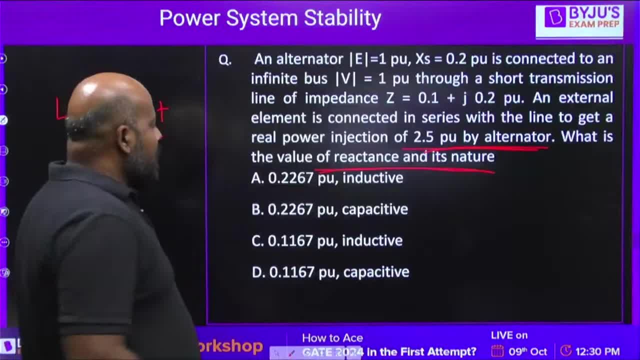 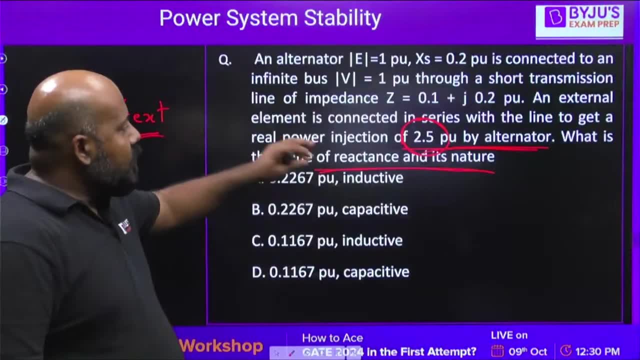 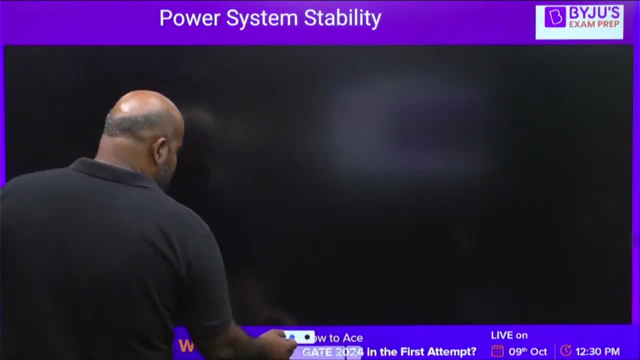 what you can do. you can work a little smarter. let us try to find what is this condition of power being transferred by the alternator. it is mentioned as 2.5, So let us understand if we talk about the real power received or maximum value of the. 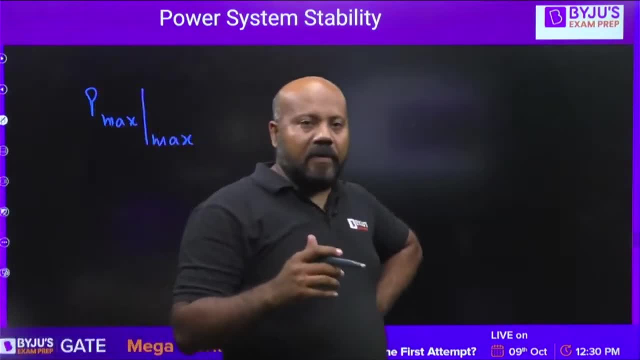 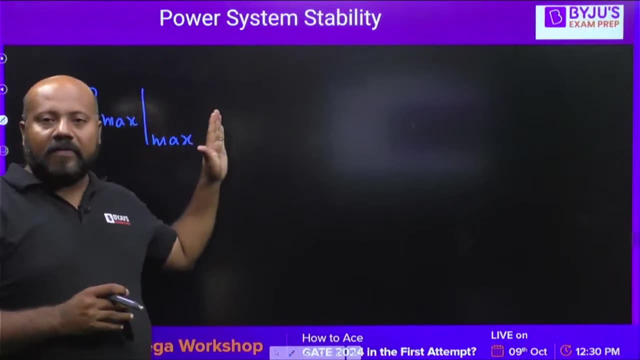 real power received: maximum value. excuse me, I am saying the maximum value of the maximum real power received at the receiving end. This is given as mod V square upon 4 R. infinite bus voltage is mentioned as 1 per unit. so 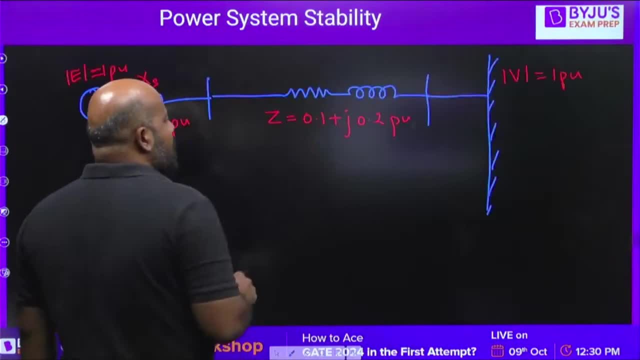 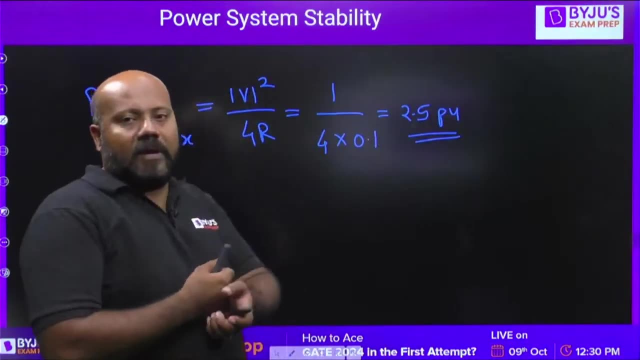 this is 1,, this is 4,. what is the resistance value? it is 0.1,. if you solve this, you will get 2.5 per unit. It means the real power transferred condition is the same condition that we find when there. 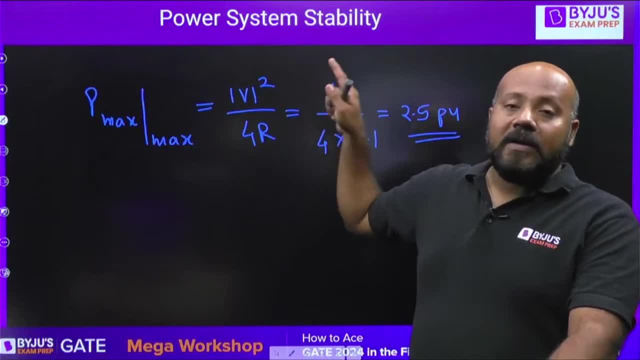 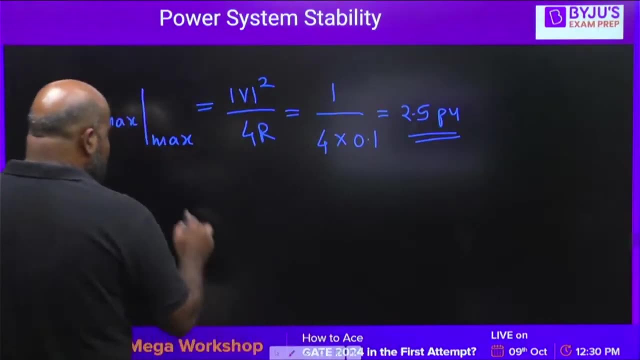 is the maximum value of the maximum real power transferred to the load. In this condition, at the design level, the X by R ratio is going to be equal to load 3, this is the condition. this is the condition for this X by R at the design level. the. 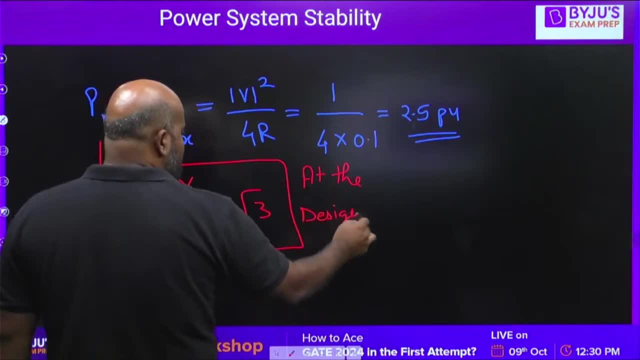 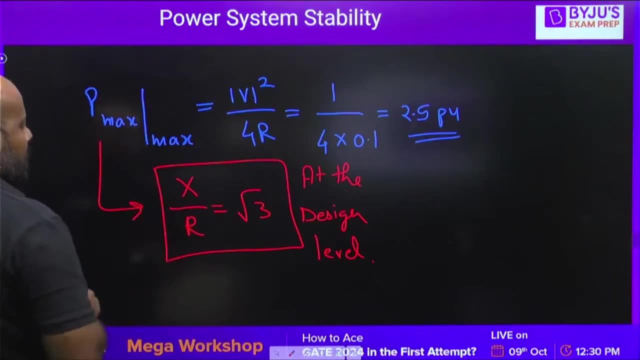 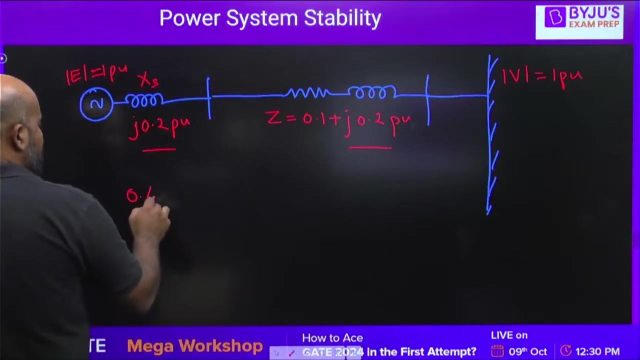 design level. at the design level, are you getting that? So put the total X value, put the R value and equate it to the under root 3.. What is total X value? It is 0.2, it is 0.2, so it is going to be 0.4 plus X external divided by 0.1, and this: 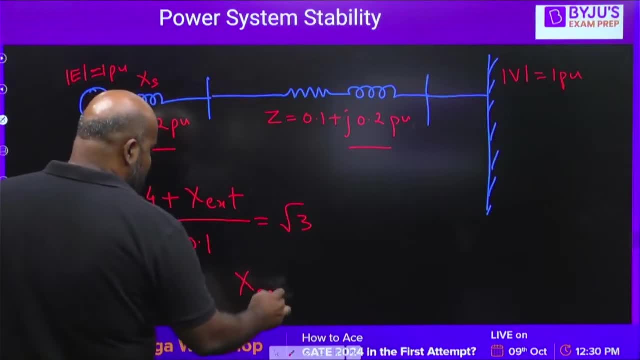 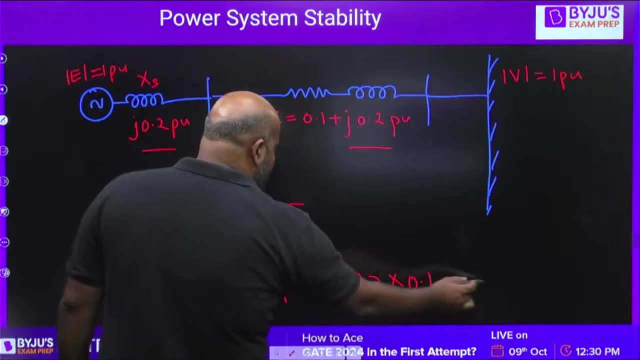 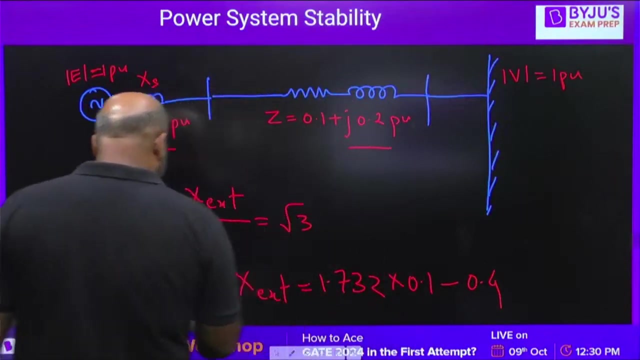 is under root 3.. So you can write it X external as 1.75.. Okay, 0.32 multiplied by 0.1 minus it is 0.4.. If you solve this- okay, if you solve this- then you will get minus 0.2267.. 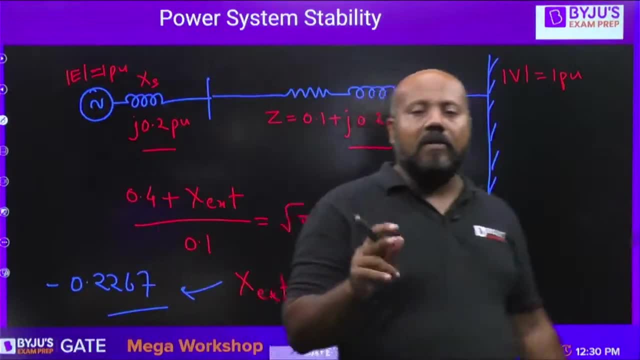 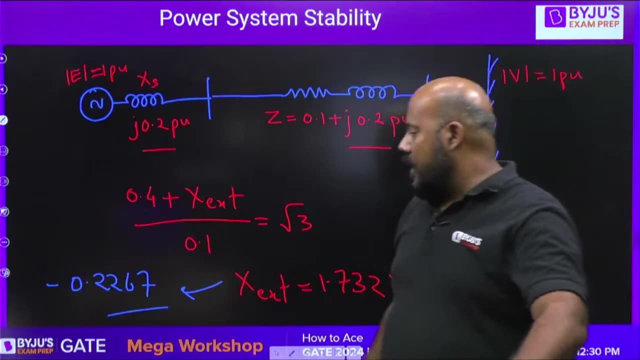 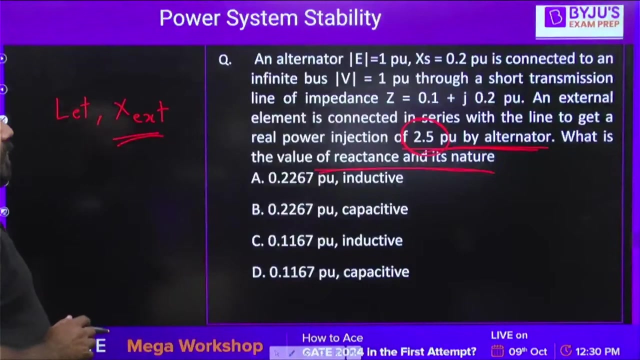 What is the meaning of this minus? This minus simply means that, instead of adding a reactance, actually you are adding a capacitance. Okay, So it is capacitive in nature. The element is capacitive in nature. That is why you are getting a negative value for this, but the magnitude will remain same. 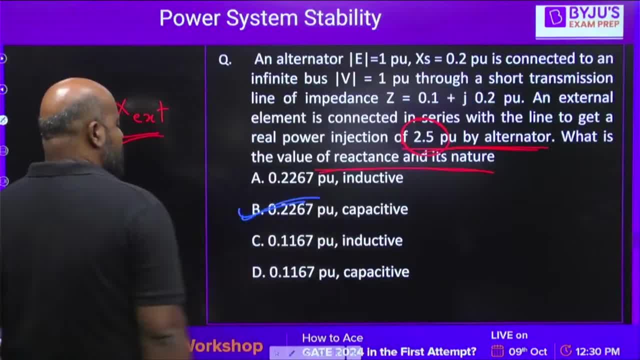 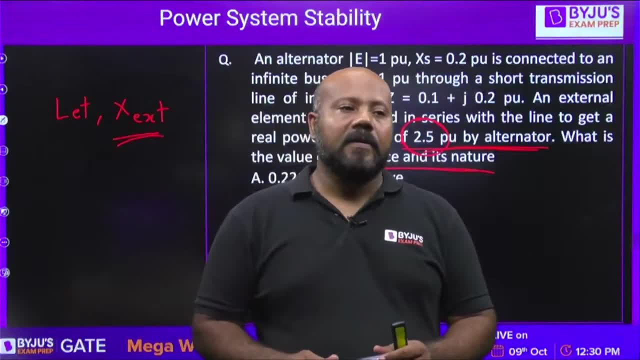 So it is 0.2267, but capacitive in nature. That is the B option. Is it clear for everybody? Are you able to follow this? Yes, everyone. So this is all from my side for a steady state stability. 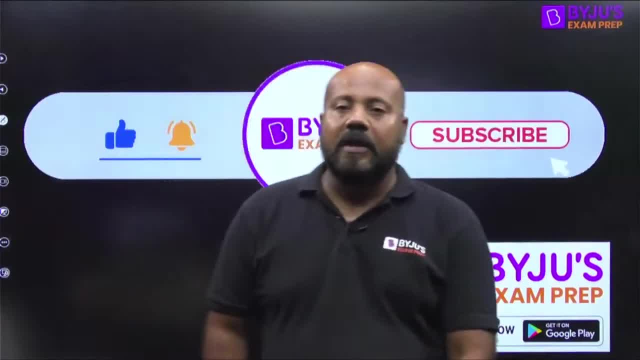 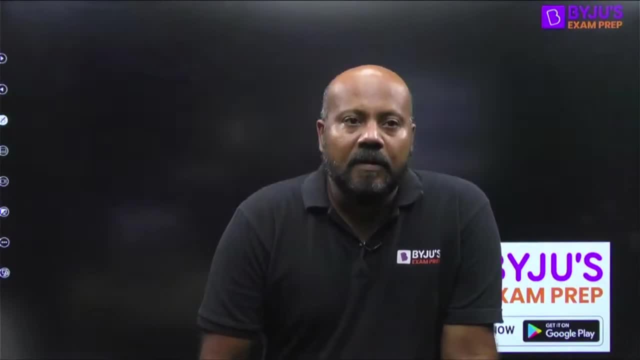 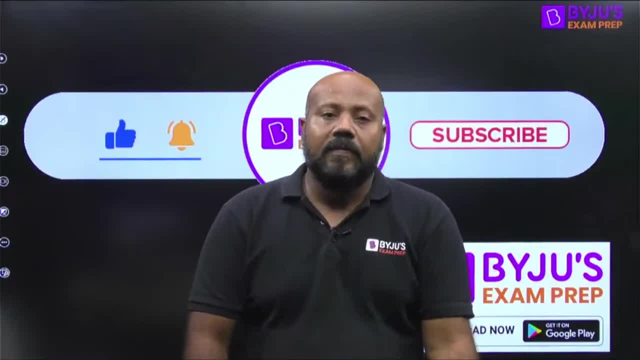 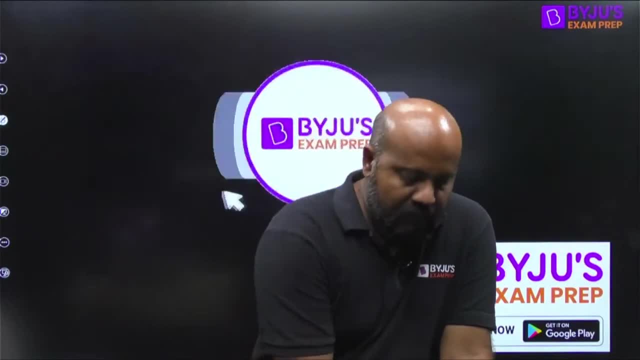 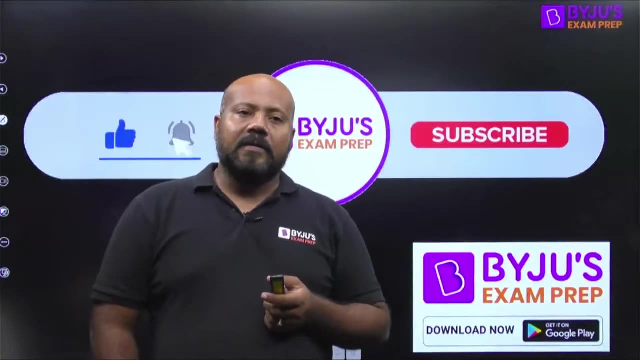 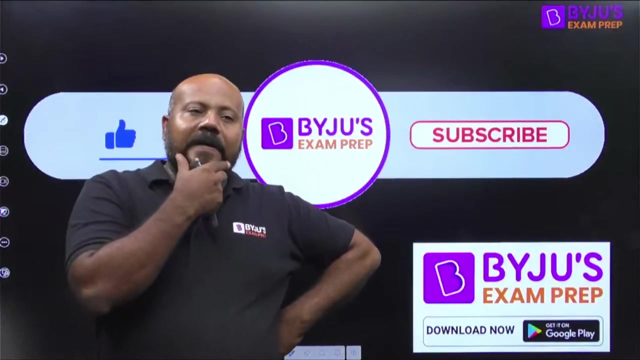